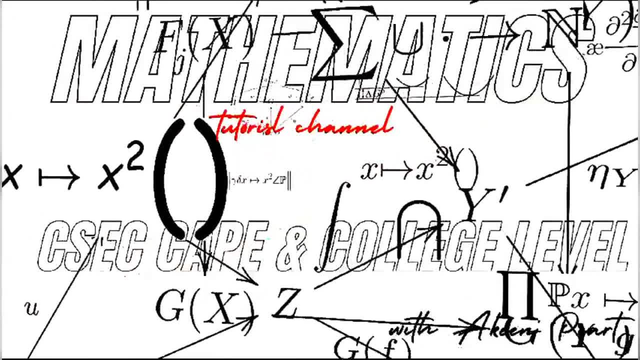 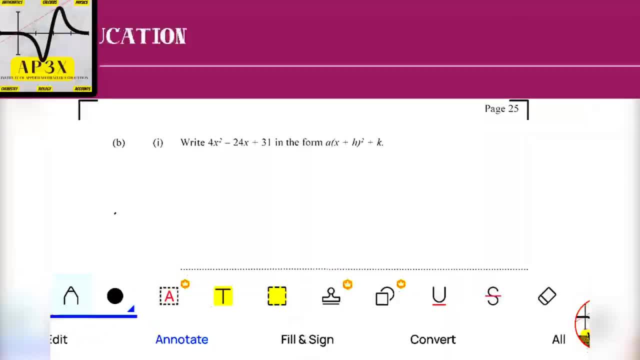 Hello everyone, welcome and welcome back again to another video tutorial from the AP3x Institute of Mathematics Education. My name is Akeen, your math instructor, and in today's video we are going 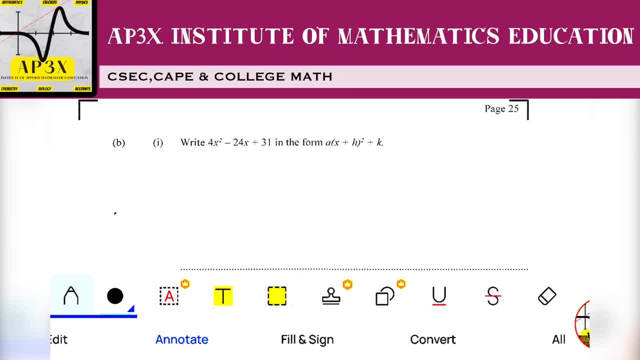 to be wrapping up the 2024 January recent examination paper that was just recently concluded in 2024. That is in fact January the 4th or I think it was January the 5th. Now of course you 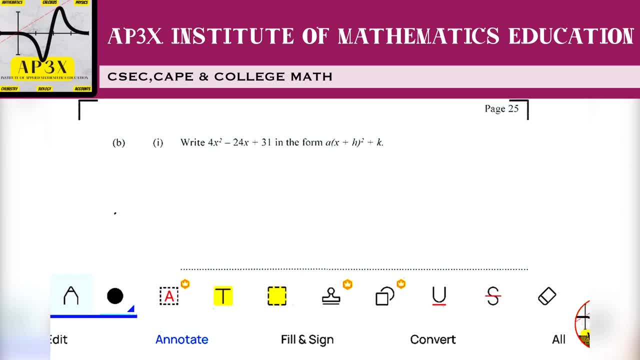 would have already seen three of our uploads. Upload one was where we discussed questions one to three. Upload two we discussed questions four to seven. And of course upload three we discussed 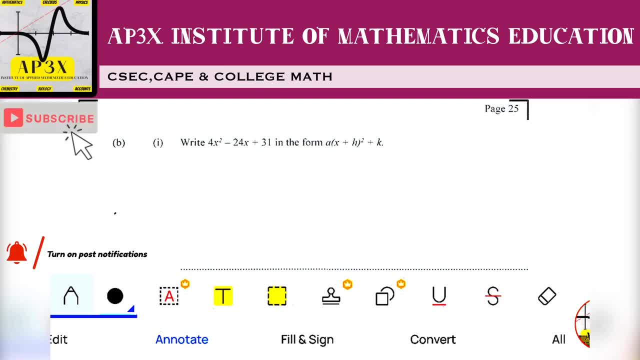 questions eight all the way to question nine. And of course that was quite of an intense video lots of stuff was discussed in that so I do recommend that if you are in fact watching this 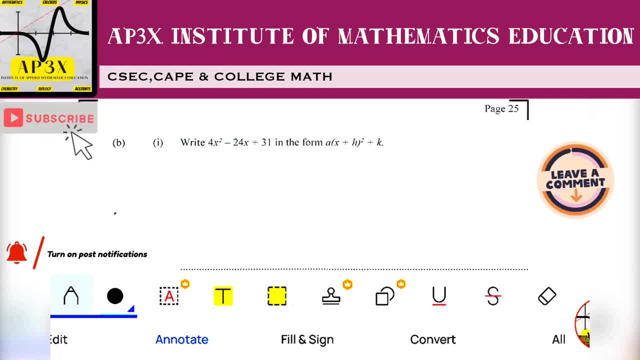 video for the first time then it would be highly recommended that you go ahead and check out part one part two and part three. Now I've decided to do the video like this because of course 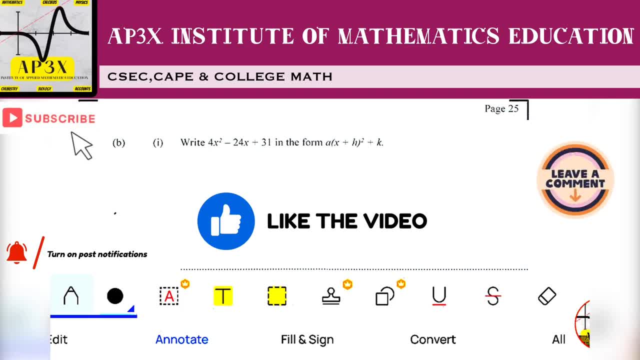 I don't just want to provide you with the solutions but I also want to develop your analytical thinking so I take my time and I go through all the little things that you need to 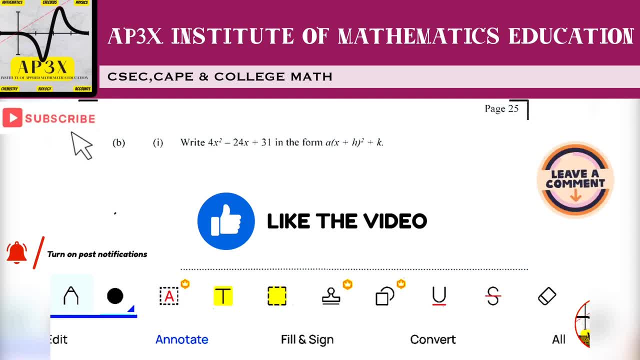 know in order to be able to answer questions of similar nature. All right so definitely highly recommended that you go ahead and check out those other three parts for 2024. I'll definitely be doing a series of videos for you as it relates to past papers. So I'll be doing a compilation 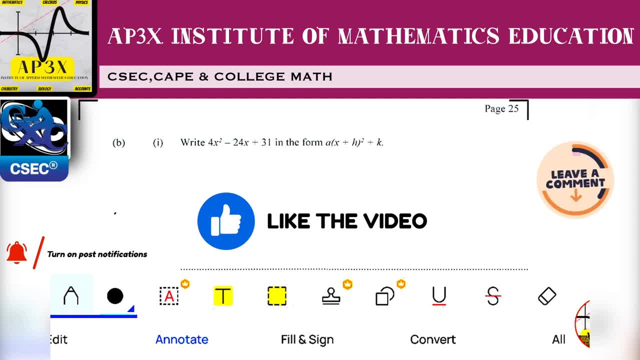 of questions one, question twos, question threes from different different years January and May to give you as much resources as you possibly can get to be prepared for the exam coming up. 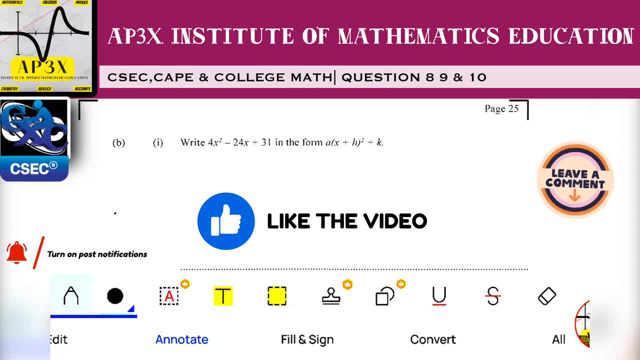 All right now of course if this is the first time you're on the channel then I would love for you to subscribe to the channel feel free to subscribe to the channel and grow the family of mathematicians future mathematicians of course do not forget to leave your positive questions and comments down 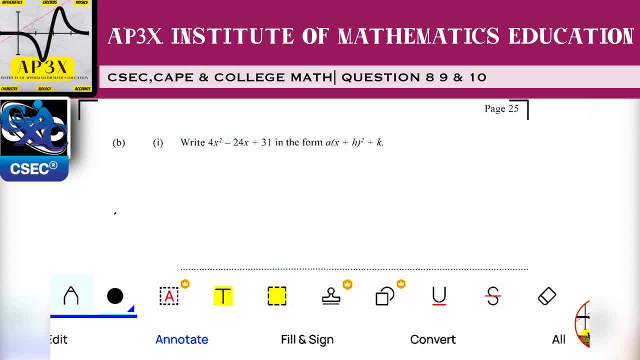 below your suggestions how I can make it easier for YouTube uh in for your math preparations of course leave a like if you have gotten some sort of value from the contents being posted here and of course do not forget to hit the like button it really really does help the channel to grow 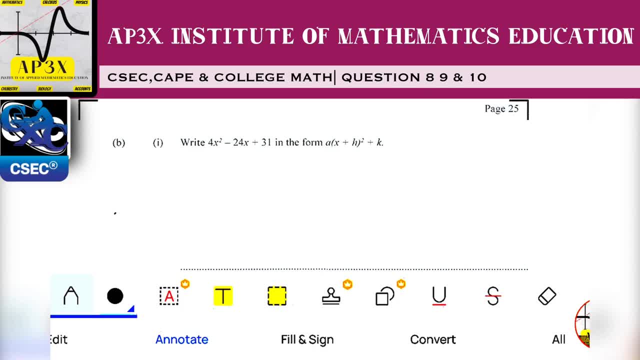 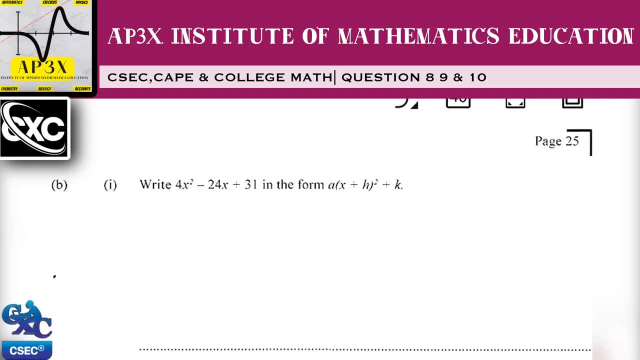 so uh let's just jump right into it and begin this final upload of the 2024 January recent people now what I've decided to do here guys for this particular uh paper here for this particular 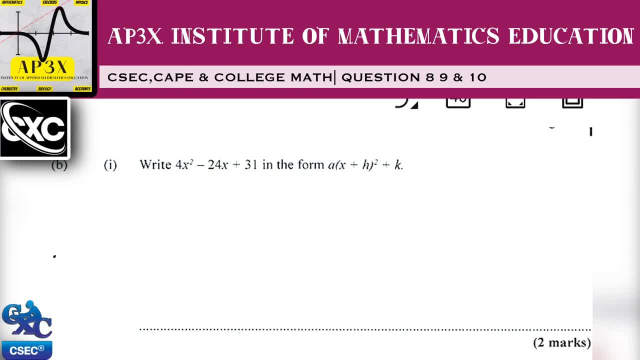 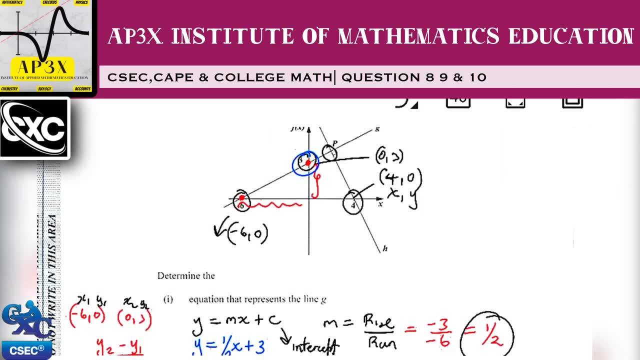 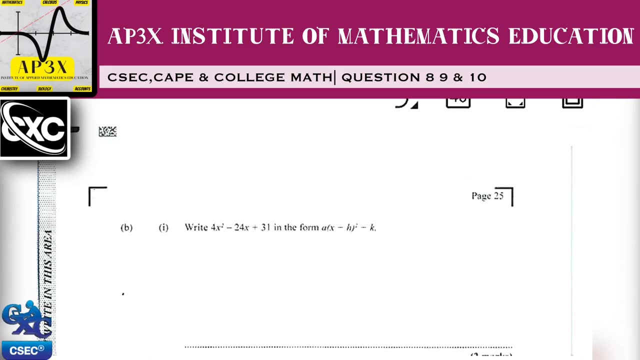 upload I've decided to go back through question C here let me scroll up I think we were doing uh this is in fact question eight so I've decided to go back through the graphical part of question eight and in the editing process of that video I kind of felt like I didn't really give you guys a good clear explanation and how to approach the completing the square problem so I'm going 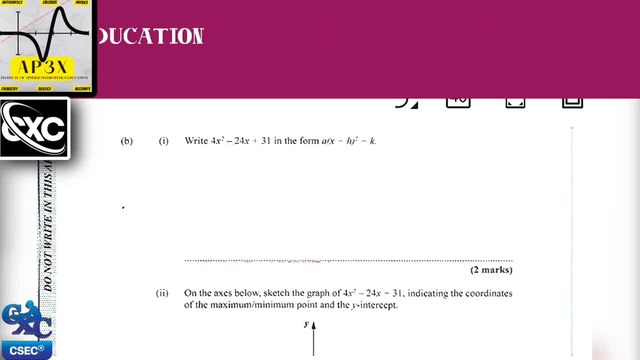 to be taking it from here and I'm going to be wrapping up the whole entire paper for you 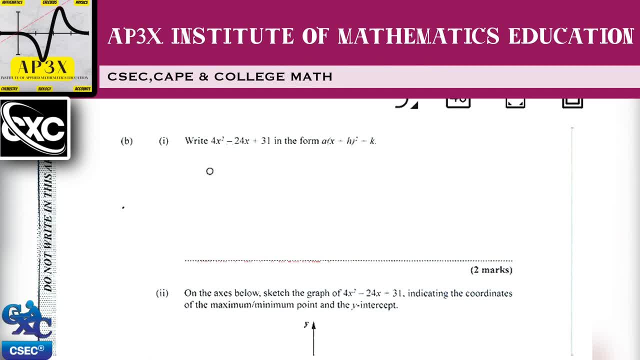 in hopefully less than an hour uh of this video all right so we're going to be starting the explanation from this question here all right now the very first thing here that we're looking at is in fact we are required to write 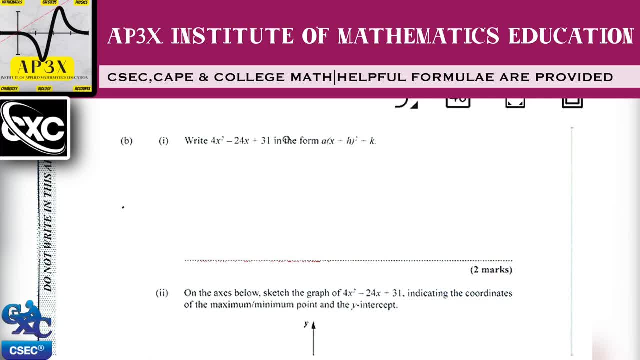 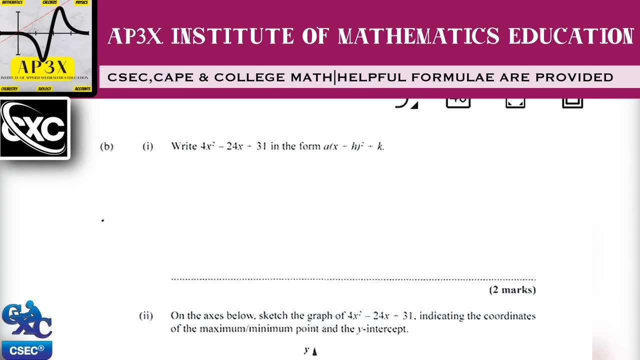 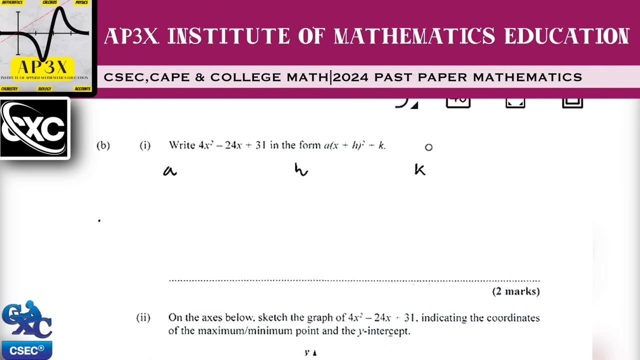 4x squared minus 24x plus 31 in the form a open bracket X plus H R squared plus K now of in completing the square there are three particular values that we need to we need to place our focus on and those values are in fact finding the value of a finding the value of H and finding the value of K now what I'm teaching you here is a shortcut method in terms of completing the square near there is a technique for doing this but in this shorter version of completing the square I believe CXC only requires you to state the values here so to find A is not particularly a value that you have to calculate A is more of a value that you have to just basically observe so when you're given a quadratic equation such as 4x squared minus 24 x plus 31 then your value of a is in fact the number that appears before the x squared so in this case here right away that a is in fact four now there 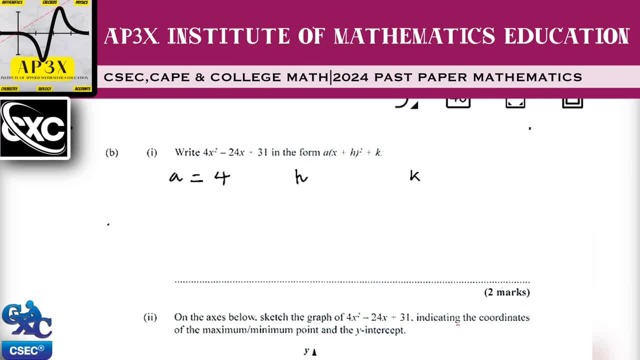 is a formula that was derived by completing the square for the quadratic format by completing the 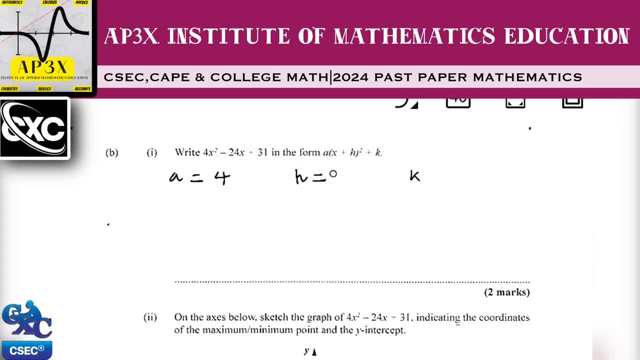 square we basically will see here that the value of h is in fact b divided by 2a now i do not have a tutorial on this of how to derive these formulas because that is more like for advanced students for csec the requirement for deriving the formula i've not yet seen that as a question on the exam paper so we just pretty much it's a case where you just grab the formula and go now to find h here it's going to be required that the value of b is in fact the number that appears before x so that is in fact negative 20 so four all right and then we're going to divide that then by say here two times the value of a which in this case is also four so when we work this out we find that h then is equal to negative 24 divided by 8 2 4 is 8 so h works out to be minus 3 and if you want some more clarity on how i'm getting my a values my b values and of course you're going to see over here my c value then you can visit the link that is pinned in the comments that will take you to two particular videos the introduction the quadratic expression and also you could watch the video on how to solve quadratic equations so that is how i'm getting my values of a b and c now here you're 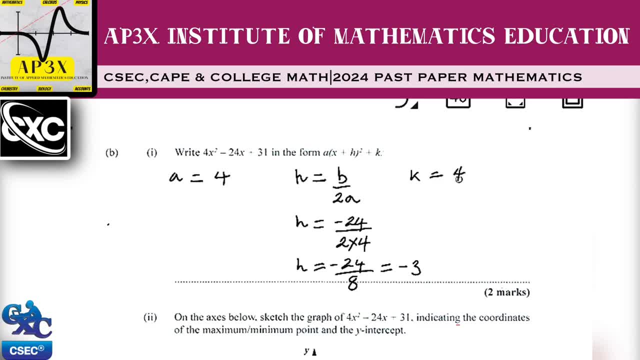 seeing here that the formula for finding the k value here is in fact 4 a c minus b squared all divided by 4 times a so therefore then uh what we're looking at then is in fact k then works out to be 4 multiplied by the value of a which is in fact 4 again multiplied by the value of c which is the constant 31 and then therefore now we're going to be subtracting the value of b squared from that that's going to be negative 24 squared and that's all b divided then by c here 4 times a which is 4 times 4 now once we go on our calculator here and we type in 4 multiplied by 4 multiplied by 31 we would end up with a result here of 496 and when we go ahead then and we square negative 24 we're going to end up with 576 and that will all be divided by say here 16 4 times 4 16 now when you work this out minus minus sorry 496 minus 576 will result in negative 80 and that's going to be divided then by 16 so easily then we end up with a k value here which is equal to say here uh negative 5 so now we can just kind of highlight our answers a is in fact say here 4 b works so pardon me not b h here works out to be minus 3 and then of course 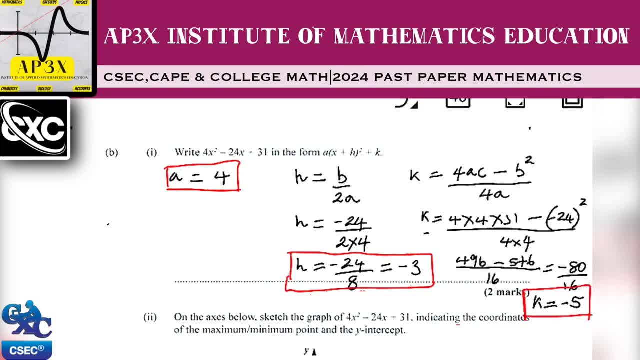 c k here works out to be negative 5. now with that we can therefore draw a conclusion by saying that the expression given 4x squared minus 24x plus 31 is in fact identical to and as they say here place the value of a which we know is 4 so that's 4 open bracket x will remain as x here but then the h value we had calculated is in fact minus 3x so that's 4x squared minus 24x plus 31 h equals minus 3. and so therefore then k then works out to be negative 5 so we have a negative 5 at the end and then this basically represents 4x squared minus 24x plus 31 written in the form a open bracket x plus h all squared plus k our answers then therefore 4 open bracket x minus 3 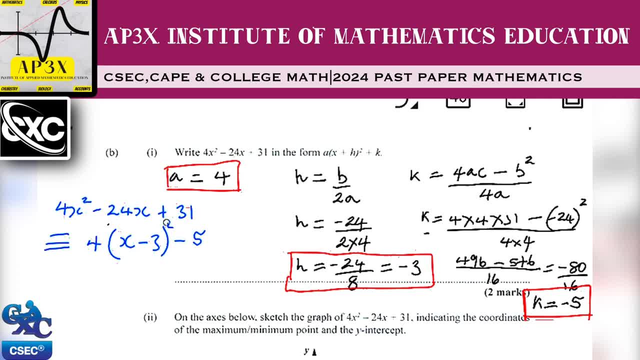 all squared pardon me i left off my square here minus 5. all right and that is how you complete the square using the short square and that is how you complete the square using the short 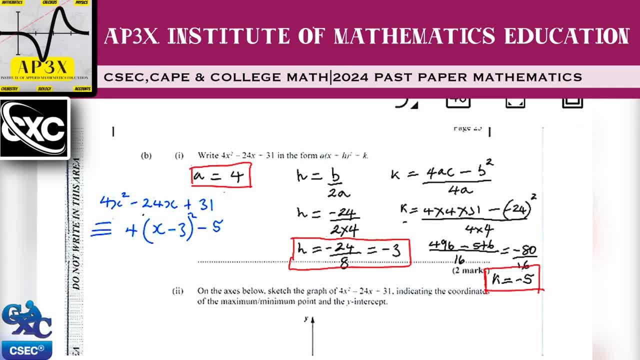 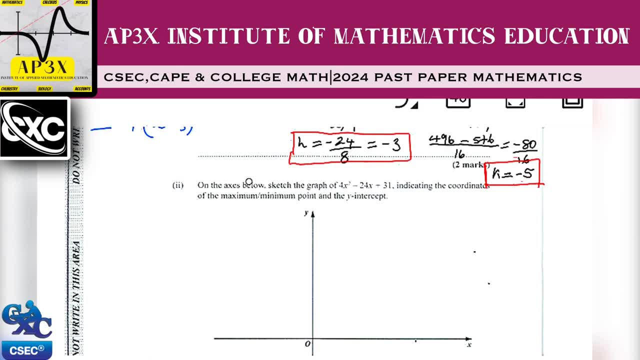 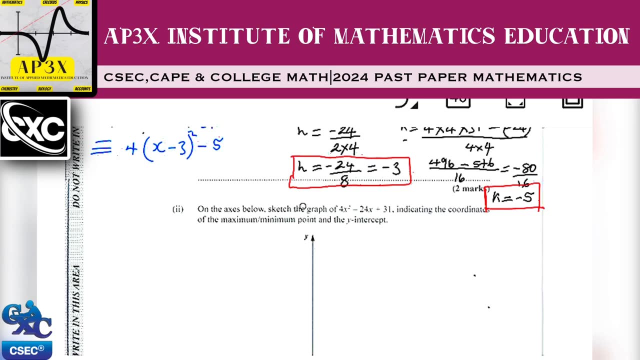 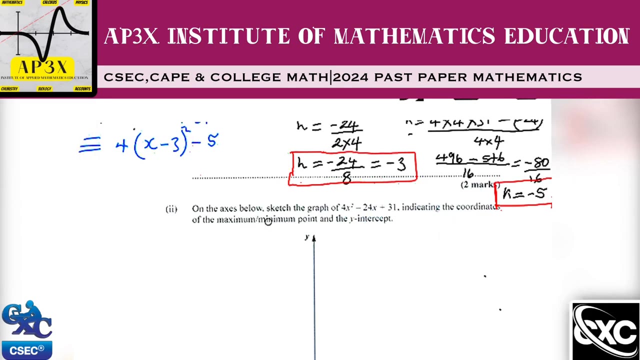 cut method then all right now beautiful let's go on here then to look at the part two to this question now it says on the axis provided which you can see here clearly they have provided you with an empty axis you're to sketch the graph of 4x squared minus 24x plus 31 indicating the coordinates of the maximum or minimum point and the y intercept now when it comes to sketching a graph what we need is just a kind of resemblance of what the graph would look like if we were given a table of values now when it comes to sketching the graph we're 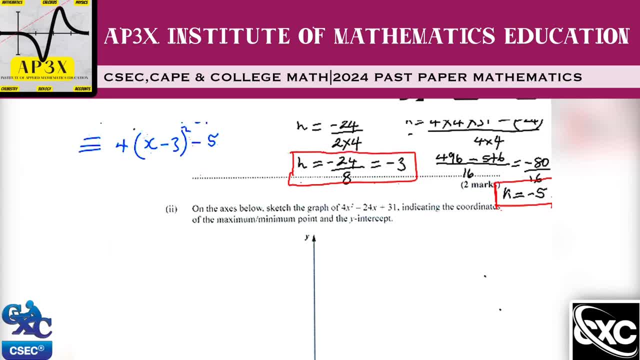 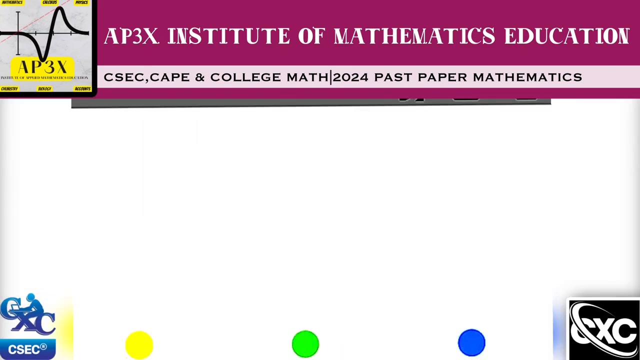 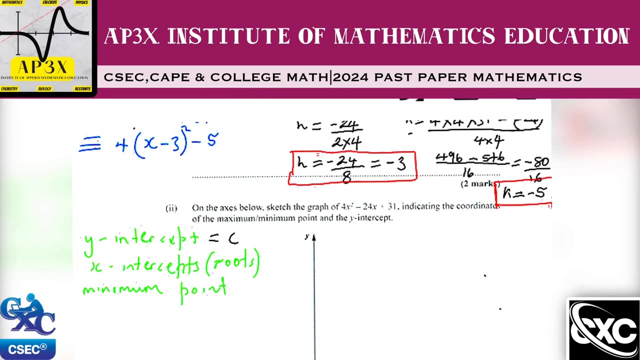 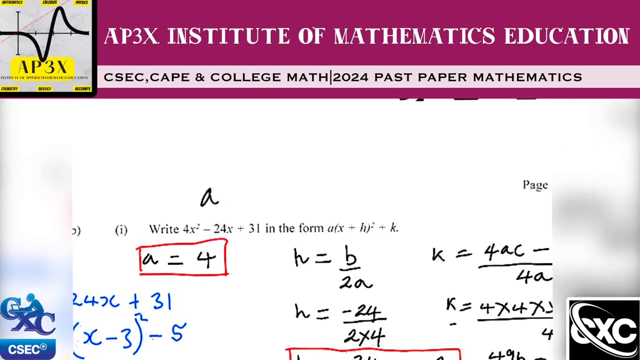 pretty much looking at in fact finding a couple terms here now let's just write them down here what are we going to need so number one i always tend to want to find my y intercept value first okay which is kind of like what they're asking you for so i want my y intercept value i'll let how you calculate that in a moment i'm also going to need what are known as the x intercepts this is more than one so my x intercepts or what you're going to find sometimes in certain questions they will refer to as the x intercepts as the roots of the quadratic equation and then you're going to look at finding what is known as your minimum point so your minimum point all right your minimum point and that's the lowest point or the maximum point in this case it's a minimum graph because it's a positive curve so i just wrote minimum point here but it could also be maximum point depending on the quadratic equation or the quadratic expression so now once we've done that then it's now time for me to tell you how do we actually predict or estimate these values now my y intercept here is what we most commonly refer to as the c value in the quadratic expression format now if you know anything about quadratic expressions you'll know that the general form of a quadratic equation or expression is in fact ax squared plus or minus bx plus or minus c so the constant at the end that number that is all by itself usually represents your y intercept 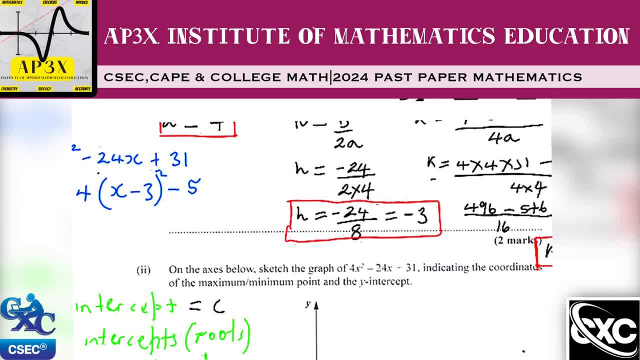 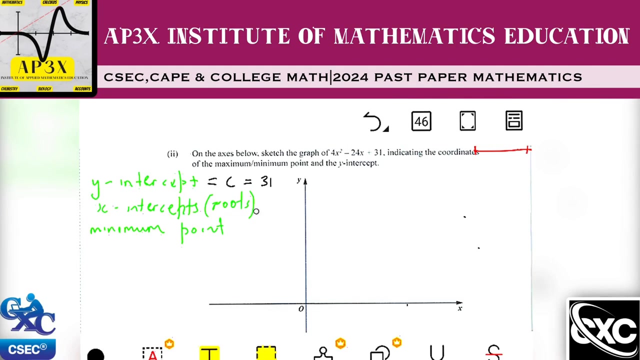 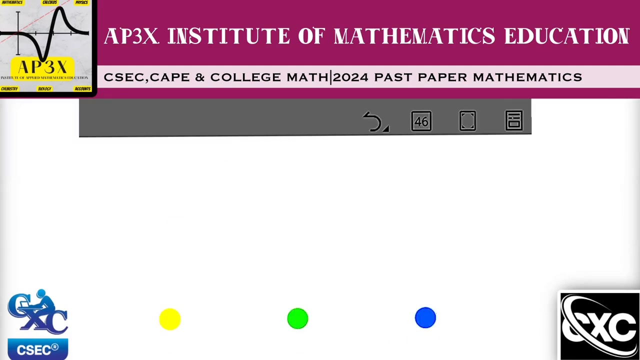 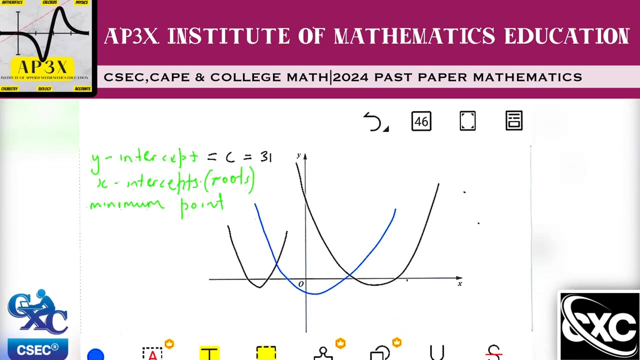 another way to actually calculate your y intercept is replace the x in the equation with zero so here we have this expression here you could replace the x with 0 and you could replace the y with 0 replace the x with 0 here work it out and you're going to find that your c value or your y intercept is 31 so we kind of just don't do that i kind of just let you know that the end number here this constant is always your y intercept okay so in this case here we end up with c being equal to 31 in a moment i'll show you how to put that on the graph now your x intercepts are what is referred to as your roots of your quadratic equation so you're going to find that your c equation basically represents the point or points at which the quadratic the quadratic curve is going to cross the x-axis so it could cross it over here and over here or it could cross it both on this side or it could cross it both on that side so you could have a graph that looks like this per se or you could have a graph that looks like this per se so both intercepts on the left side of the x or both intercepts on the left side of the on the right side of the left side of the x-axis or it could be a case where we end up with a graph that pretty much crosses both sides of the axis something of that sort okay so it could be any one of those three and for us to determine that we're going to need to find the x intercepts then so how do we actually find the x intercept 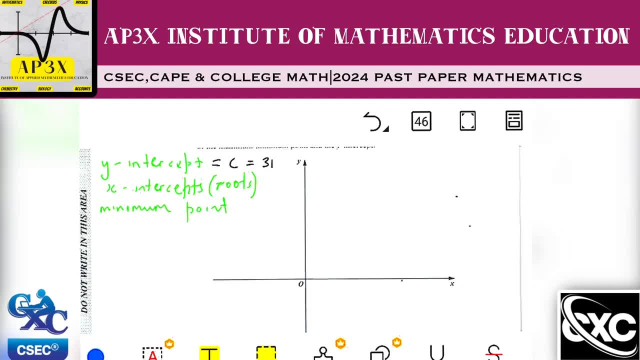 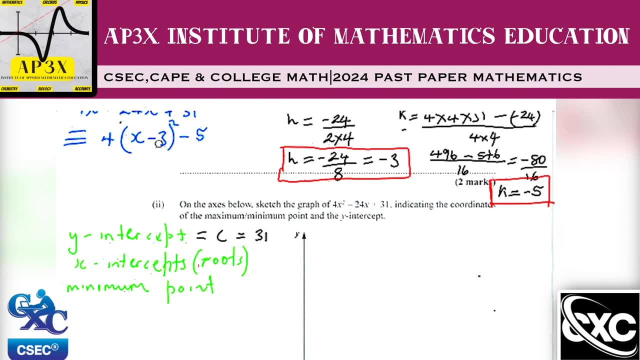 we find the x intercept by a couple of methods you can actually go ahead and uh complete the square you can sub the complete in the square equation that is up here or you can go ahead and use the formula minus b plus or minus the square root of b squared minus 4ac all divided by 2a that formula you can see in the formula sheet provided to you on your question booklet by cxc on a yearly basis just 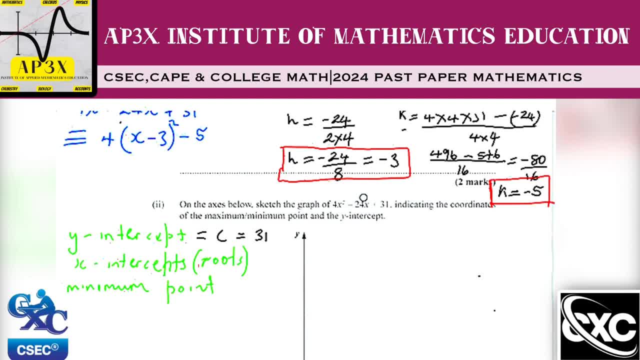 go to the front of the page or the document and you will be able to find say here the quadratic equation uh for finding the roots or finding the formula for finding the roots of the quadratic equation now i'm gonna try to use what i already 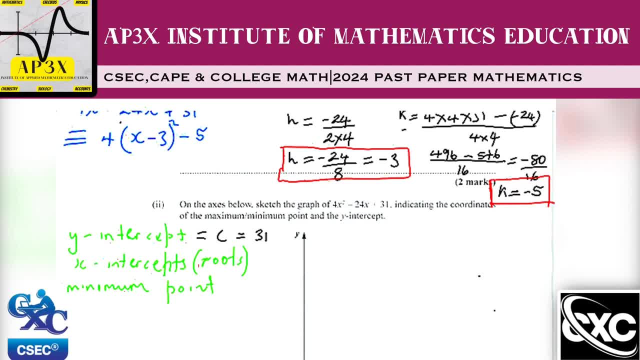 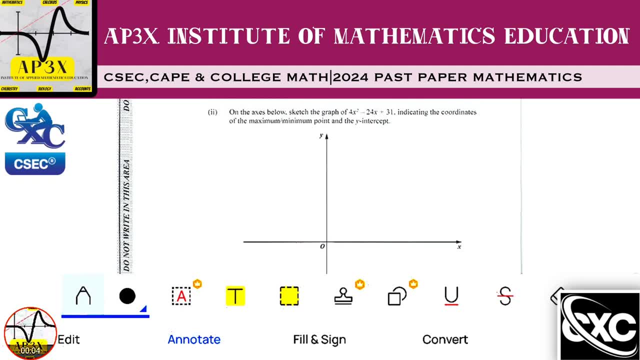 have to help me i don't want to use any additional formulas then so now that i have cleared my graph here for you let us begin the process here so as i said before the y value here we had established that the y intercept in this case so that's my y intercept that's going to be equal to 31 so because it's a sketch all we have to do is just make an estimate as to where 31 might be so this is zero we can just estimate that 31 is going to be at the highest point here that is in fact 31 let me just write then the 31 on this side here so this would be my 31 that's just my estimated point that's 31 now as i said to find the uh equation then we can therefore take say here 4x 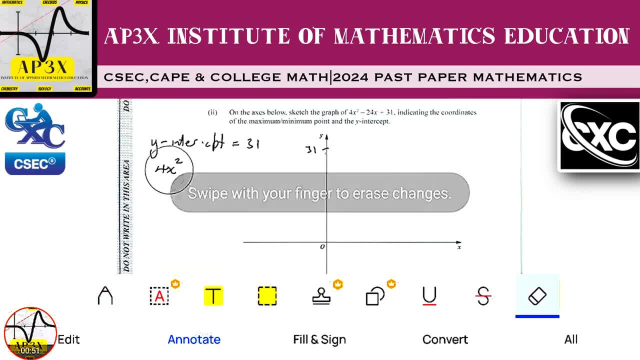 squared pardon me that's not what we had all right so i've already completed the square and the result that was provided was in fact 4 open bracket so that was 4 open bracket x uh i think it was minus 3 was it i think it was yes i think it was minus 3 and we had and that is all squared and then we had actually worked out the k value to be minus 5 as well so that was the equation that we got now as i said before i kind of want to just use what i've all the work that i've already done i'm just going to therefore go ahead and equate the equation to zero and i'm going to solve this equation now remember that's what we're looking for is the x intercept so we're looking at what point did it cross the x axis so to do this then we have to go ahead and carry the 5 over here we're going to end up with 4 open bracket x minus 3 all squared and that's going to be equal to positive 5 now i'm going to read i'm going to isolate the bracket the x minus 3 all squared by dividing both sides by 4 so when i divide the left side here by 4 the 4 is going to cancel so i'm going to be left with x minus 3 all squared and of course i'm going to divide the right side by 4 so i'm going to end up with 5 over 4 so now in order for me to 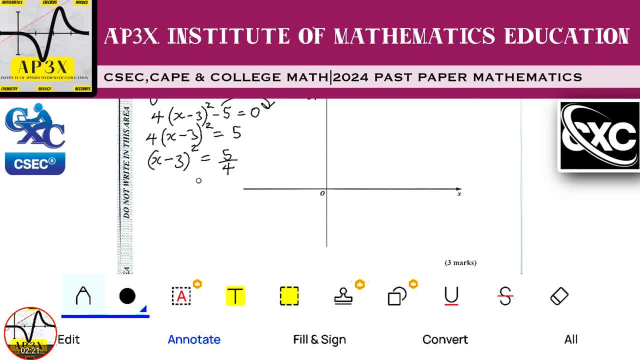 get inside the bracket to get access to the x i'm going to have to square root both sides of my equation so when i square root the left side here the square root will in fact cancel the square we've discussed this in my change of subject change of changing the subject of the formula video you can see that pinned in the comments below so you'll see that link in the description you can therefore go ahead and check out how to remove the powers from a from an expression so when i square root the left side here i'm going to have to square root both sides of my equation so when i square root the right side here i'm going to end up with x minus 3 and that's going to be equal to of course when i square root a value i'm always going to get plus or minus say here the square root of 5 over 4. now i can therefore then go ahead and subtract pardon me i can add three to both sides or some or some instructor will say transpose the negative three so you end up with the formula that x is equal to positive three plus or minus the square root of the x to the minus idea is this formula three-definitive i figure that's correct and i'll add x to the equation and i will do the next step and we'll talk about the positive three which we'll talk about when we x is equal to positive three plus or minus the square root of the x equal to minus ang transferring the愛 to the Obi radial equation and that serves to uppercase because that's the formula for than saying that the Engineer has a mind on lesson� plus or minus the square root of five over four. 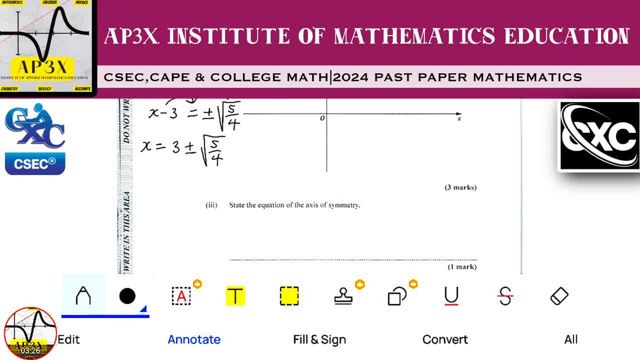 Now we can go ahead on the calculator and we can therefore say, find the square root of say five divided by four, all right? You can divide five divided by four, you're gonna get 1.25. And when you square root 1.25, you will find that the answer then works out that X is equal to three plus or minus 1.1. Now I need to get two solutions. 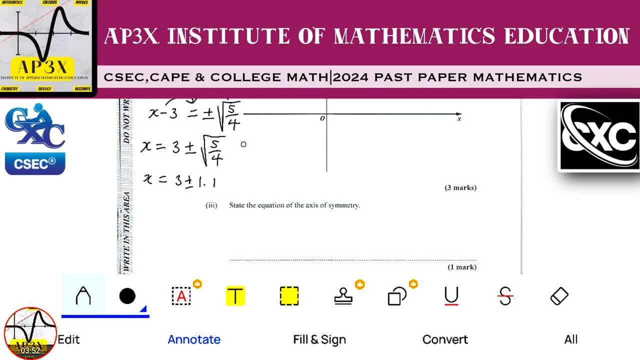 So therefore one of two things are gonna happen. Well, not one of two, both of these things are gonna occur. X is gonna be equal to three plus 1.1 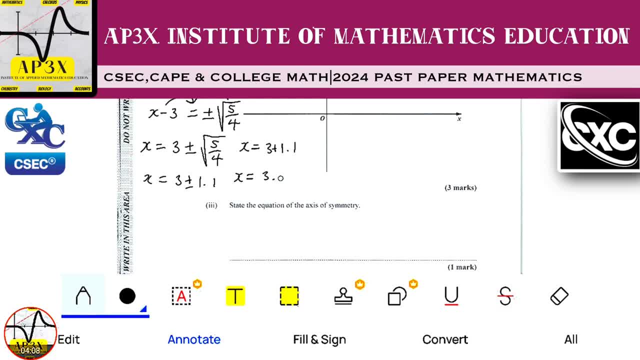 or X is going to be equal to three minus 1.1. 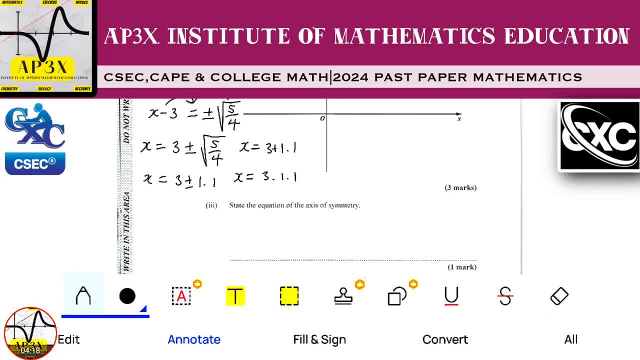 So therefore then, we're gonna work out, that X then is equal to say here, 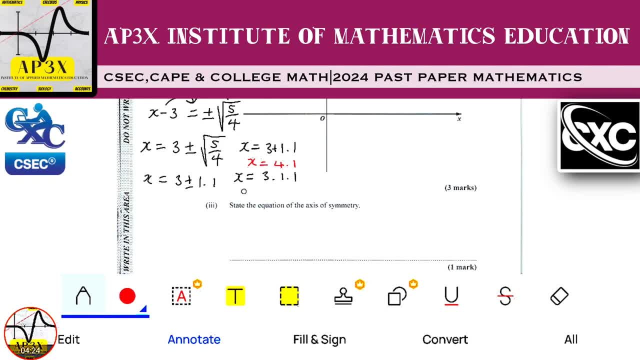 4.1 and then it also works so that X is equal to 1.9. 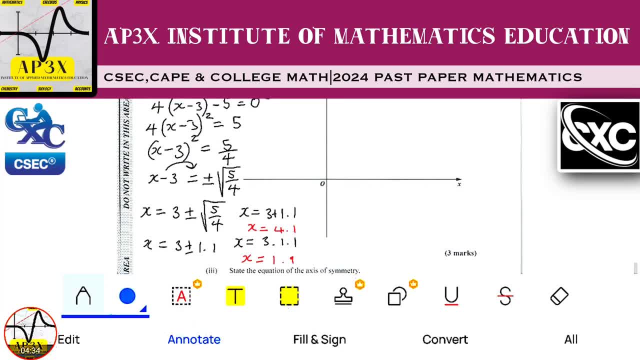 And so those two values then therefore tells me the student that I need to estimate where 4.1 is gonna be. 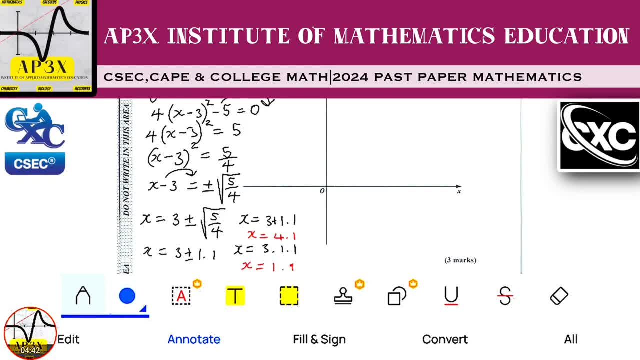 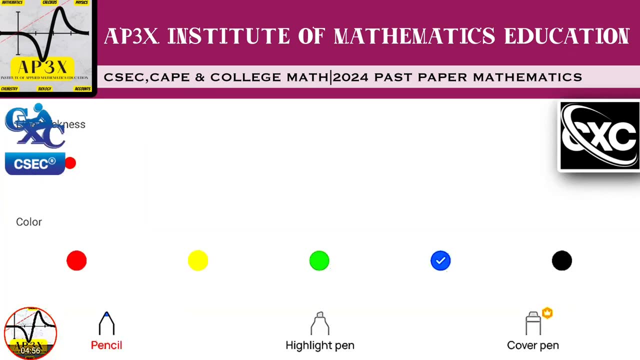 Now of course here, I can just label whatever, I can just say here that is one, this is two, this is three, this is four. Remember it's a sketch. This is say five, it doesn't have to be accurate. So if this is one and this is two, I know that 1.9 can therefore be very, very close. 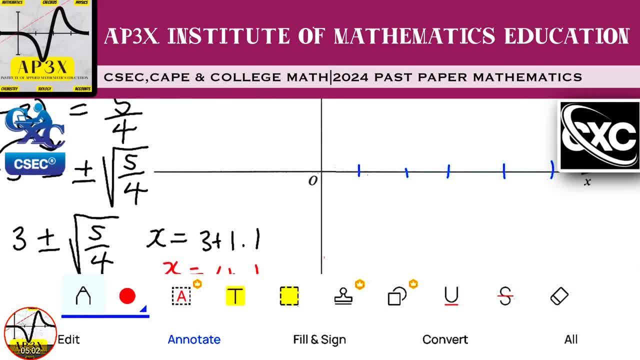 Almost, it's almost on two, but it's very, very close here. Very close knitted right there. 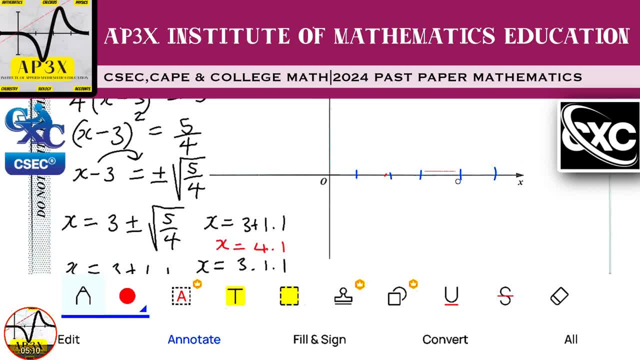 And then now of course, 4.1 is going to be, this is three, this is four. So 4.1 is like about here. All right. 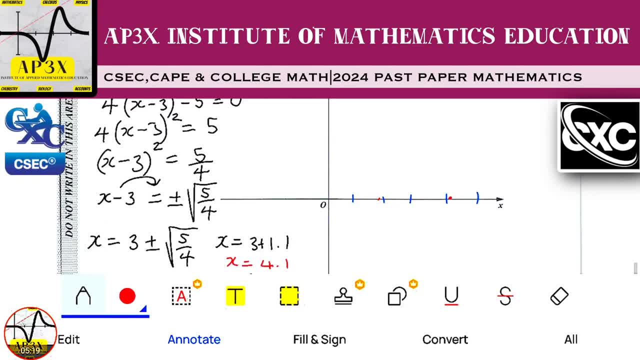 So we know therefore that we have had our two X, two X intercepts. 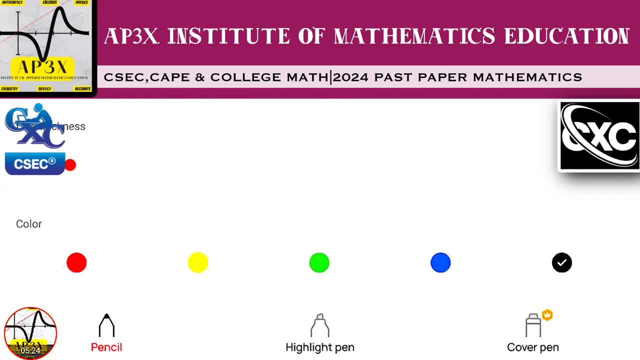 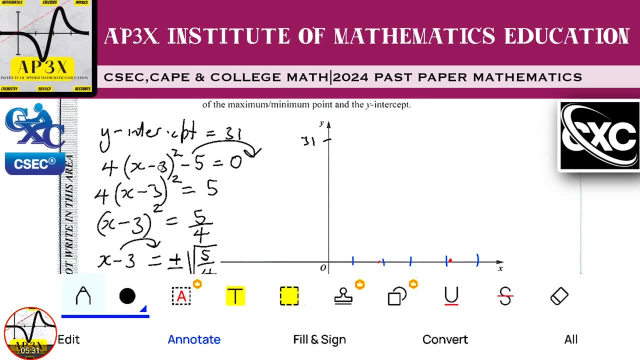 Now the next thing that I need is in fact the minimum point. And so the minimum point in short form here is a combination of this number inside the bracket and this number outside. 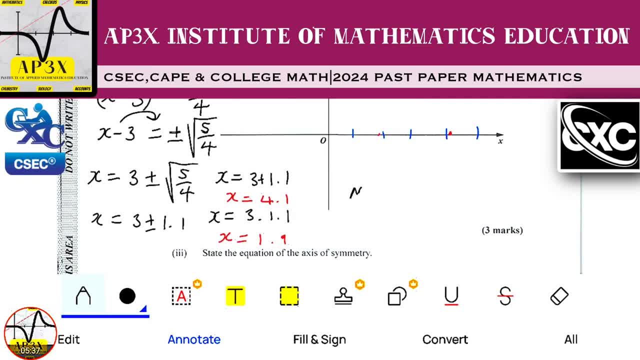 Now a better way to put it here is that to say that the min or max value, min or max, pardon me here. Let me just give myself some space. 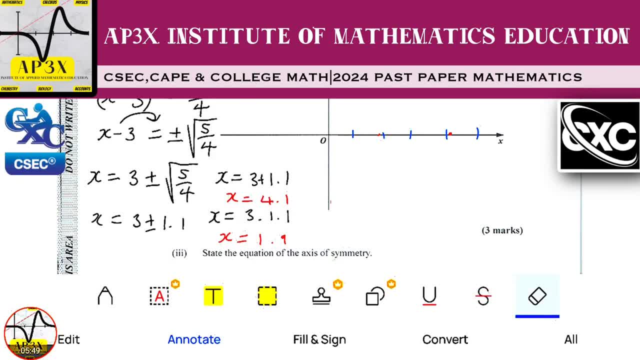 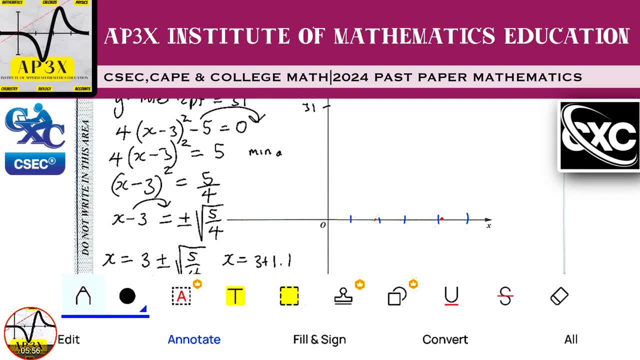 So I can just go right up here and I can write that min or max value is in fact equal to negative H comma K. 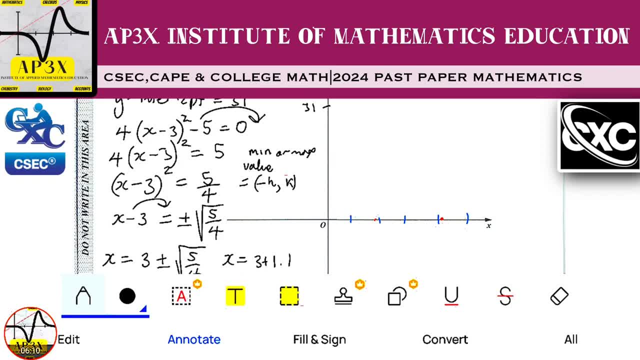 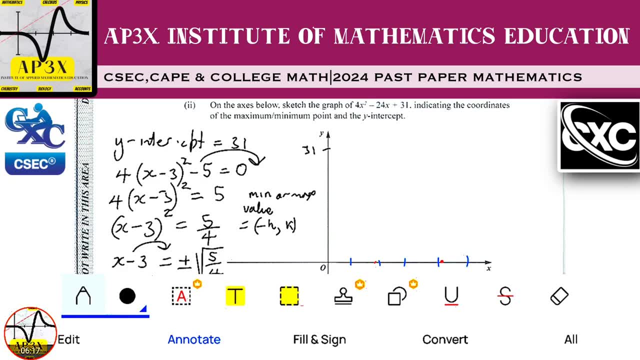 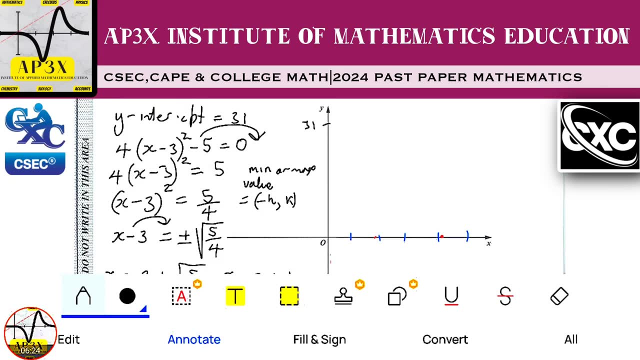 So once I know what the H value is, I just take the negative of that value. Now we had established that H is in fact minus three, minus three. And so the negative of minus three is positive three. So right away, I know that the positive three is my axis of symmetry. So I know that this is three right here. 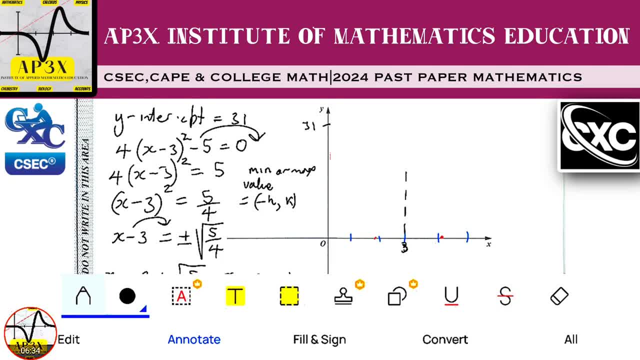 So I know that the graph basically is at this position here. 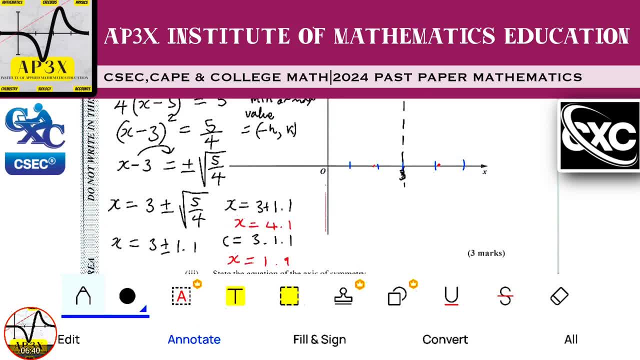 This is my halfway point of my graph. Now as to how far I go down, that is basically going to determine by the value of K. 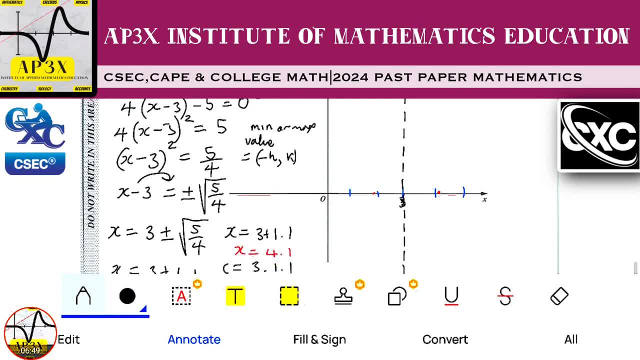 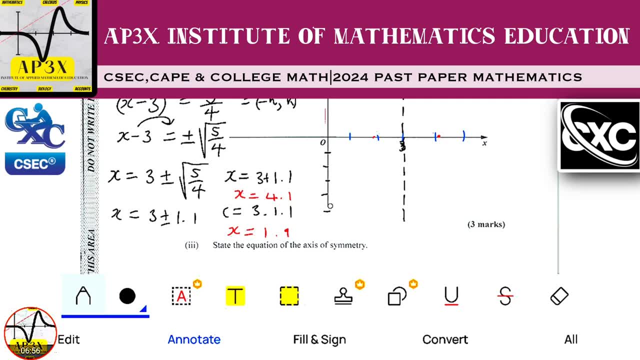 And we had calculated that K is in fact negative five. So I know that here, see this is negative one, negative two, negative three, negative four, negative five. I already know clearly that my graph will not go beyond this point here. 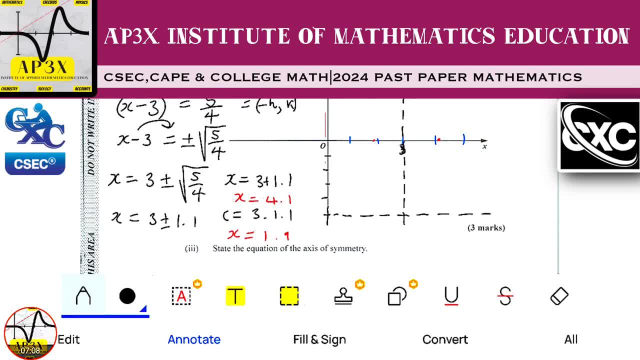 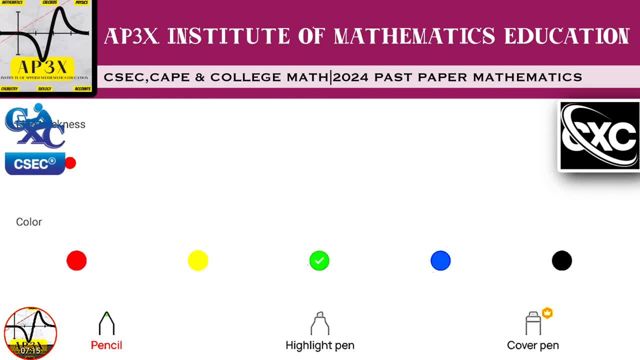 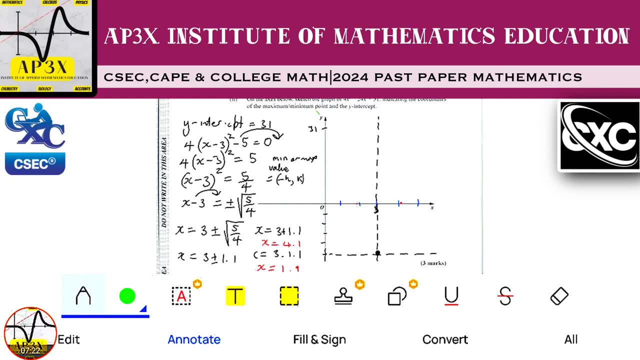 And so now that I have my minimum point, which is the intersection of say here, I know therefore that at the most reasonable sketch that I can come up with for this graph here is that in fact let me just zoom out here for you it's gonna basically the graph is gonna come down see through 31 it's gonna pass through 1.9 it's gonna come all the way down to the minimum point it's going to turn it's gonna bend up and come all the way through 4.1 and come all the way up like that all right and that's going to be like a decent sketch 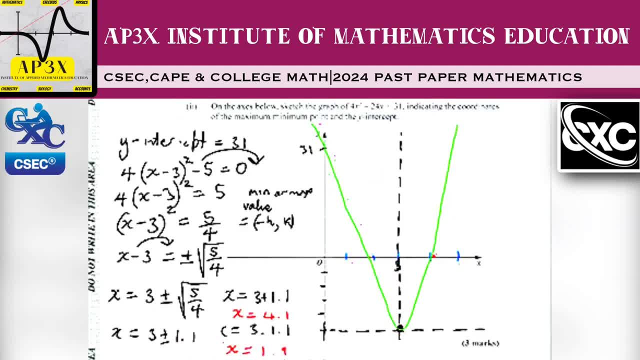 of our quadratic curve and that's what you need to go through in order to get the answer to this type of question so i hope that made it a little bit clearer maybe a bit much but definitely check out my tutorials on a weekly basis to see if you see uh a topic on this on my channel all right currented at making this video there is not an available video for 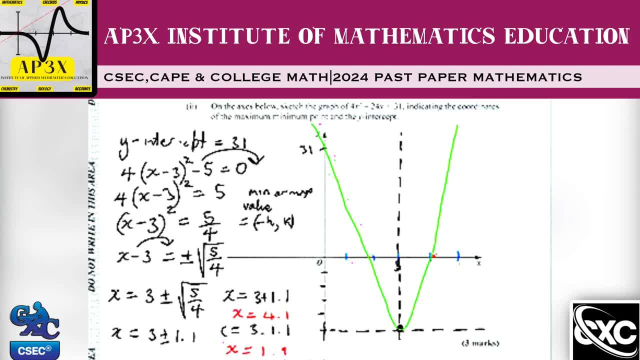 completing the script but i'll try to go on a limb and make that tutorial for you to give you a much better idea of how to do it and i'll see you in the next video bye bye 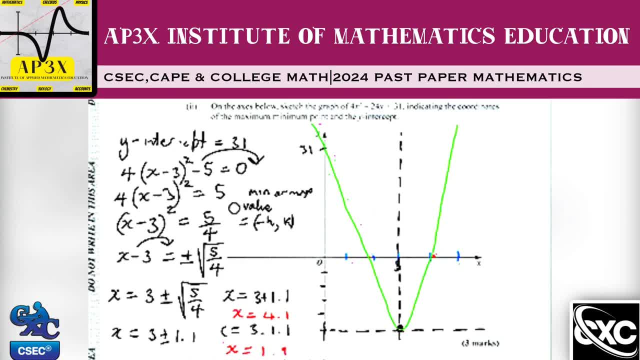 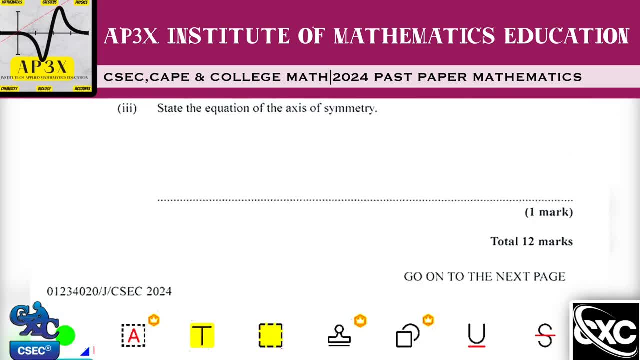 detailed breakdown version of how to find these values here all right all right beautiful let's continue on to the past paper here it says state the equation of the axis of symmetry and so the 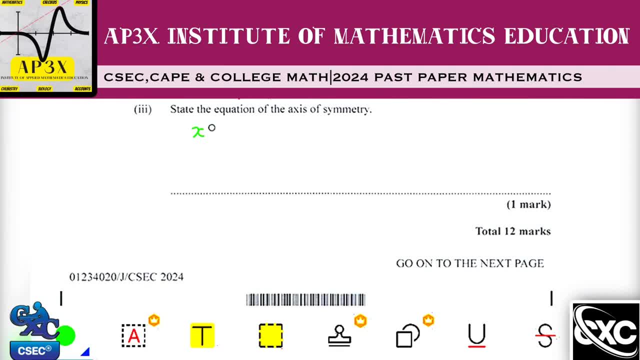 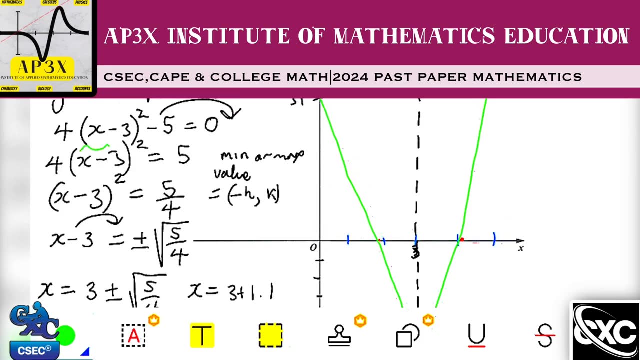 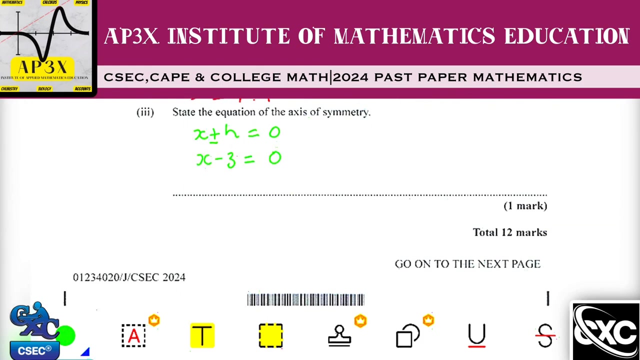 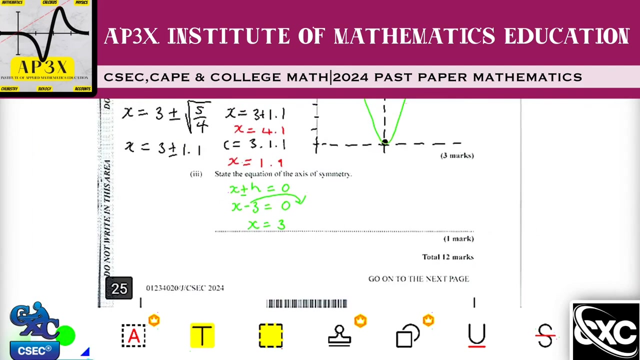 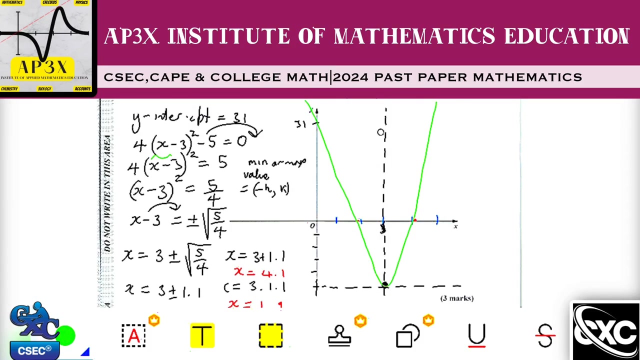 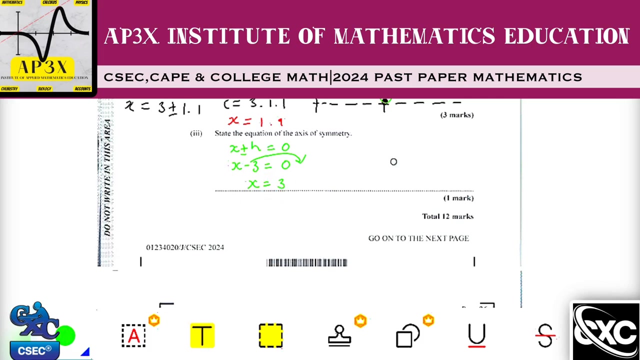 axis of symmetry is in fact when x plus h is in fact equal to zero so we know that well sorry it says when x plus or minus h is equal to zero now if we go back in our bracket here we recognize that inside the bracket here is where you find x plus h so therefore we're looking at saying x minus 3 is in fact equal to zero so the equation then is going to be x equals 3 which is kind of like basically the line that i drew on my graph here this broken line here represents my axis of symmetry but the equation of that line is in fact x equals 3 and that's what csec is looking for all right so that pretty much 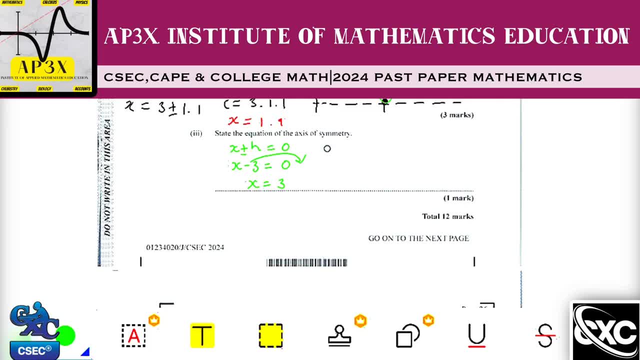 kind of sums up what they sent for functions and relations for this particular exam paper definitely keep watching or re-watch the video if you want a little bit more clarity on some of the steps that were taken all right but we have much to complete in this video 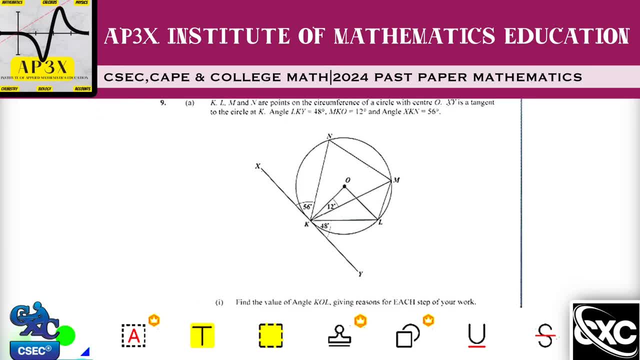 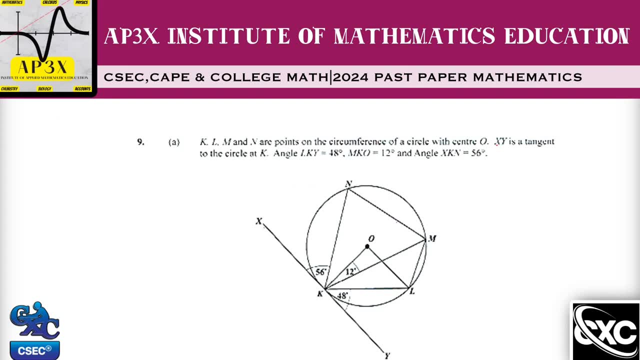 so let's just then go on to question nine now i also made an attempt to actually do this question in the latter part of the previous uh upload that is in fact part three of the video but then i didn't feel like i gave you the more concise steps so i'm going to try to make my steps very concise and to the point without going into too much theorems i felt like i gave a bit too much 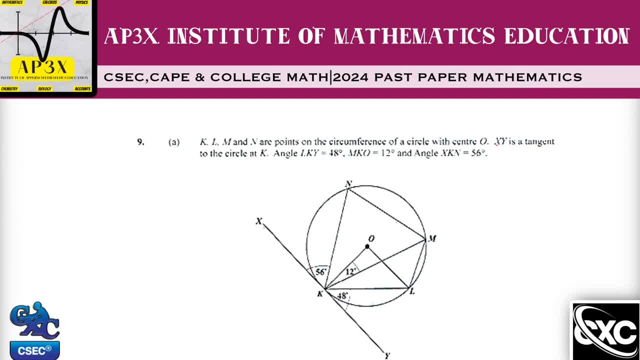 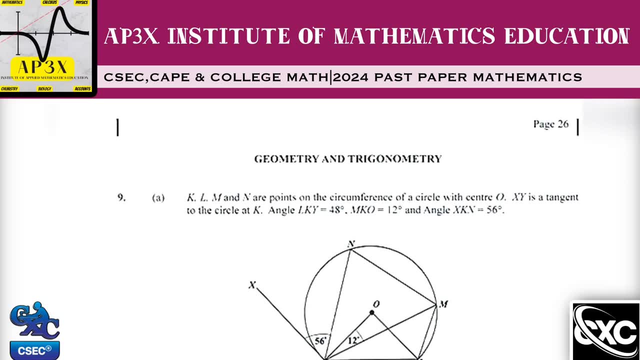 theorems for you to get to your answer so i'm going to try to make this as simple as i possibly can all right so here we go now what we're looking at is it says here that k l m and n are points 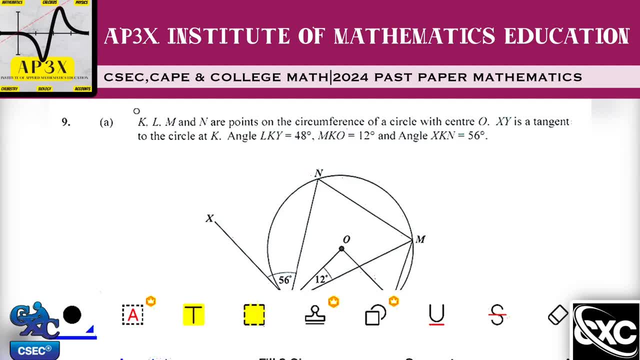 the circumference of a circle now let me pause here this seems to be a very traditional sentence that csec starts off most of the circle geometry question with and hopefully when you're doing the 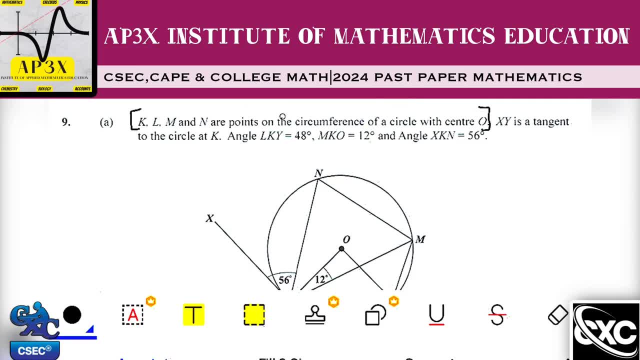 particular exam that's coming up for you when you see this sentence here already that's a clue given to you by csec they're telling you right away that if four points are on the circumference 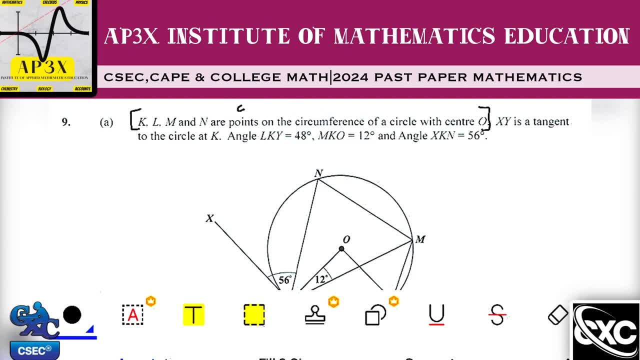 of a circle and they are connected then what you're looking at therefore then is what is known as a cyclic quadrilateral so there is in fact in that diagram below which 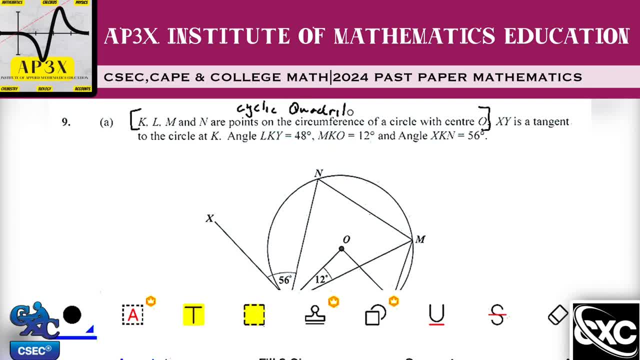 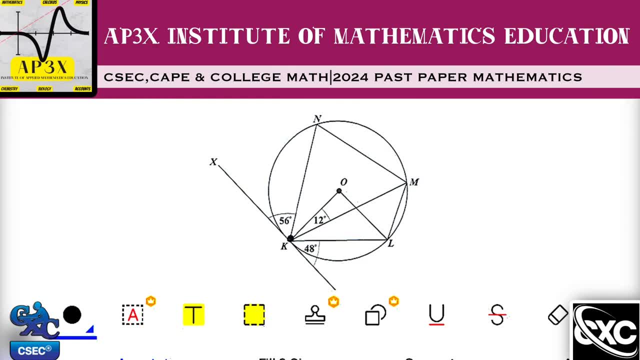 which you're looking at at the moment you will find that there is a quadrilateral that is inscribed inside the circle and so therefore we can see here that this is k this is n this is m and this is l and so your geometry is going to play an important role 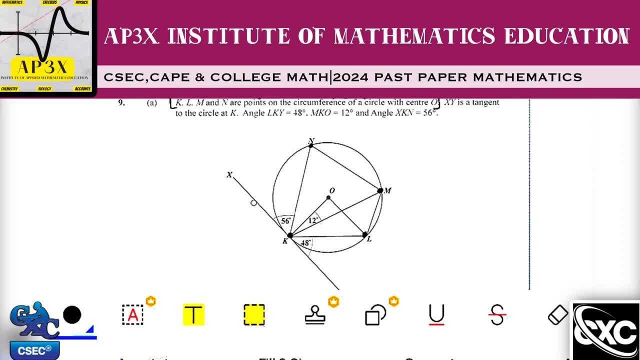 because already in the first sentence i know that there's a theorem that sticks about the opposite angles in a cyclic quadrilateral it is said that they add up to 180 so later on that theorem might play an important role the next thing it says here is that x y is a tangent to the circle so i know right away that a bit later from now i know that 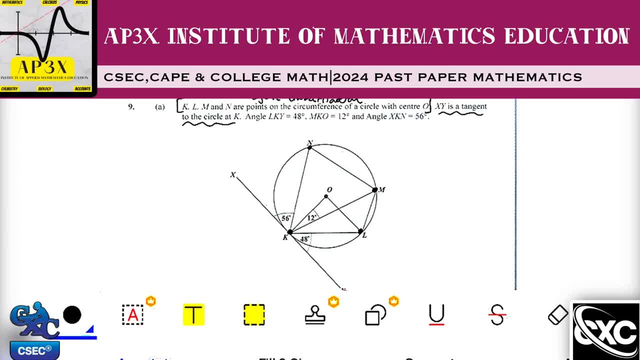 my tangent theorem as my tangent theorem is gonna come into play now i did in fact did a tutorial on the first five rules or the first five theorems on circle theorems you definitely want to check that 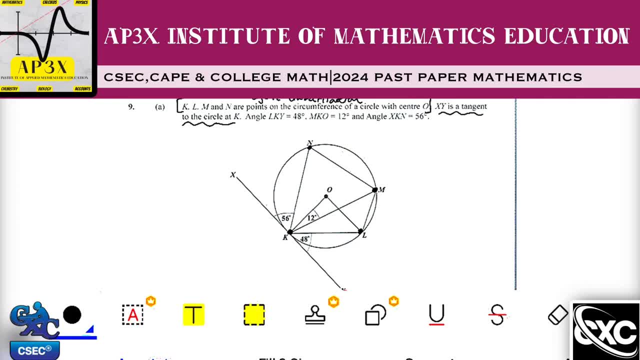 video out i'll pin a link in the description check out my tutorial on circle geometry the first five theorems and i in fact also have a video that goes through a series of these types of questions so do also check out that subsequent video as well in a time convenient to you 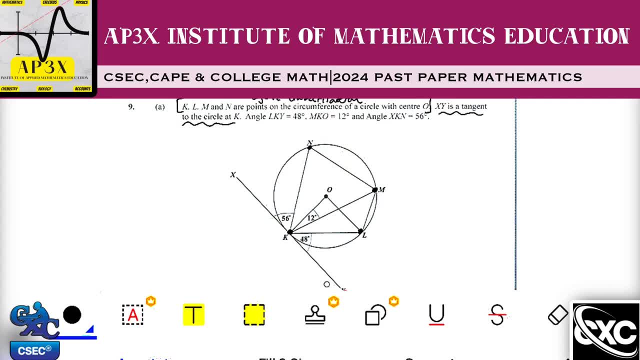 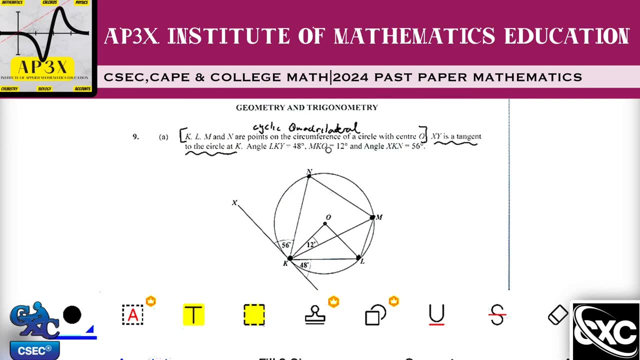 so already i know that later on this tangent is going to play an important role in the second course of course it's just gonna play a role now it also says here that angle lky is 48 degrees which we can see here so angle lky so lky is 48 it also says here that m ko m k o this piece of angle inside here is 12 and of course it also states here that i got xkn xkn equals 56 which which which we can see right here and we use the definition of that pero for this work in light of course i am using the term to yet very then after some uh point we're taking from the factors against the natural direction two ever before the little one half point nausicaa before the general shape played back sides or starting the dividends of a indycom기에 six millimeter ideal wait now the other part over here instead also comes out wipe some squared off every next unnie leads to this globalih ends theронcist mange penny 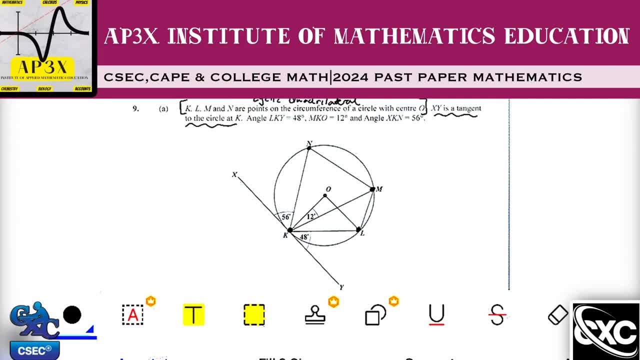 Now, in my honest opinion, remember that this particular video here is not necessary to just give you the answers and how I got my answers is to really guide you to a thought process. Some of the things you ask yourself. 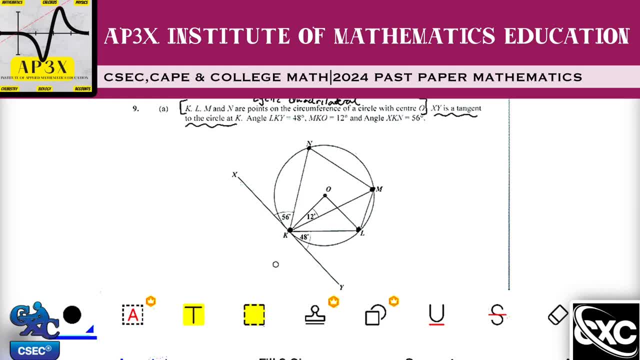 Now, in my honest opinion, I feel like this particular type of question challenges students when they are unable to dissect the diagram. You have to be able to look for certain key things inside the circle. Now, some of the key things that you have to look out for is stuff like if a radius meets a tangent or if a diameter meets a tangent or do you see any triangles? Do you see any isosceles triangles? These are some little quadrilateral theorems, some little theorems that you have to look for. 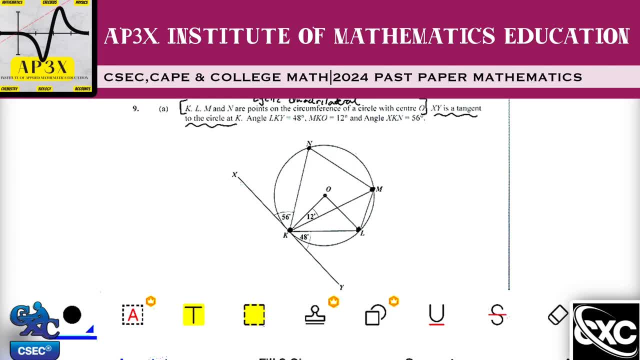 Triangle theorems, quadrilateral theorems, you know, tangent theorems. If you have to be familiar with your geometry theorems. If you're not familiar with them. Then this topic might be a challenge to you. 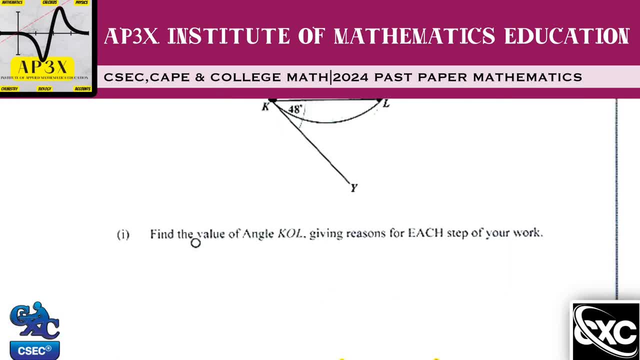 Now, here, let's have a look at what you're asking us to find here. It says that we should find the value of angle KOL. So this means then that the angle that we're looking for is in fact at the letter O. So angle KOL and you're to give reasons for each step of your work. So I'm going to take my time here. 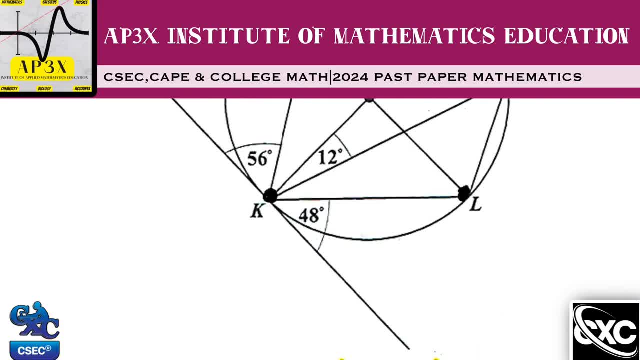 I'm going to highlight the angle KOL and so the angle is going to be right in this section here. 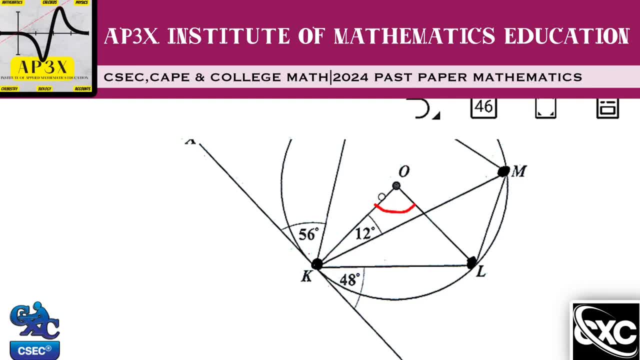 Now, when I look at this angle, I can immediately see that this particular diagram here is a triangle. Already, I know that I might have to use a triangle theorem. Now, which one of them am I going to use? 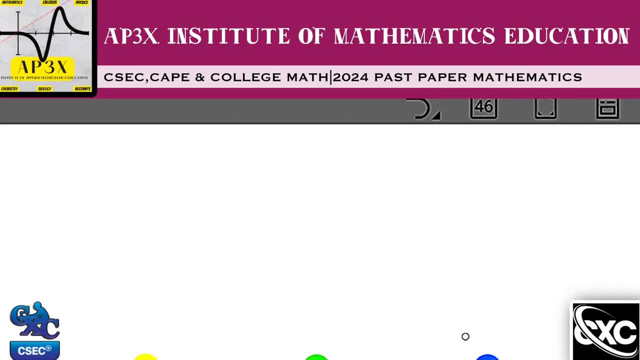 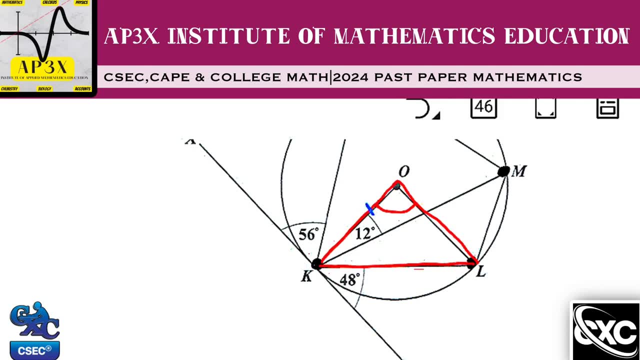 Well, one thing I do note here is that if you look closely, you'll see that OK is a radius. So I'm going to mark that with a line like that. And you can see also that OL is a radius. And one of the theorems is that OL is a radius. So I'm going to mark that with a line like that. And you can see also that OL is a radius. 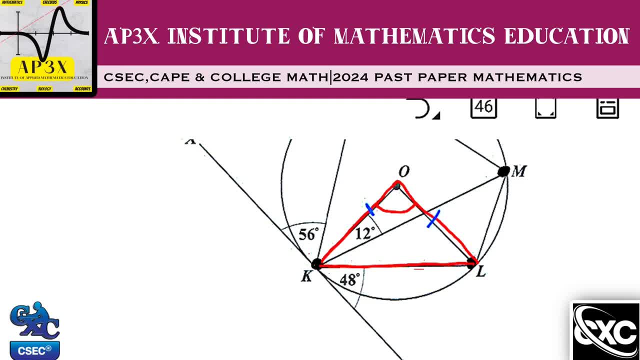 And one of the theorems is that OL is a radius. One of the first theorems that you're going to learn about in my circle theorem video, 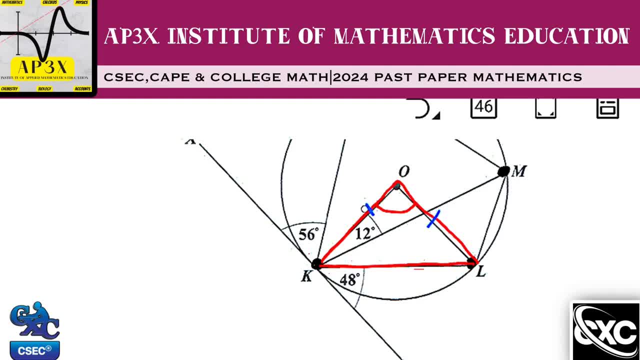 which a link is pinned in the description, you'll find that the theorem explains that two or more radii of a circle are basically of equal length. 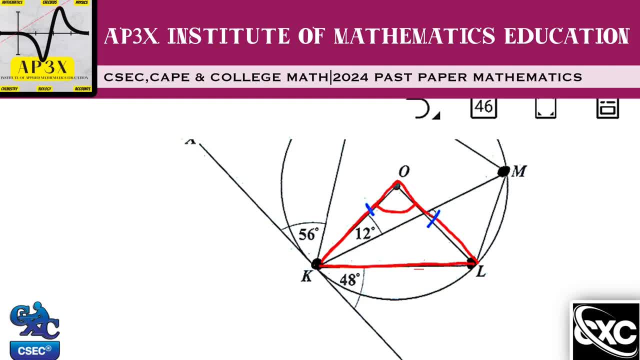 So therefore, then, since this side is then equal to that side because of that theorem, then it therefore means that the triangle that you're looking at is in fact an isosceles triangle. 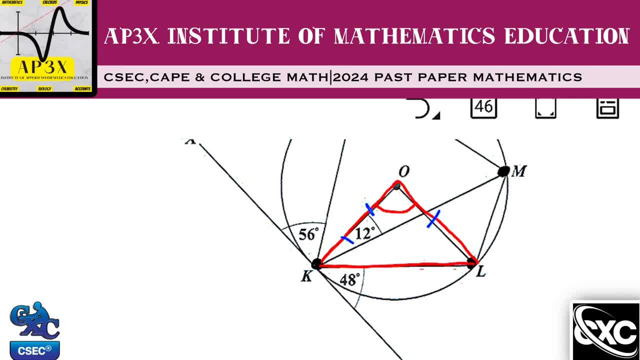 So therefore, then, this angle here plus this angle here, they are equal. 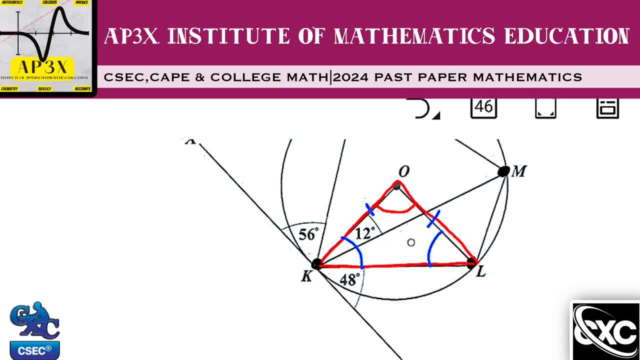 All right. That's one thing that I know for sure. So I know that these two angles here are equal. 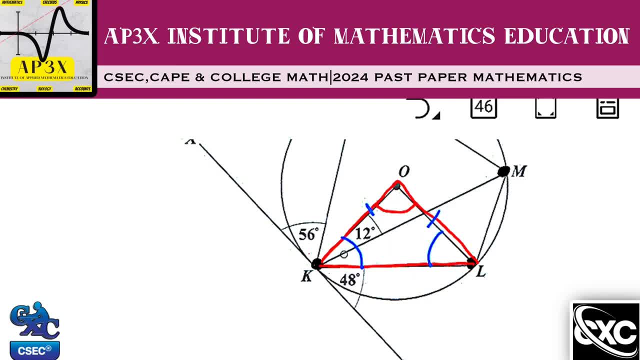 Now, the only way to find KOL is to, in fact, find these two angles here. Now, how can I find this angle? You also look carefully. 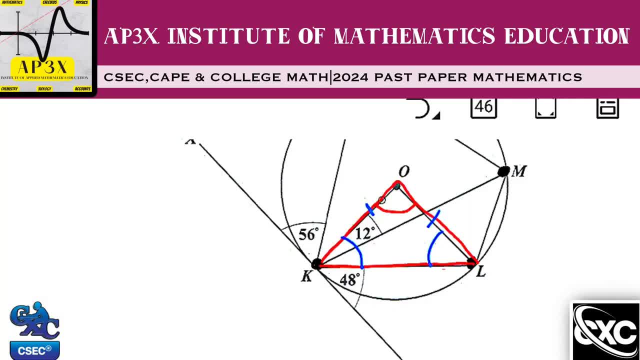 You will realize here also that since OK, the radius, connects to the tangent, then a radius is drawn perpendicular to a tangent, which basically makes this angle here 90 degrees. So if the angle that we're looking for combines with 48, gives us 90, then it therefore means that angle that we're looking for is in fact, say here, 90 minus 48. So that angle, therefore, is OKL. 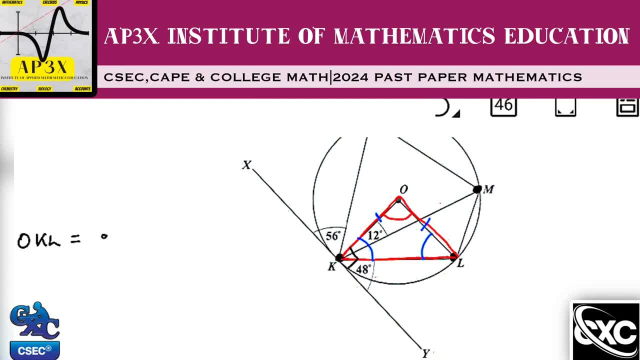 Is therefore, then, equal to 90 minus 48. And that calculation there is as a result of the radius being perpendicular to a tangent. 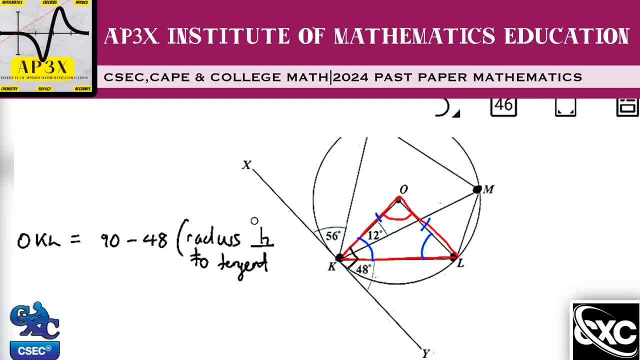 He said that we should give reasons for our answer. So because the radius is perpendicular to the tangent, we can therefore subtract that 48 from the 90. 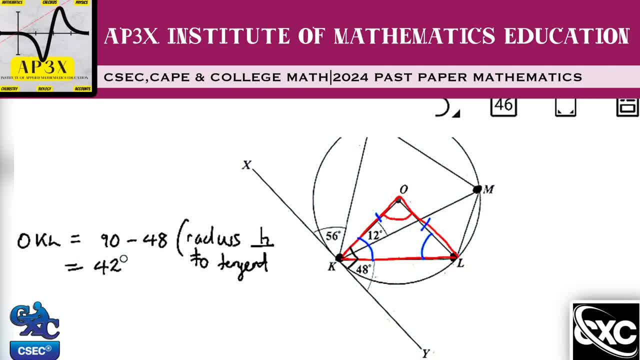 And that will therefore gives us an answer hereof. See here, 42 degrees. 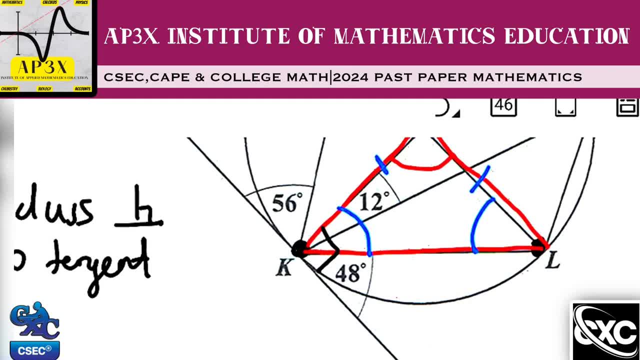 So that means this angle right in this position here is in fact, 48 degrees. All right. 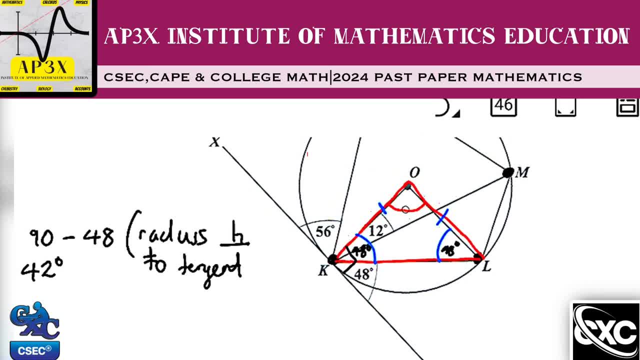 Hey, guys, so I made a little error here by writing 48 degrees when I should have actually written 42. 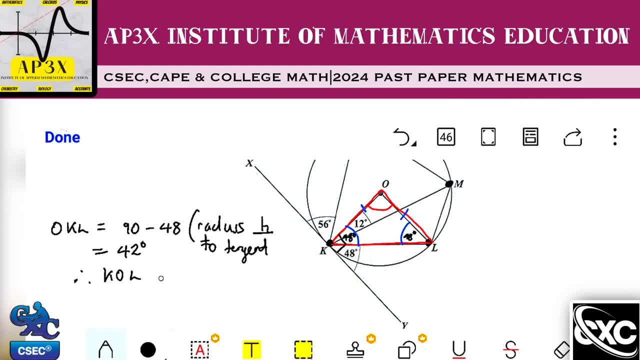 I'm going to make the corrections in my calculation in just a few seconds. So again, I do apologize for that. 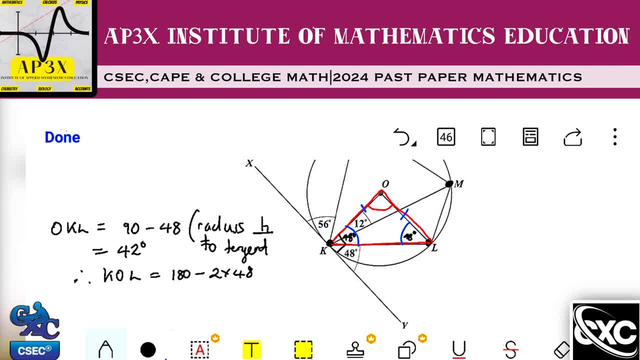 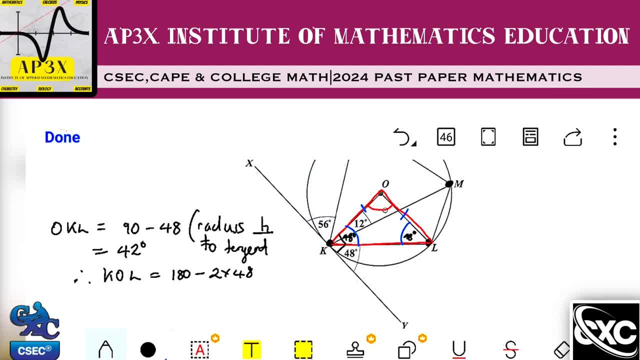 But now, of course, during the editing, I'm always going to be able to make necessary corrections. So thank you so much for leaving your comments down below for that correction. The angle is actually 42 degrees. OK. 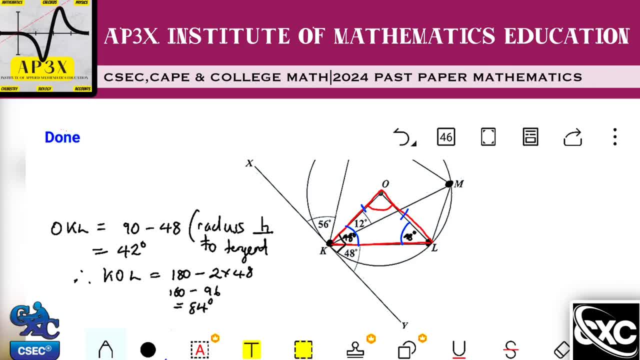 Section here to be equal to, see here, 84 degrees. So therefore, this angle here is in fact 84 degrees. 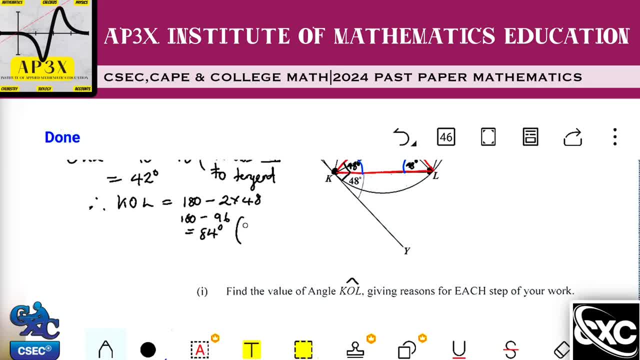 Again, the statement for this would have obviously been that the sum of the angles in a triangle are supplementary. 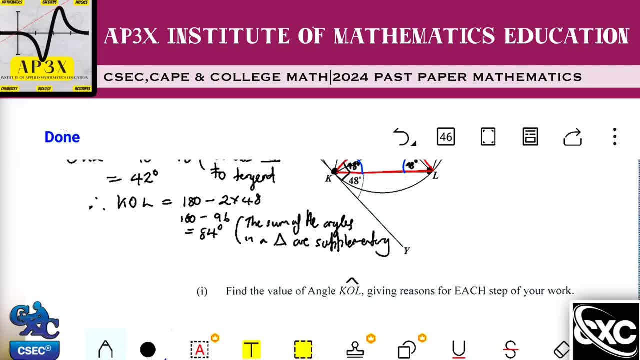 Supplementary means that they add up to 180 degrees. All right. 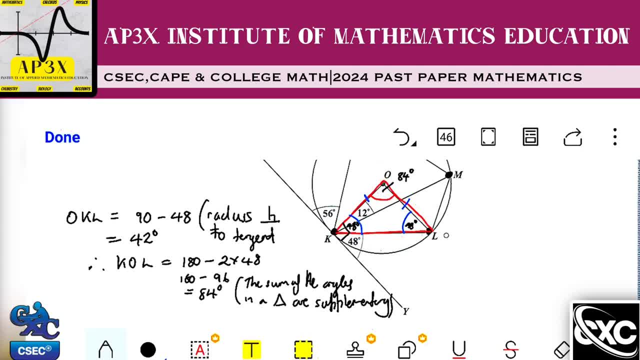 Or you could just simply say that triangle KOL is an isosceles triangle. 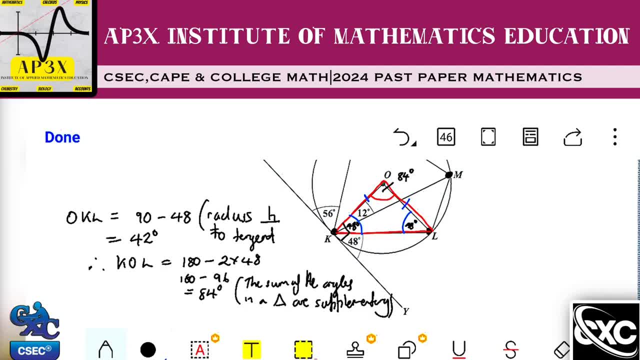 Hence, base angles are equal. That could also suffice as a geometric reason. 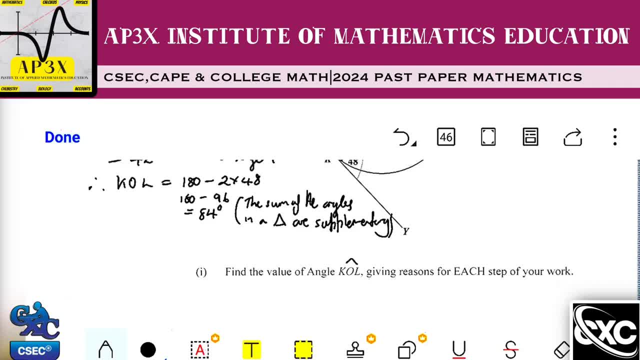 All right. So that basically answers this particular question then. All right. 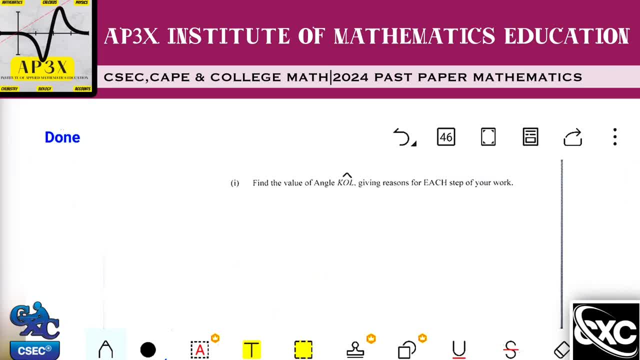 So we could write our reasons down here, as I admit, as I did not even see the space for the work, you know. But let's move on to the next question. 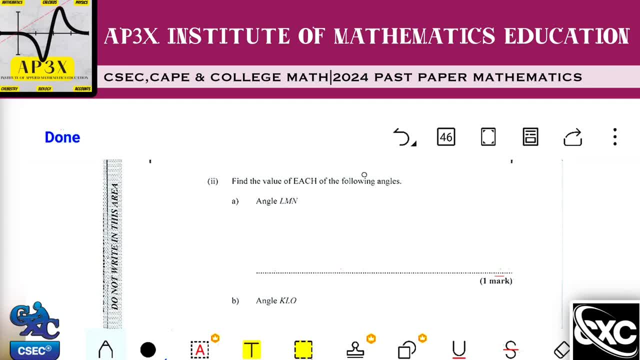 We are to find the value of each of the angles below. Now, one of the things that I've explained to many of my students that I teach live is that when you're finding an angle, when CSEC names an angle with three letters, then the angle is located at the letter that is in the middle of the three letters. 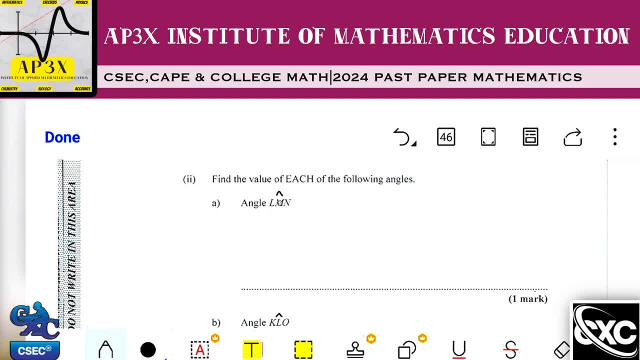 So LMN, the angle is at M. Now, many angles can be formed at the same point. So you must be able to find the start, find the end, and find where the start and the end intersect. And then that will create your angle. 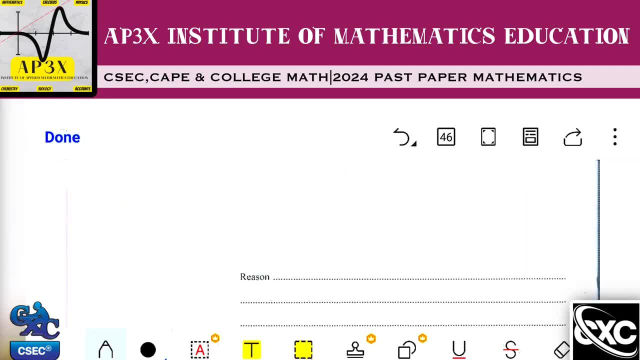 So, for example, here, angle LMN is therefore then, let's see here, let's go on our diagram. So we have L. We have LMN. Notice that I have L here. Okay. So I have L here. And I have N here. 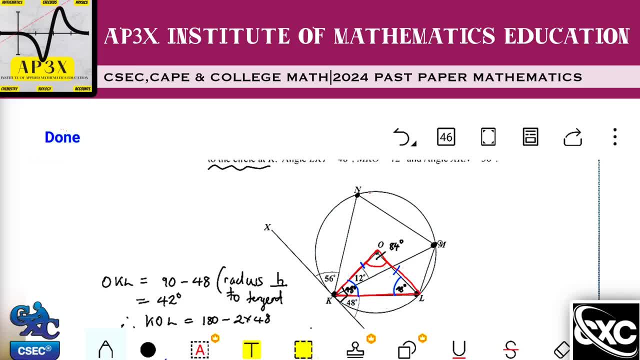 So when L and N meet at M, we basically form all of this angle right here. Now, how would I find that angle? 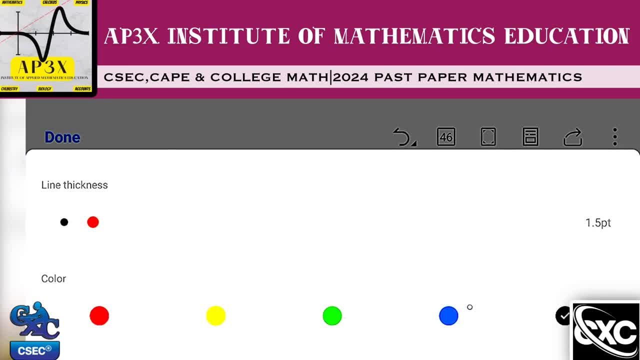 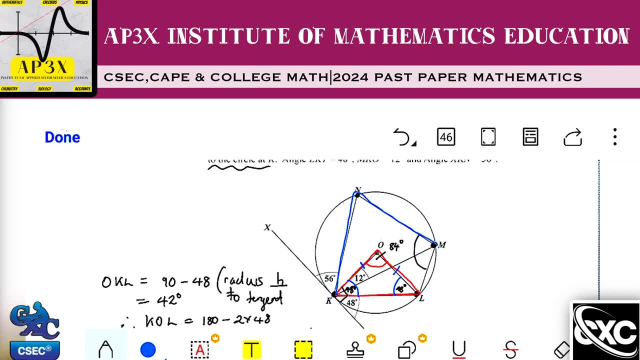 Now, it basically, and if you look again here, see carefully, you'll recognize again that this particular quadrilateral is going to come into play. Again. Because now that angle that we're now looking for is now basically an angle within that quadrilateral. 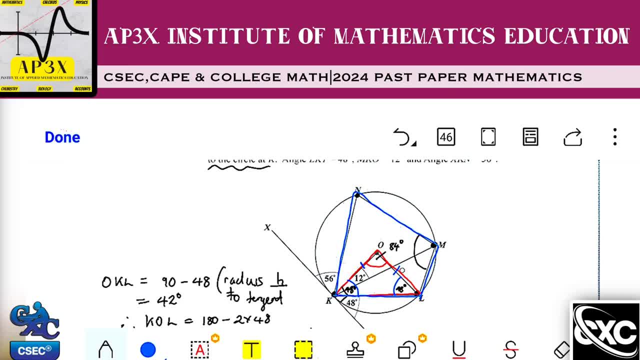 And one of the theorems that comes with finding an angle inside of a quadrilateral is that it says that the opposite angles are in fact supplementary. 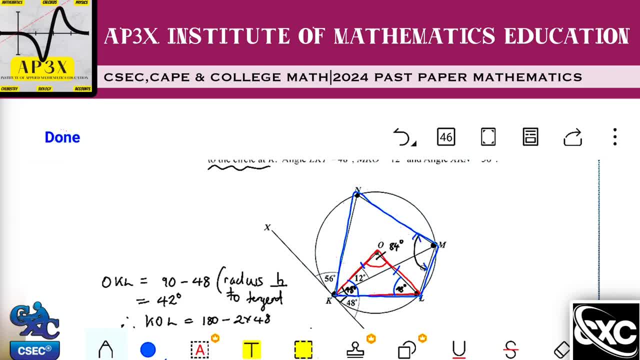 So this angle over here that we're looking for, plus all of this angle here, all of this angle right here, adds up to 180. So now, once I can find all of these angles, all of these angles here, all of these angles right here, adds up to 180. 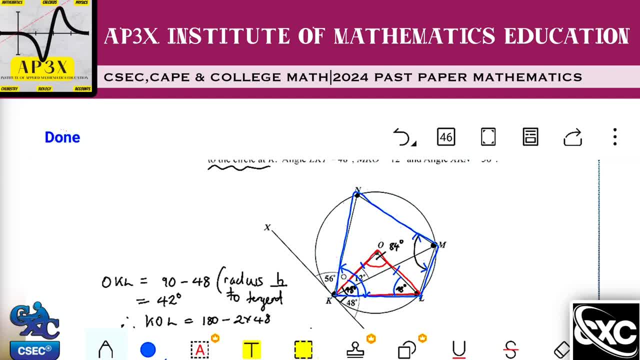 Once I can find all of this angle, which is inclusive of this piece right here, then you can easily calculate our answer. 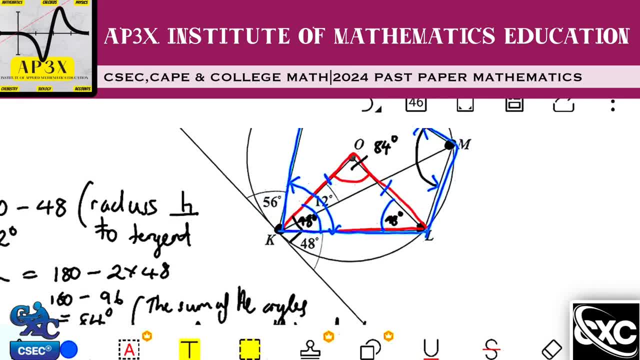 Now, let me just zoom up a little bit more here for you as best as I can. There we go. 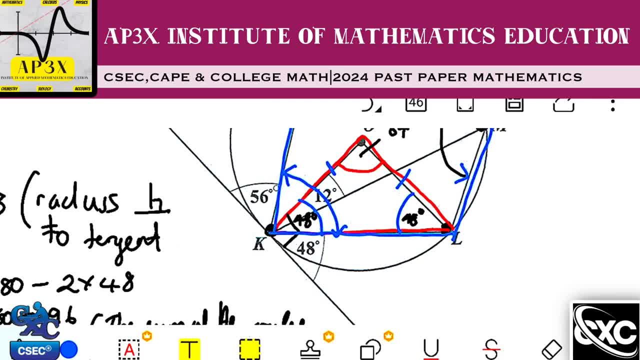 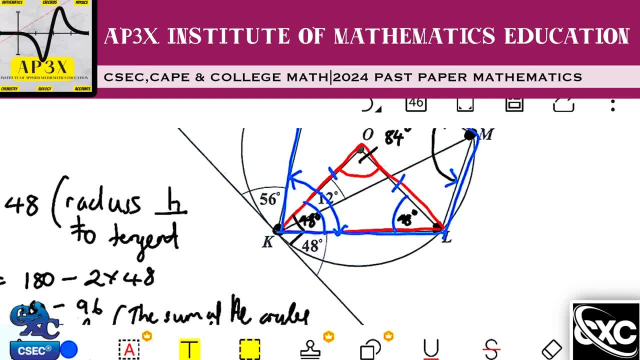 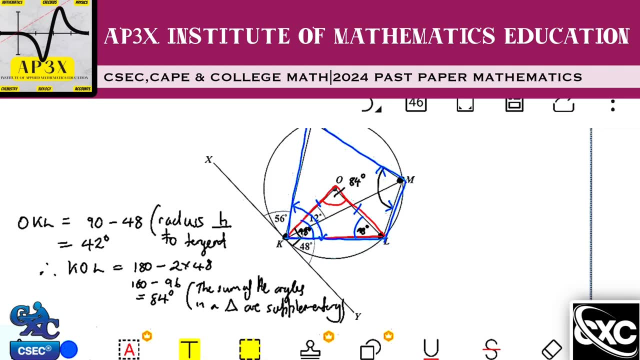 Now, if you look that the 56 degree and the angle that we're looking for along with the 48 basically adds up to 180. Because in fact, XKY is a tangent, which is a straight line. So the 56 plus the angle that we're looking for plus the 48 on the outside sums to 180. 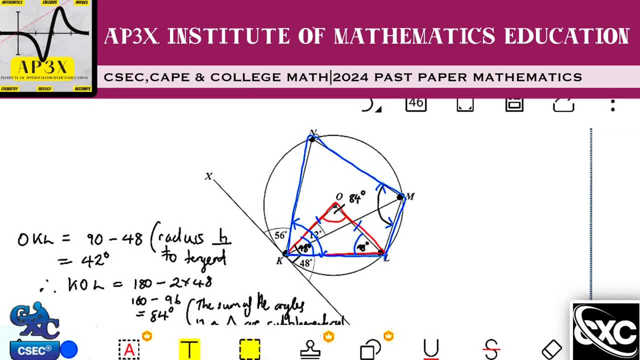 So already, I'm going to just go ahead and write my first statement that NKL. Let me just go down here. 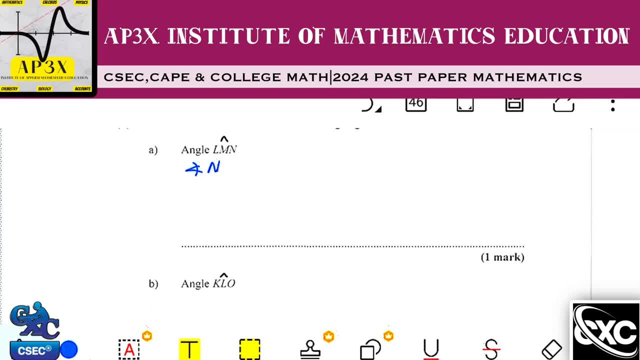 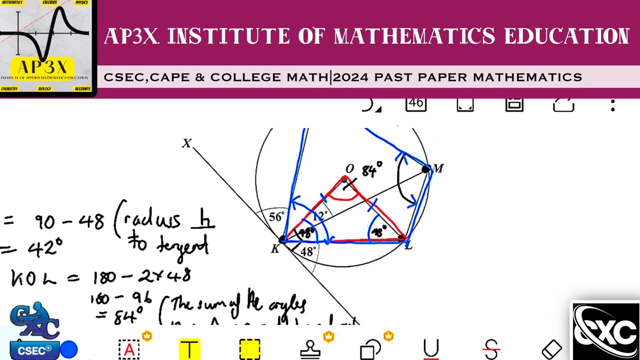 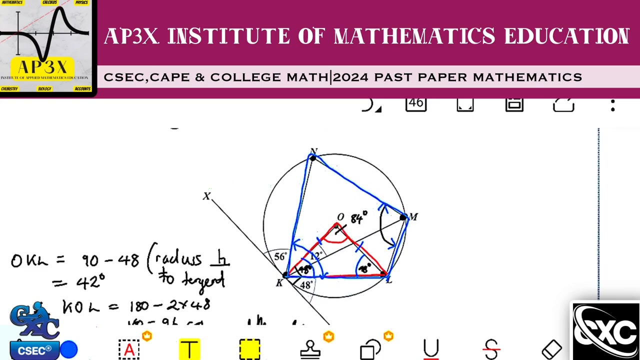 So first step is to say angle NKL is therefore equal to 180 minus 48 plus 56. So that's going to be 180 minus, say here, that's 96 and that's 104. And so therefore then, let me just double check, 50 and 40, that's 90, 98, that's 104. So 104 away from 180 gives me 76 degrees. And so therefore then, this angle right in the center that we're looking for is in fact 76 degrees. So now that we know that this angle here is in fact 76 degrees, I know therefore then that I can just subtract the 76 from 180. And therefore that tells me, say here, the angle over here. So therefore my concluding statement is that therefore angle LMN, which is what they're asking me for, angle LMN. 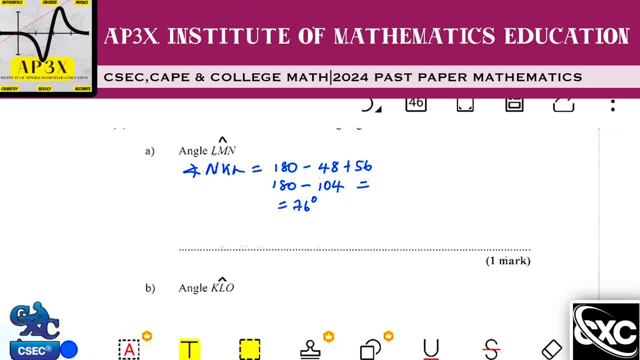 So therefore then. Okay, so therefore then, angle LMN is equal to 180 minus 76, pardon me, not 74, 76. 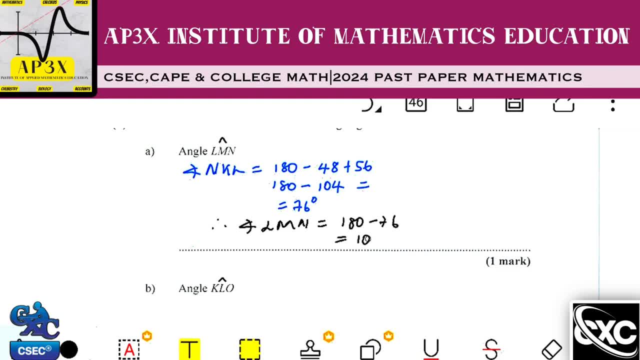 That's therefore equal to 104 degrees. 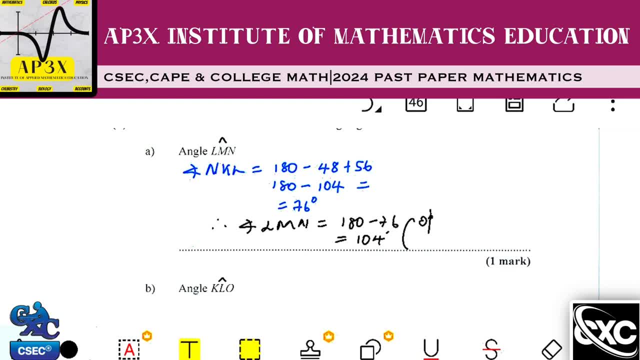 And so the reason for this calculation is that opposite. And so the reason for this calculation is that opposite. And so the reason for this calculation is that opposite. Angles in a cyclic quadrilateral are supplementary. Okay, are supplementary. Hope you guys understand that little scribble there, it means supplementary. 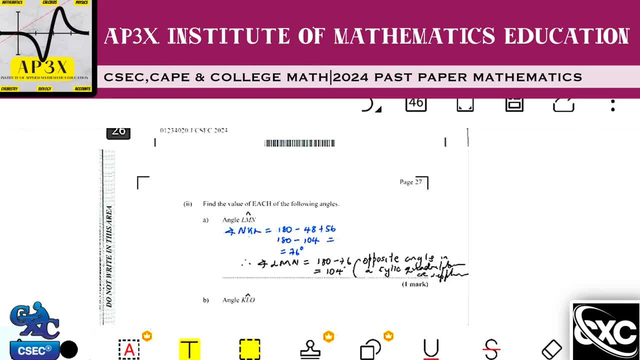 So that is how we'd end up finding that angle on that side of the diagram that you're looking at. See all of you over here. 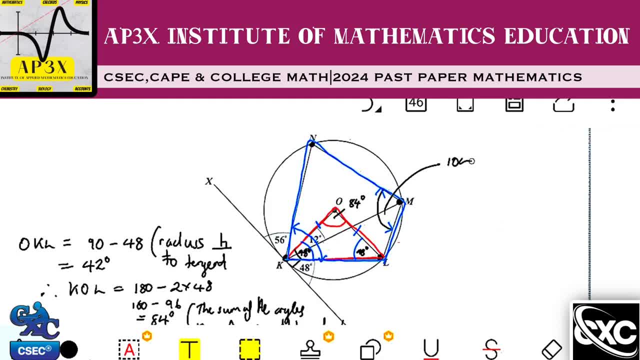 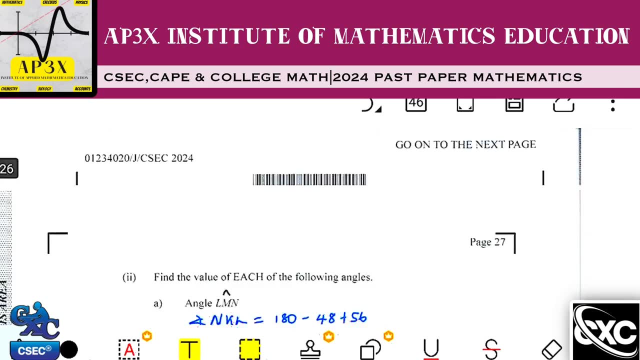 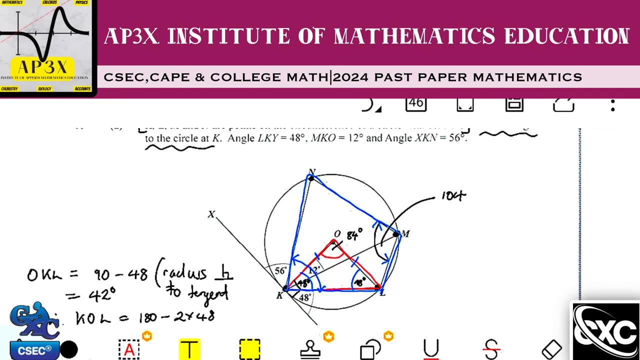 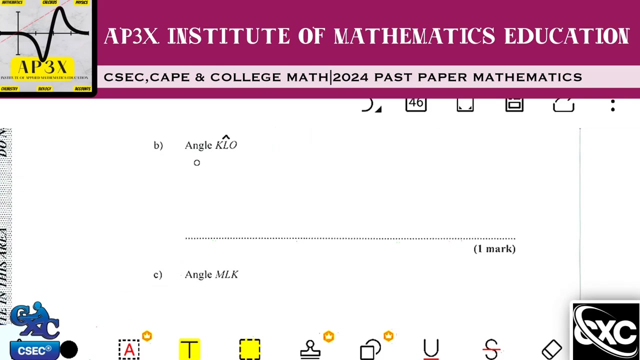 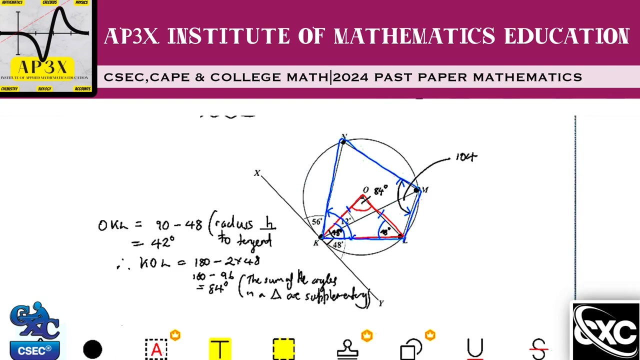 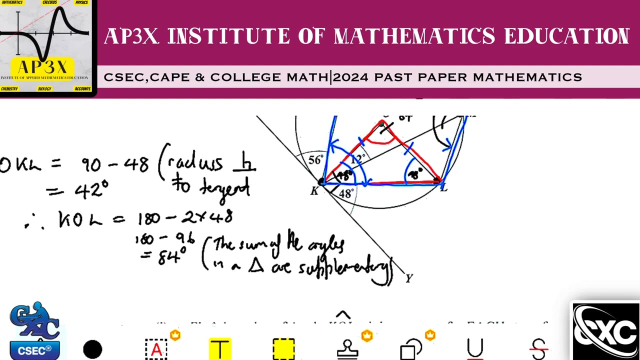 over here so all of this angle here is 104 degrees all right that's beautiful so therefore then that is it all right fantastic now let's move on then to the next question angle k lo so let's go for that let's scroll up here angle k and then we have to go down to l so go across okay right here l and go back up to o we inadvertently found that the angle is 48 degrees when we try to find angle kol so some of the work has already been done for us here so we know then that this kol here angle kol klo pardon me is equal to 48 degrees and the reason why we know that is that triangle kol is an isosceles triangle and the marker the examiner will already know that once you make such a statement then you therefore then found out already that that is 48 all right you could therefore say because the radius meets the tangent at 90 degrees then you're gonna take say here the 48 from is it 48 or 42 let me just double confirm on that it is in fact 42 degrees so it is 42 degrees I think I actually made an error here so this was not supposed to be 48 I think got a little bit confused when we did the calculation here it was supposed to be 42 so when I said 2 times 48 it 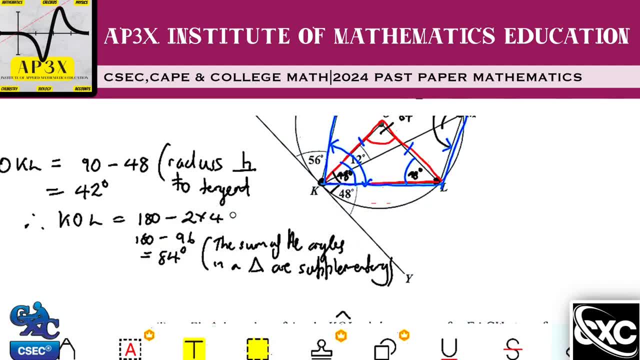 should have actually been 42 and then this should have been actually 84 and then this should have actually been 96 degrees so this should have been two times 42 which is 84. 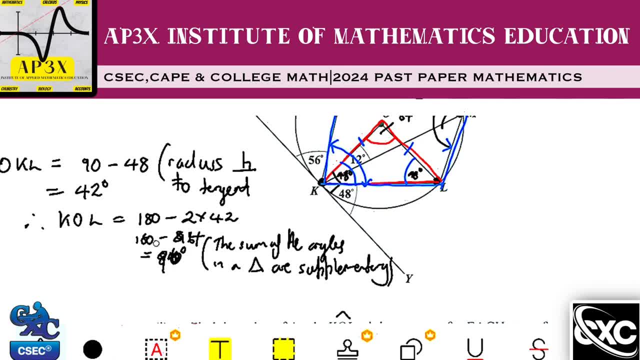 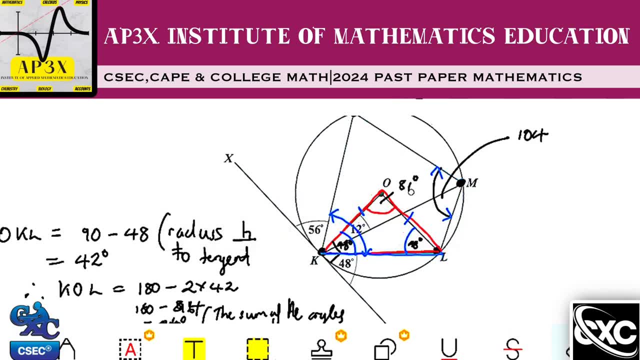 and then of course 84 from 180 gives us 96 so this angle right here is in fact 96 degrees so sometimes you have to kind of recheck it guys okay and let me just get back some of my lines here 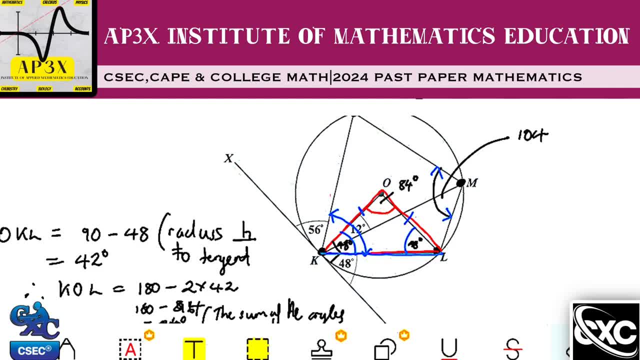 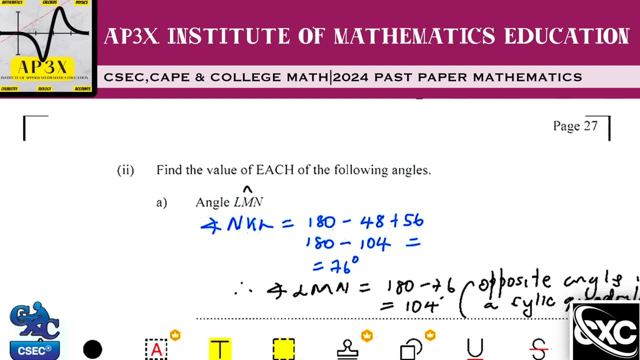 all right so this should have actually been 96 degrees instead hopefully that did not affect any of my calculations after that so that's 96 okay and we have a reason there all 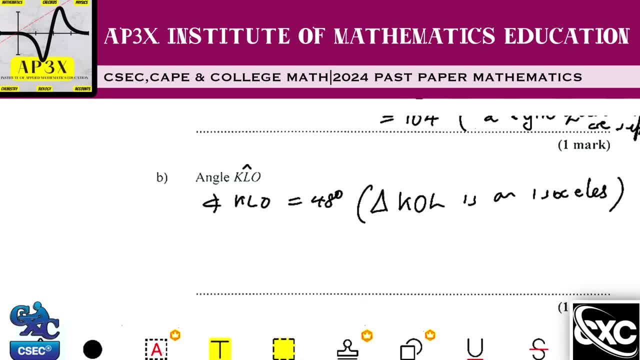 right there we have it so we're good to go so therefore then ko L is in fact then as opposed to being 48 it is in fact 42 degrees and again the reason doesn't change it is in fact because triangle ko L is I societies so therefore 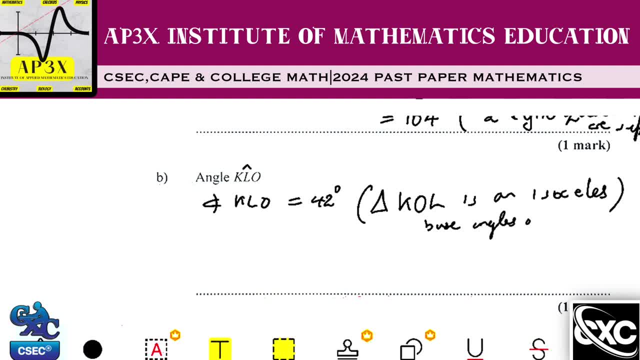 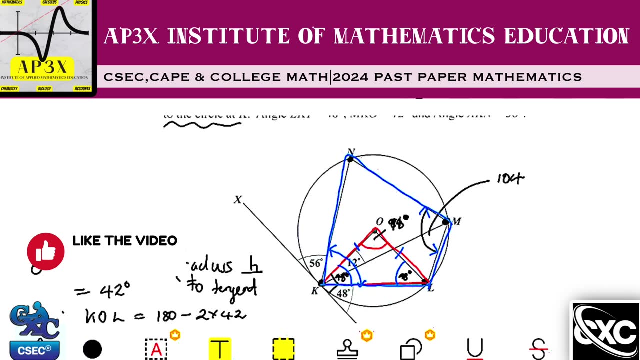 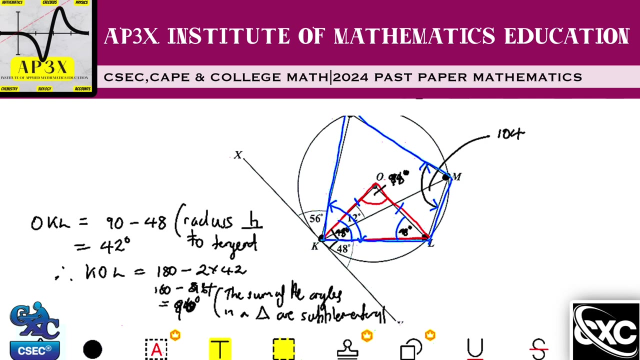 we see that these angles are equal all right so next we're looking at under MLK under MLK let's scroll up here angle MLK where is that so under MLK that is all of this inclusive of that say here 48 so it's 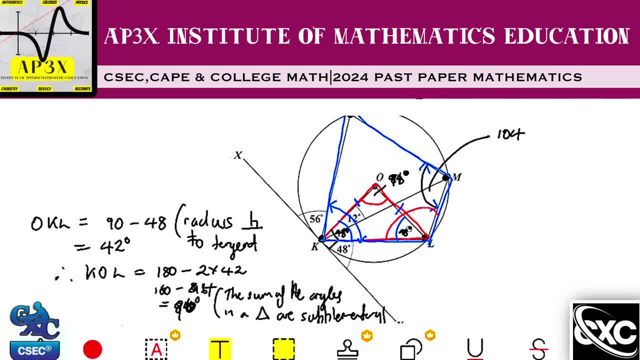 under MLK key all of this inclusive of the 48 here well in this case here it is in fact 42 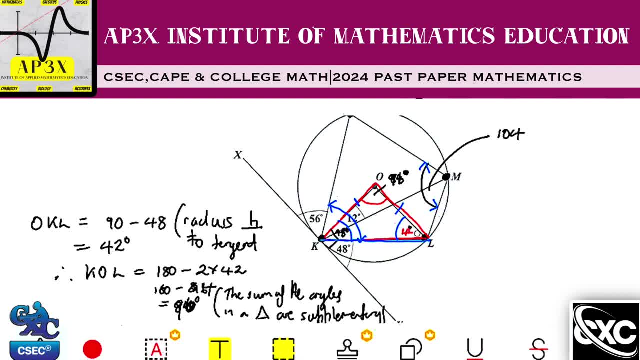 all right so it was supposed to be in fact 42 so the angle we're looking for is inclusive of 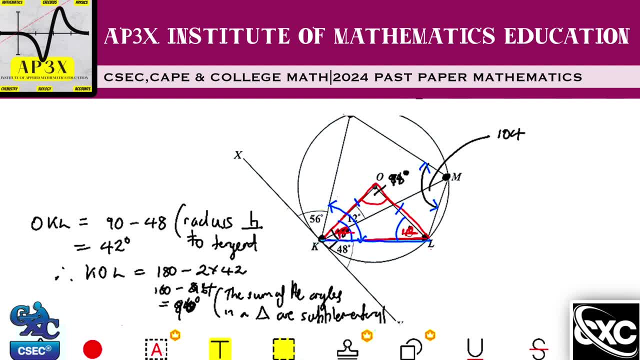 this 42 degrees that we have here so now all you need to know is to find a way how to find this angle over here so we're looking for all of this angle here inclusive of the 42 so i need to 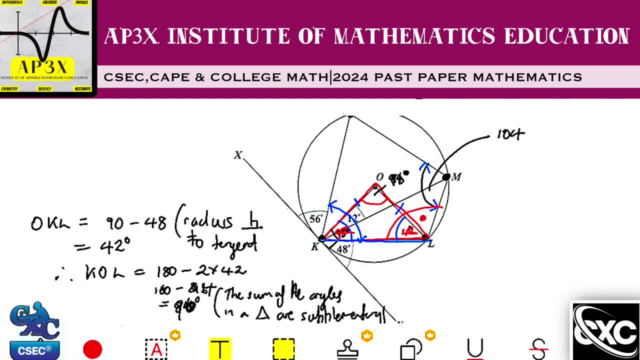 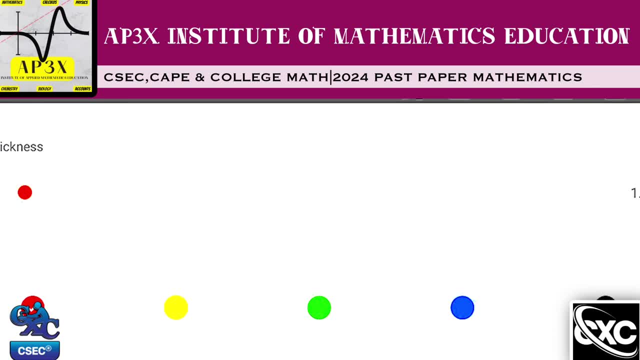 find this angle right in here now it's a little challenging to find that angle right so what i'm going to be doing is that i'm going to be using my tangent theorem here and my tangent theorem 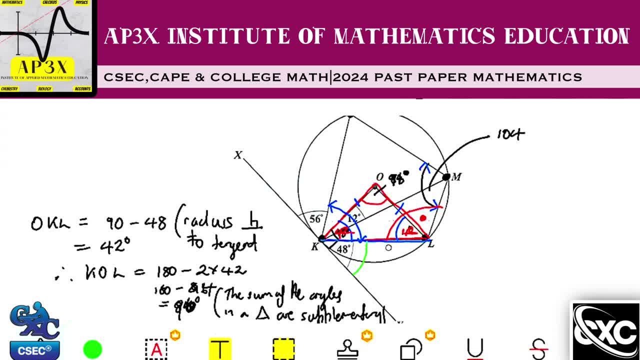 states that if i have an angle that is created between a chord and a tangent 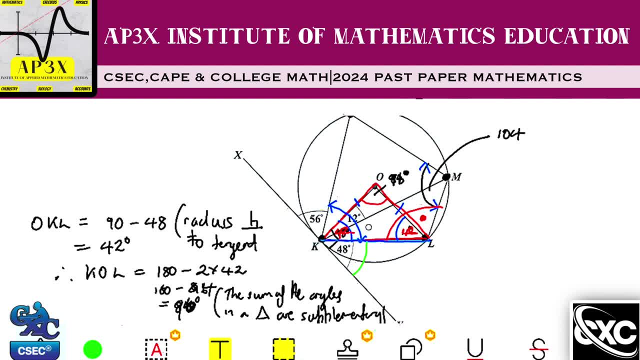 then that angle is going to be exactly equal to the angle that that is created by the chord in the alternate segment so this 48 degrees here this 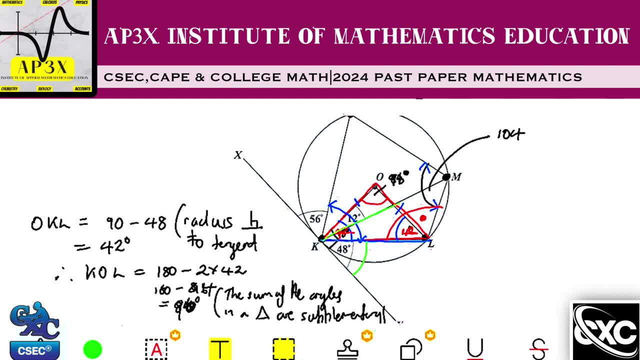 chord here kl created an angle all the way up here so this angle right in here is in fact also 48 so let me just go ahead and write a statement for that 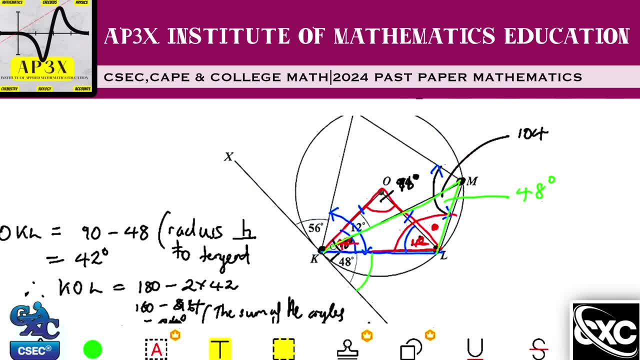 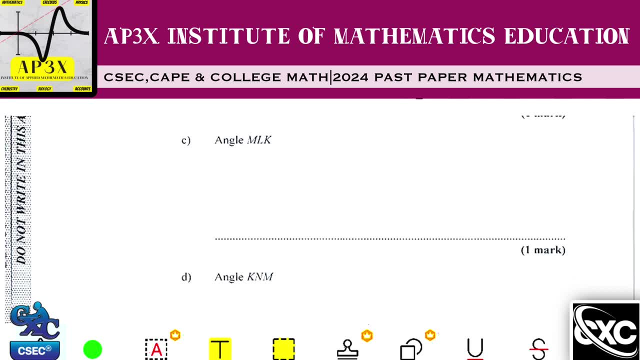 so we can name this angle here an inadvertent angle that we have to calculate so it is k ml that's our statement that's our starting statement so angle k ml is in fact equal to 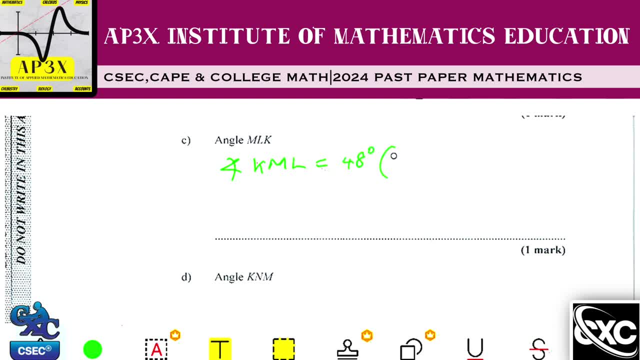 188 degrees and that reason is simply because the angle between a tangent 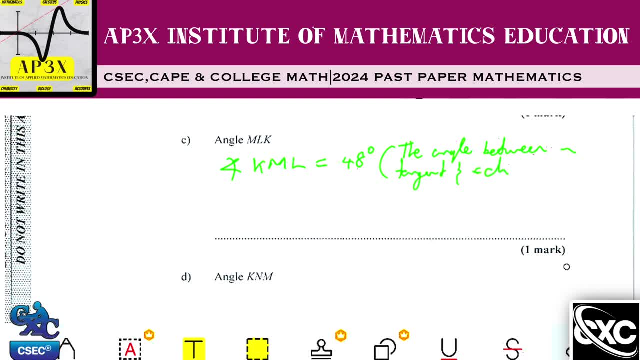 and a chord don't know what word is that that i just spilled guys so the angle between a tangent and and cord is equal 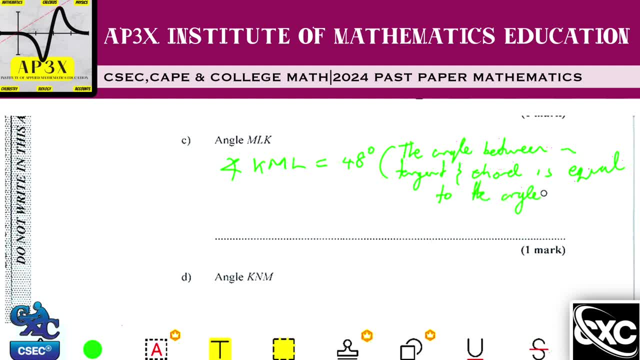 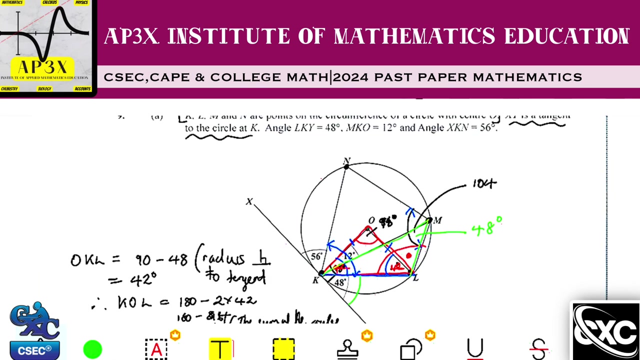 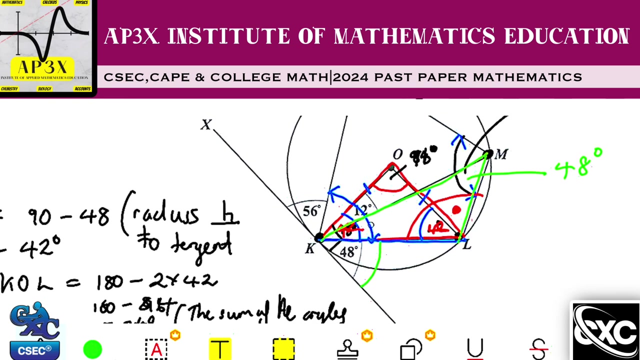 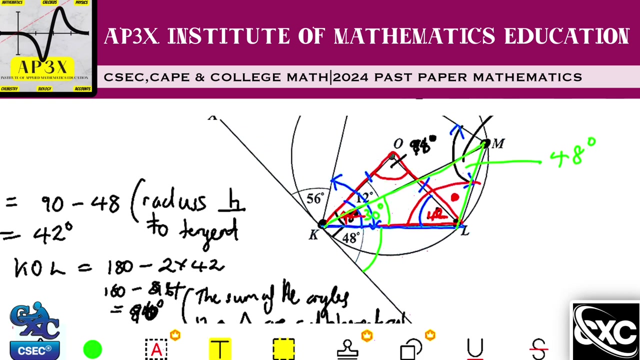 angle in the alternate segment in the alternate segment all right so that would be the geometric statement for that now once I've calculated that angle of 48 degrees that angle is going to be brutally helpful because now that angle is 48 I then already know that this angle here is 48 this angle down here we can eat this angle this piece below the 12 here we know that all of it is 42 and I've already calculated 12 out of it so now that this little piece here in here is actually equal to 30 degrees so that 30 plus that 12 is equal to that 42 so this angle in here this green triangle is 30 so now I have 30 I have this angle of 48 and I have a partial angle here of 42 so therefore then I could then add up all of that and take it from 180 no or I could just simply add the 48 which is what I'm doing I'm gonna be adding the 48 degrees here and this 30 degrees that I've just inadvertently calculated and take all of that now from 180 and I'll get the full angle that I'm looking for so we have a couple of statements to write here from triangle KML 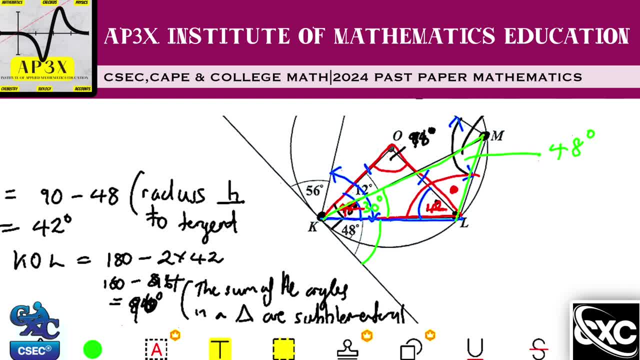 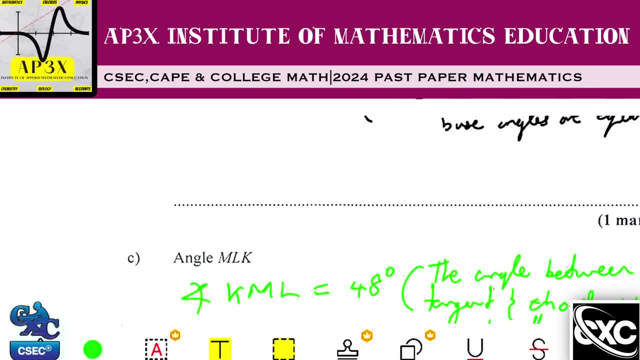 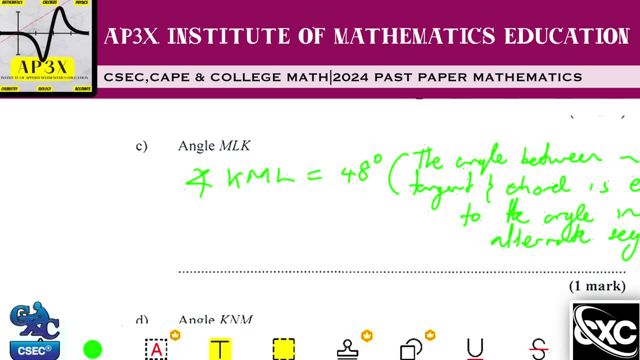 alright so we can just instead of just state in the triangle we can see angle K L M so let's go down here so we can go ahead and unsee angle key think I'm a little confused here guys hold on let me just get my triangle in here so I just 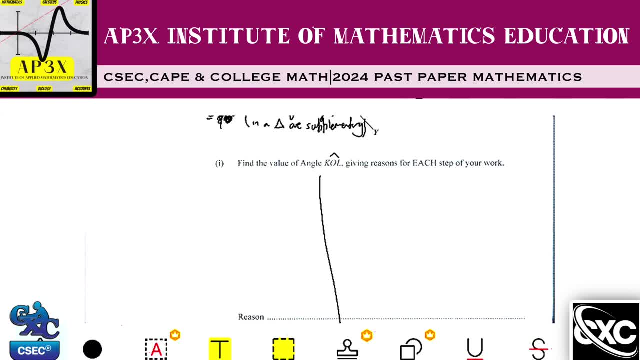 my triangle again my digital I'm not used to this new digital device that I 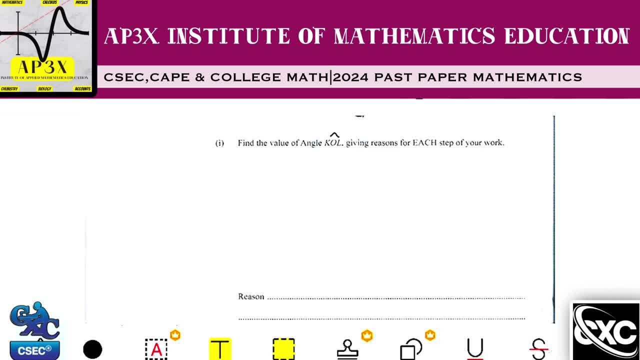 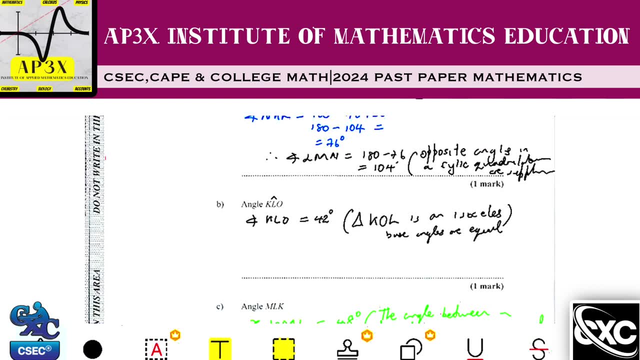 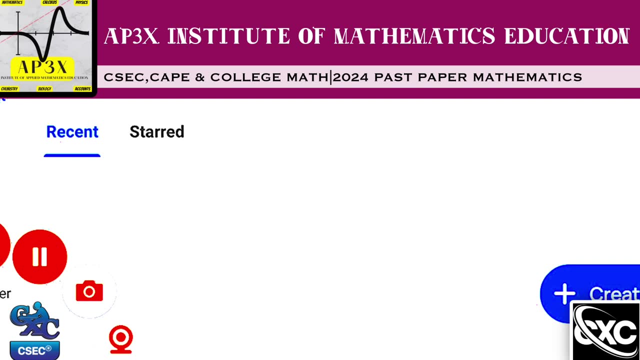 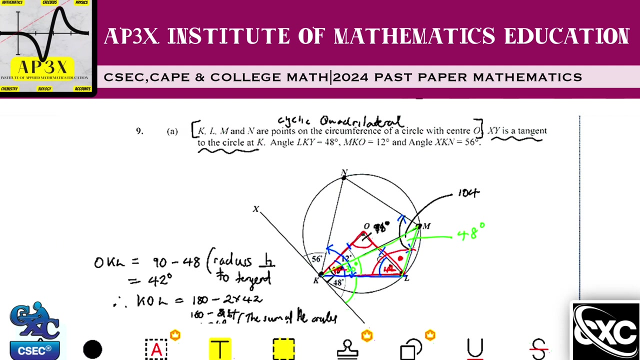 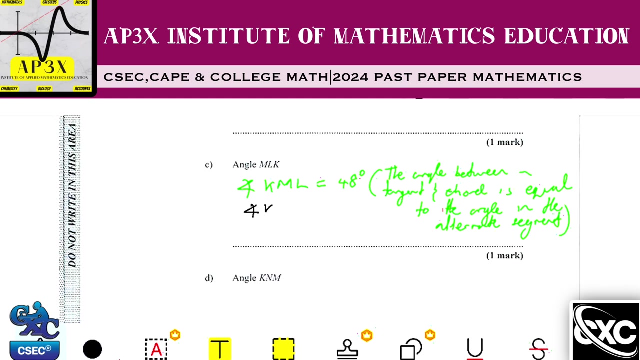 have so angle KLM okay so let's go here all right so angle KLM which is the angle we're looking for will be equal to 40 e plus 30 and take that from 180 so KLM is equal to 180 minus 48 plus 30. so that's 180 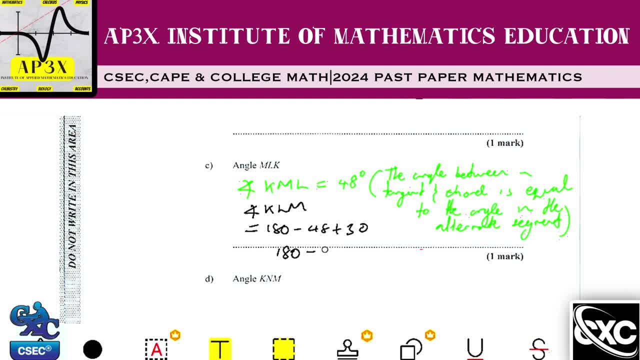 so that's 180 80 minus uh 78 and that's therefore equal to 102 degrees all right and that is because of the 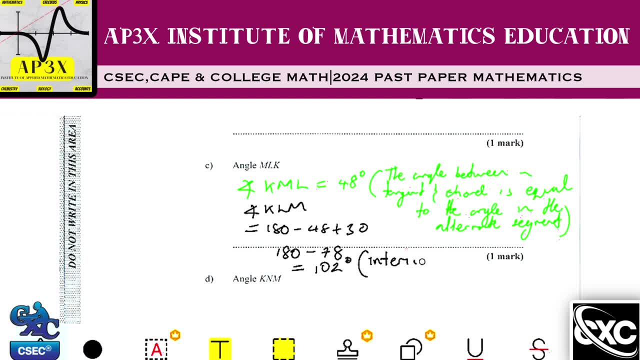 interior angles the interior angles of a triangle theorem so interior angles of a triangle are equal all right here we go guys all right so just bear with me here guys this new platform 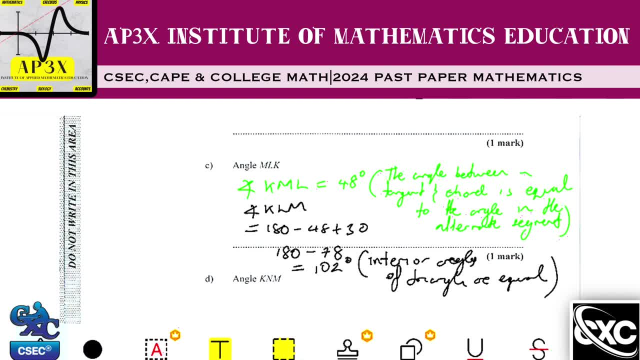 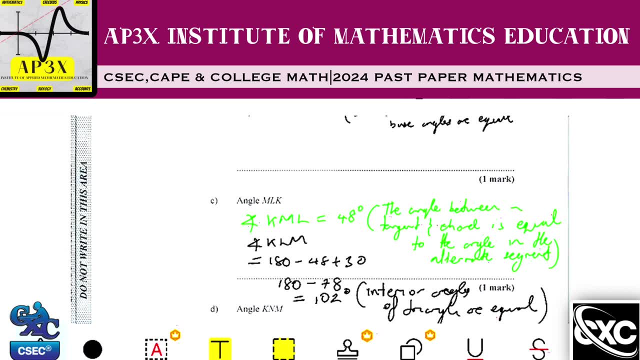 that i'm using to make the videos for you is a little bit challenging to navigate when i'm writing and i'm you know i don't have a lot of space i have to be scrolling up and down so forgive me if there's a little bit of pause during my explanation or a little bit of cut 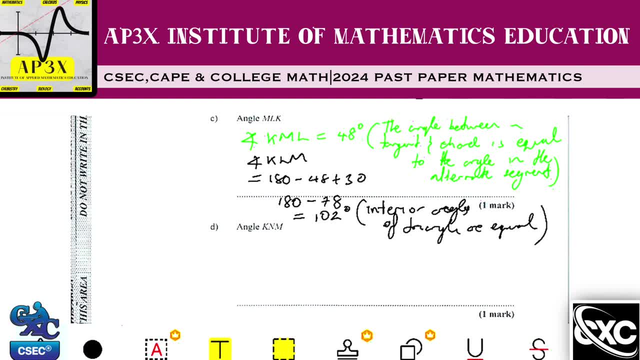 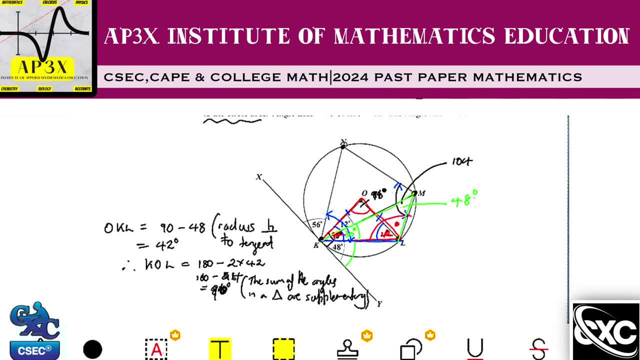 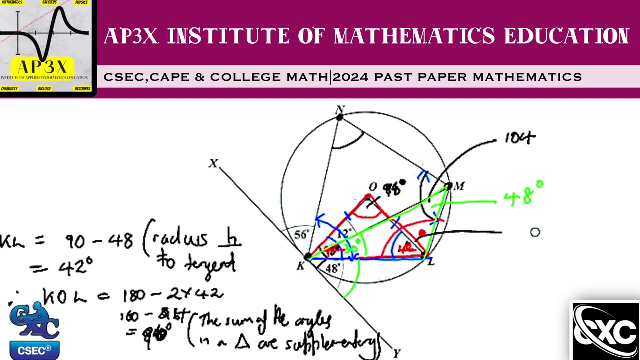 during my explanation all right just trying to make it as clear for you to follow now here say we're looking for k n m so let's go back up here k n m so let's look at k n m so that is k here n up here and m so looking for this angle here and that's easy because as we said earlier that the opposite angles in a cyclic quadrilateral are supplementary and we just found this angle here to be 100 and two degrees and it is directly opposite to the angle we're now searching for so we can just get straight to the point and say k n m 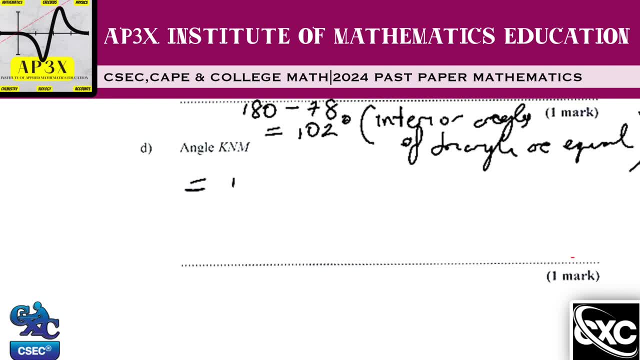 so angle k n m that's going to be equal to 180 minus 102 and that's equal to 78 degrees and the reason for that is that opposite angles in a 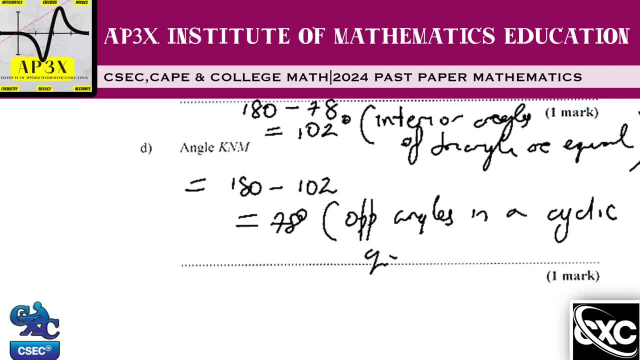 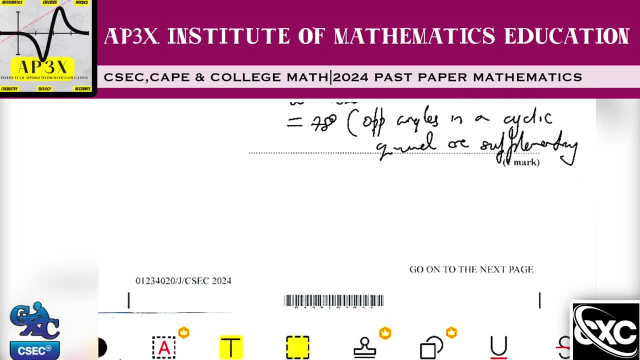 cyclic quad are supplementary all right hope i'm not over explaining myself all right my teaching style is based on the type of students that i do teach so a lot of the times my students are having to learn these concepts within a very short space of time so um this is how i have to get the 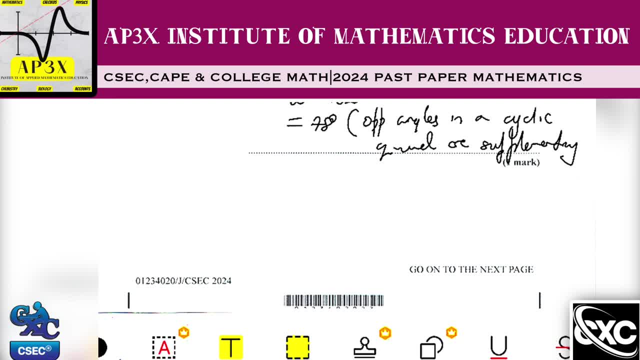 lesson across to you guys here who are watching this video so hopefully it's helpful and if it is again do not forget to leave your comments down below and hit the like button 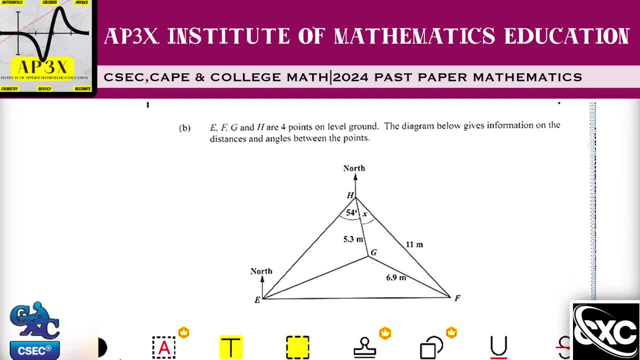 now we're going to be finally moving on then to the trig part of trigonometry here the whole 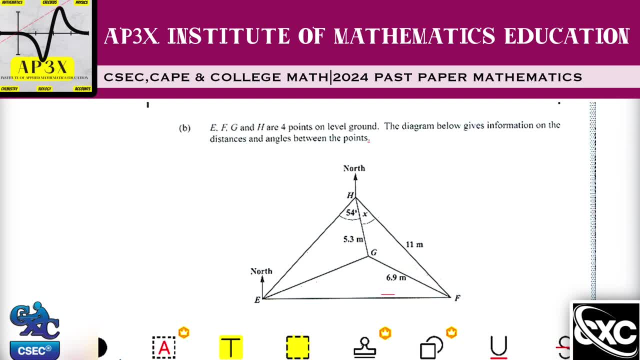 cosine sine and tangent ratio and all those fancy stuff so here now we're looking at e f g and h are four points on level ground e f g and h are four points on level ground okay noted the diagram below 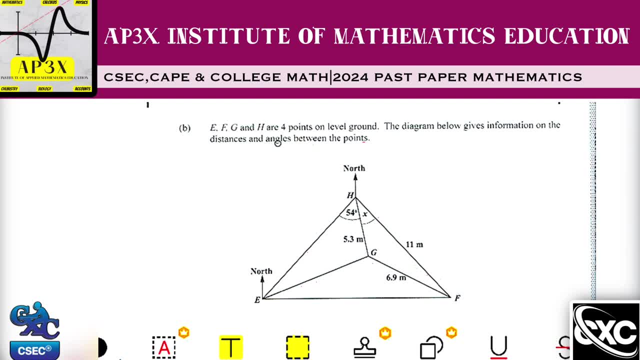 gives information on the distances and angles between the points so we're looking at say here this is a north line here that's a north line here we have 5.3 meters here we have an unknown angle here we have a side over here which is 11 we have 6.9 meters point f g h and e all right so 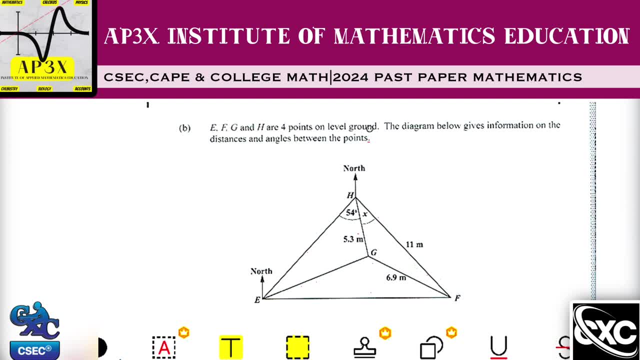 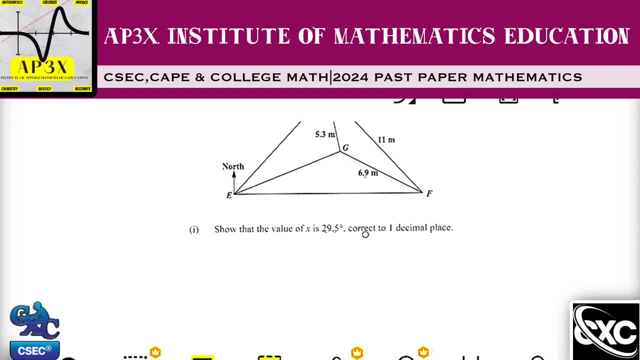 i've seen all of those all right there's not much clue given up here so let's scroll on and see what we want us to find we are to show that the value of x is 29.5 degrees corrected to one decimal place so we have to show that this angle is 29.1 29.5 degrees now in order for us to show that they're basically telling us that the angle is in fact 29.5 but we have to show how that answer 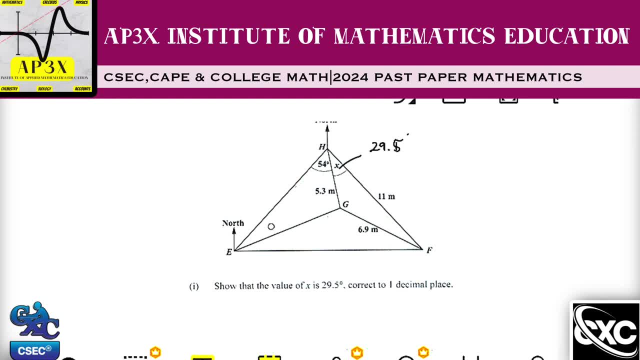 was derived now one of the things that i like to look for when i see trig the very first thing that my brain tells me is that i need to look to see if i see any potential right angle triangles 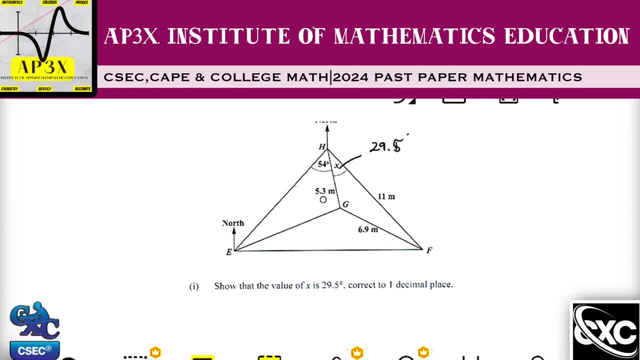 if i see any right angle triangles already i know that i may have to be deciphering between the cosine the trig ratios which is sine cosine and tangent or i need to be looking at pythagorean theorem if i don't see any possible right angle triangles then it means then i'm going to be 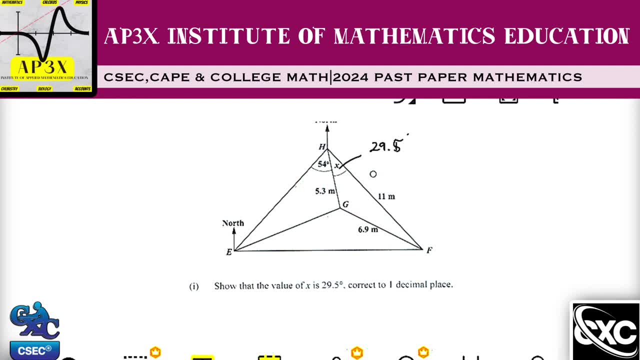 thinking about two formulas which is sine and cosine rule again a link will be pinned in the description of this video to where you can find it and i'm going to show you how to do that 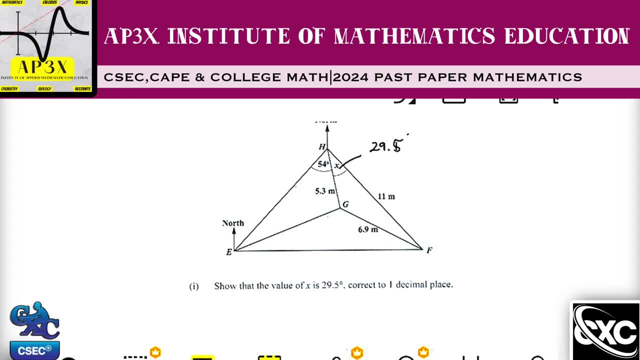 how to apply the sine and cosine rule which was done a few months on my few months ago on my channel so now i don't see any right angle triangles now i'm guessing that maybe i need 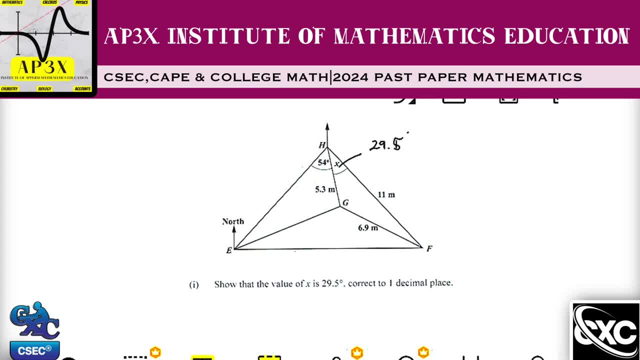 to use the cosine or the sine rule now when i observe this triangle over here as i'm going to be zooming up for you now say here i realize that this x here that i'm looking for is in fact in a 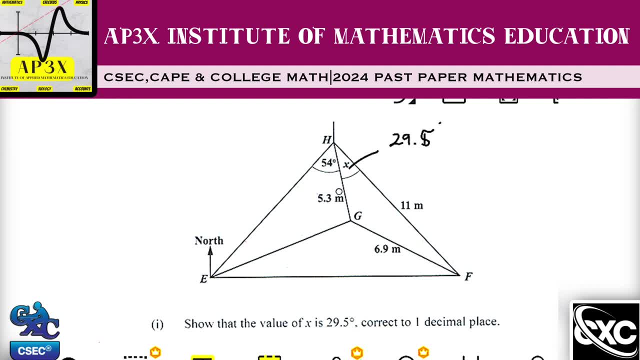 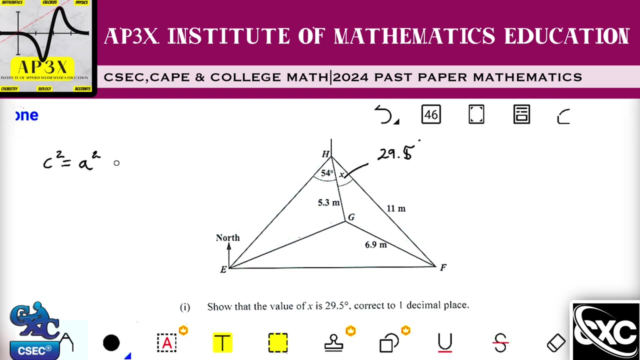 triangle that is non-right evidence of any 90 degree here now the cosine rule is applied to the cosine and cosine rule which is sine cosine and cosine rule which is sine cosine and cosine rule here because we use the cosine rule in two different scenarios when we are given an angle between two sides or when we are given all three sides now already i know that the cosine rule is in fact c squared is equal to a squared plus b squared minus 2ab multiplied by the cosine of the 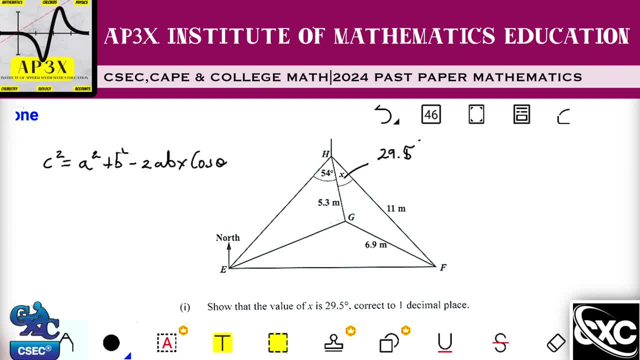 angle that we're in fact looking for again you can check out the tutorial video on my channel about how to apply this formula 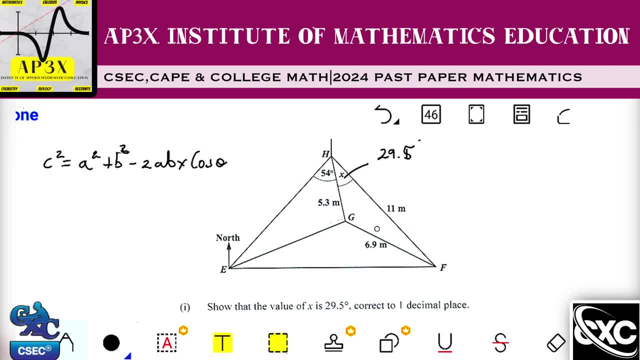 so c squared is in fact going to be the side that is facing the angle we're looking for so in this case here my c is going to be 6.9 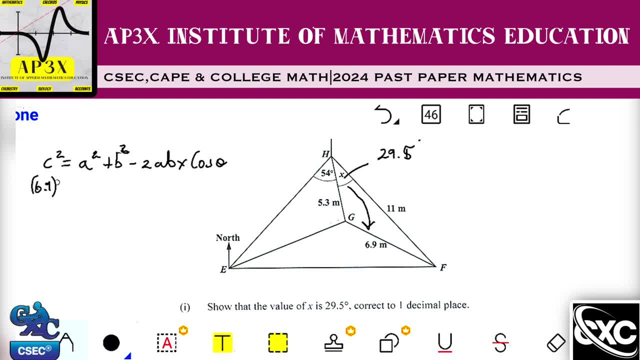 so that's 6.9 squared a and b are going to be the other two sides respectively so that's 5.3 squared plus 11 squared minus 2 times 5.3 times 11 squared so c squared is in fact going to be the side that is facing the angle we're looking for 11 and obviously multiplied by the cosine of the angle which we do not know in this case so let's grab our calculators out 6.9 squared is in fact 47.61 and that's going to be equal to 5.3 squared that works out to be 28.09 and 11 squared is 121 and that's going to be subtracted we're going to subtract 2 times 5.3 times 11 that works out to be 116.6 cosine theta that's joined onto it so 47.61 will be equal to when i add 28 to 1 28.9 28.01 and that's going to be 11 squared times 5.3 squared that works out to be 116.6 and that's going to be subtracted we're going to subtract 2 times 5.3 times 11 that works out to be 116.6 and that's going to be 0.09 pardon me 28.09 to 100 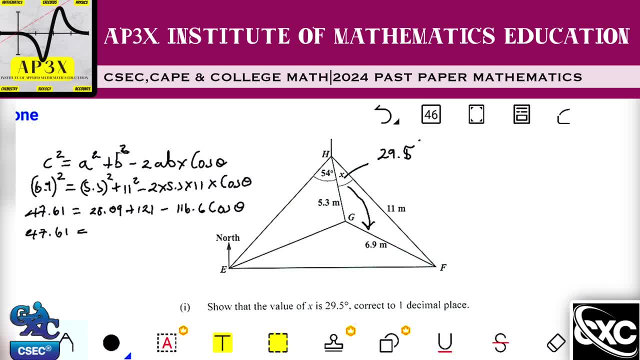 and Tesla out 19 I'm gonna add those together now I'm gonna get 149 and 10 9 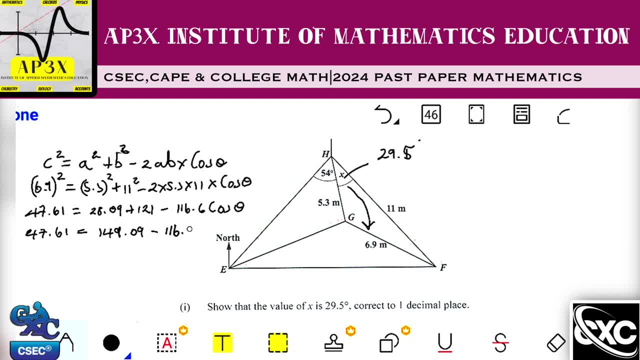 I'm gonna subtract 116 point-six cosine theta now the objective is to get cosign force and t to the be positive so therefore if we can have democratic 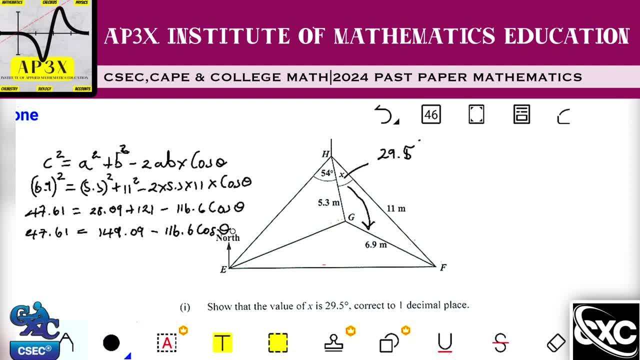 So therefore, then I'm going to transpose the negative 116.6 cosine theta to my left because I need my cosine theta to have a positive sign in front of it. 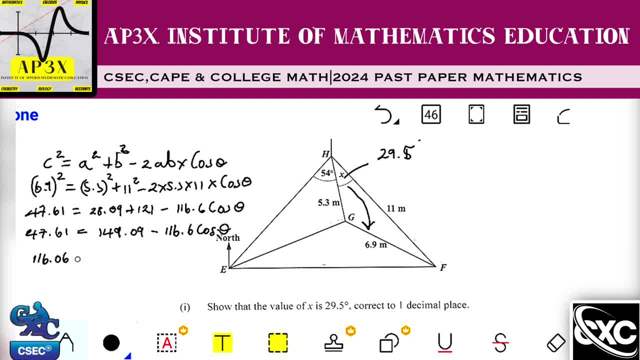 So I'm going to have 116.06 cosine theta. Remember that these two numbers are attached. 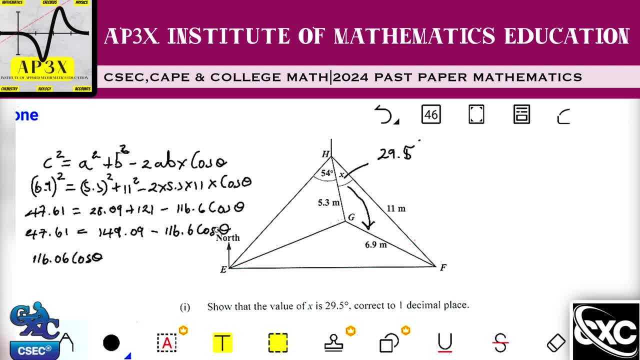 These two, this constant here and this variable here, cosine theta, they're attached. And so therefore, bringing that to the left forces me to bring the 47.61 to my right. 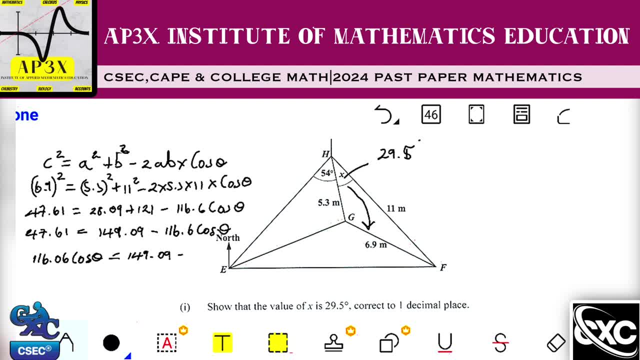 So that's 149.09 subtract, say here, 47.61. 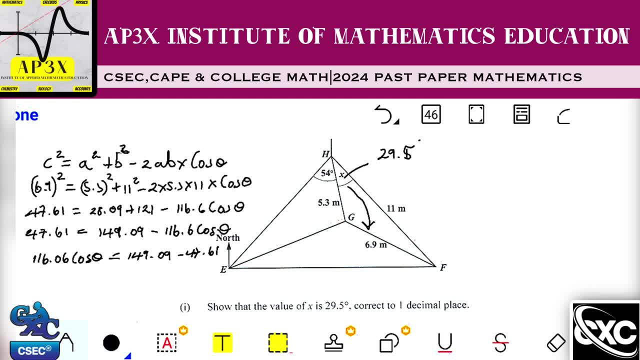 So subtracting then 149.09 minus, say here, 47.61, that works out to be 101.48. 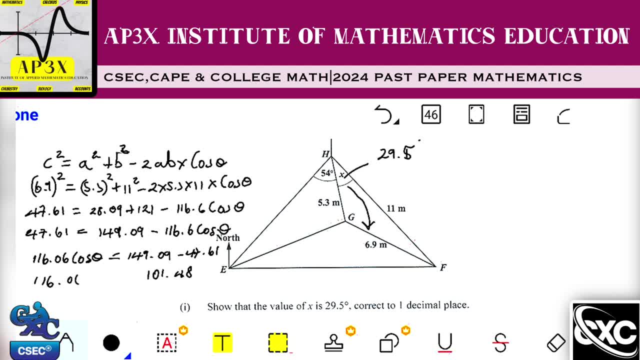 And that's going to be equal to then 116.06. So that's going to be 116.06 cosine theta. 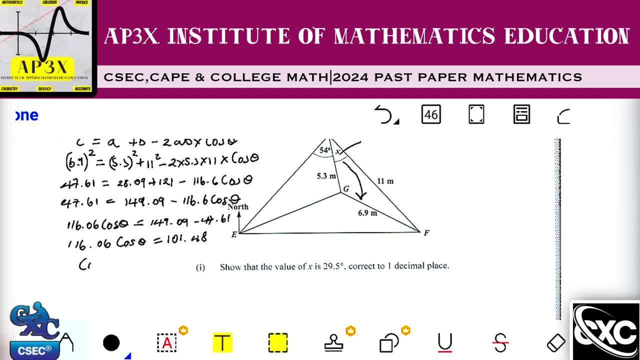 Now I need to isolate cosine theta by dividing both sides of the equation by 116.06. So that's going to be 101.48 divided by 116.06. 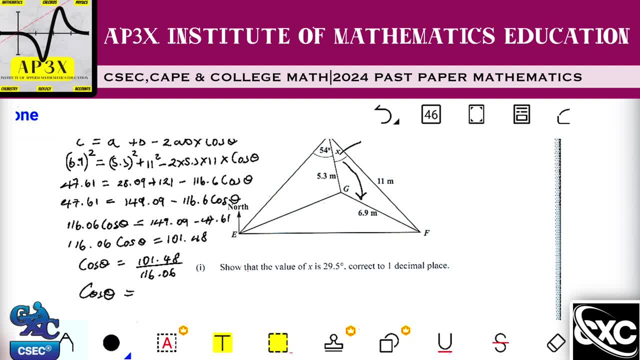 And so cosine theta then works out to be 101.48 divided by 116.06. 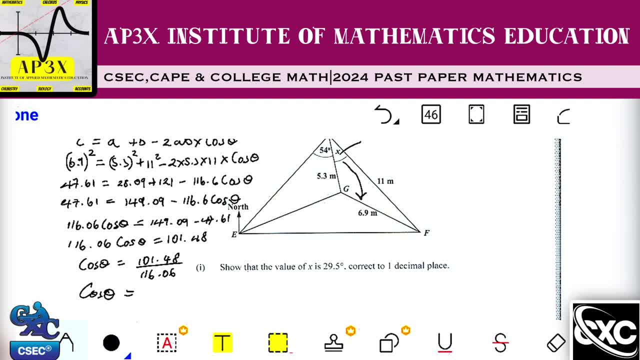 And that gives me an answer here of 0.874. 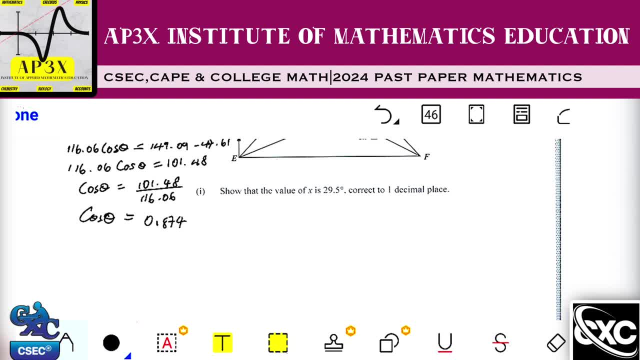 Now if you go on your calculator as you're watching this video and you press the shift button or the second function button that you can find at the top left-hand corner of your calculator, and then you press the cos, you should see cos raised to the minus 1 coming up. 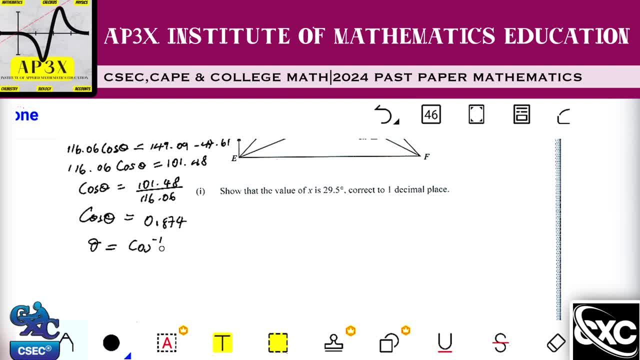 So theta then is equal to cosine raised to the minus 1. Of the value that you're looking at here. 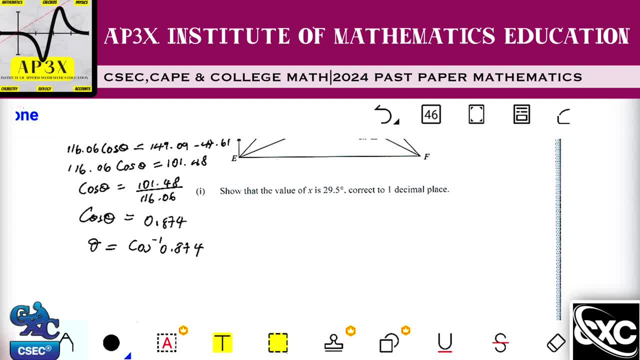 And if we have done our calculations correctly, it should show that the answer is 29.5. So that is shift cosine 0.874. 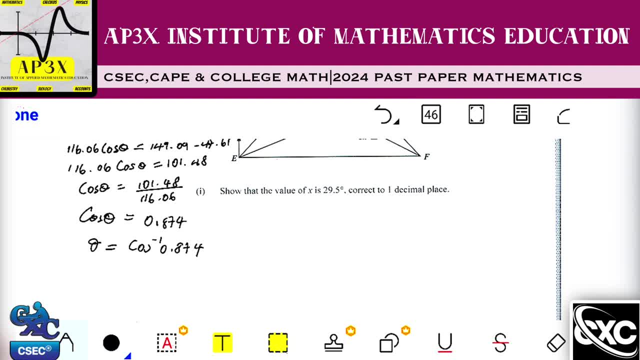 And if you get 29.07 or thereabout, then of course, you see, round it off. They said that theta here is equal to, well, on my calculator, it's telling me that it is 29.07. 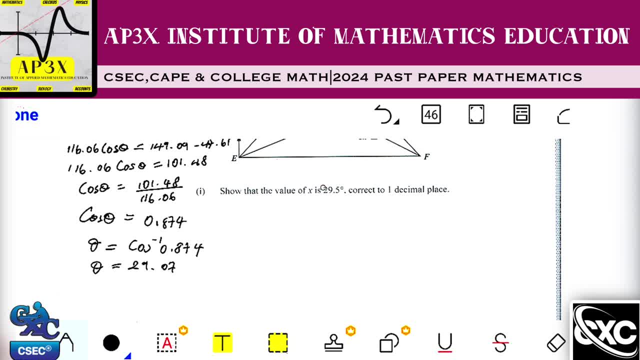 All right. So it is very, very close to 29.5. 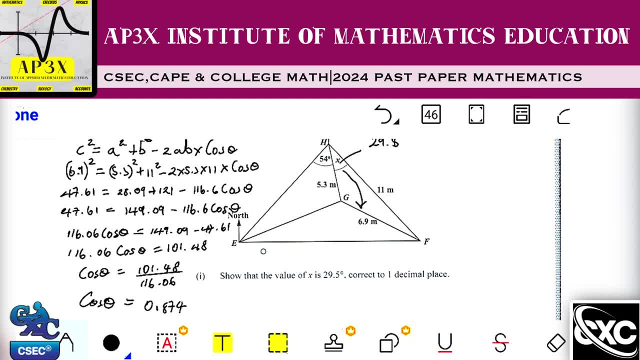 I'm not sure why I'm not getting the exact value as requested, but it could be a case where maybe I needed more decimal places here. 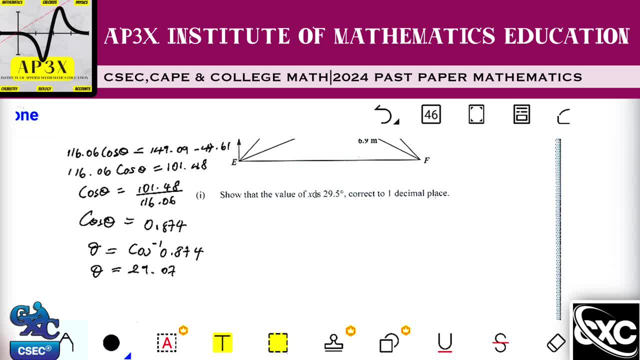 So it could be anything really, but it's very, very close to the answer requested by C6. It's within a range. So this would be an acceptable estimation for the angle. So that we have proven there. All right. 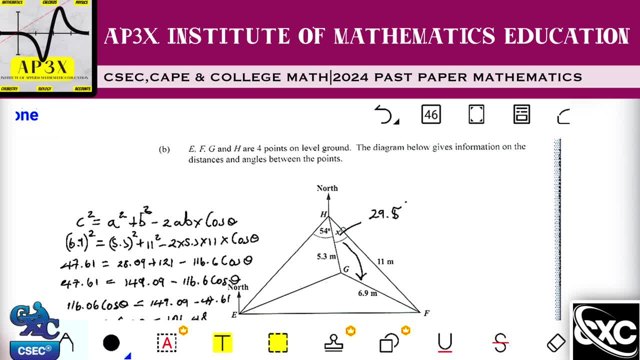 So let's put. That information here on the diagram. We know that X is in fact 29. See here, five. 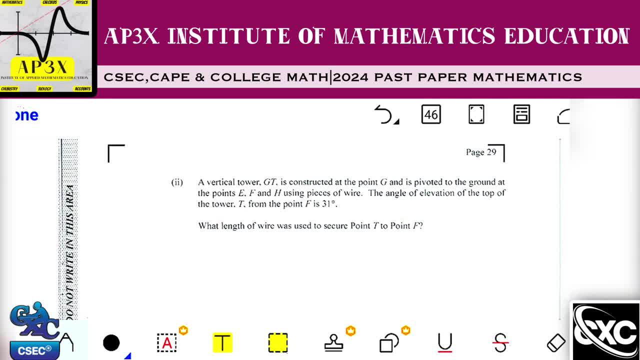 Now we're going to go down to this section then of the paper. And it says that a vertical tower, G, G, T, a vertical tower. Normally, when you see that word vertical, you know right away that a 90 degree is going to be involved. So vertical tower G, T is constructed at the point G. And is pivoted to the ground. 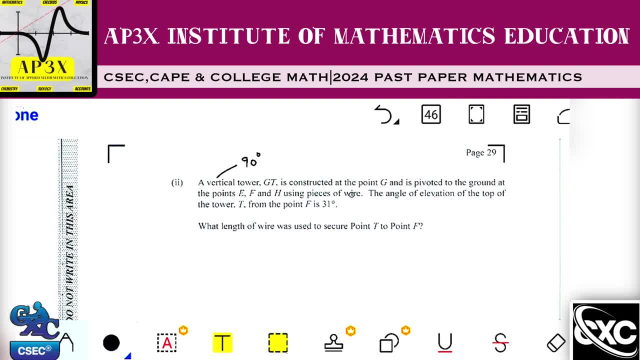 At the points E, F, and H, using pipes, pieces of wires. Let's just look at that first of all. 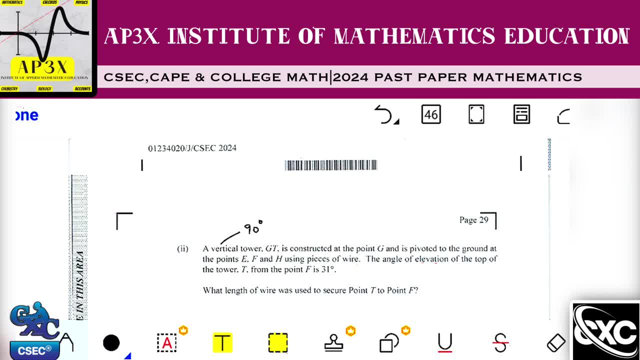 So it says that a vertical tower, G, T, is constructed at the point G. So vertical tower, G, T, vertical tower. 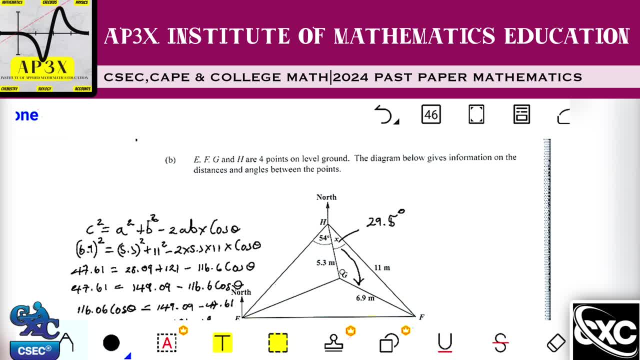 So right away then, I'm looking at from the point G, a vertical tower has been constructed. Let me just remove this 29.8 to get a visual of this. 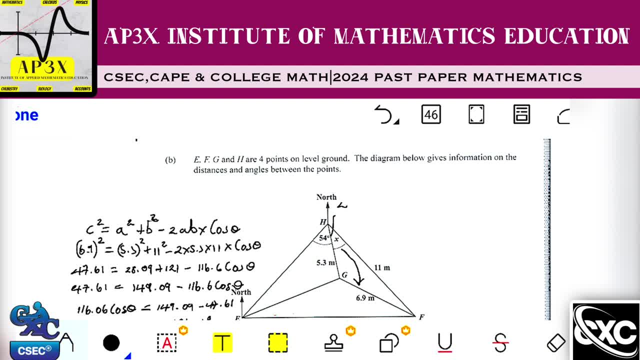 So this is 29.5 degrees. So this is a vertical tower. 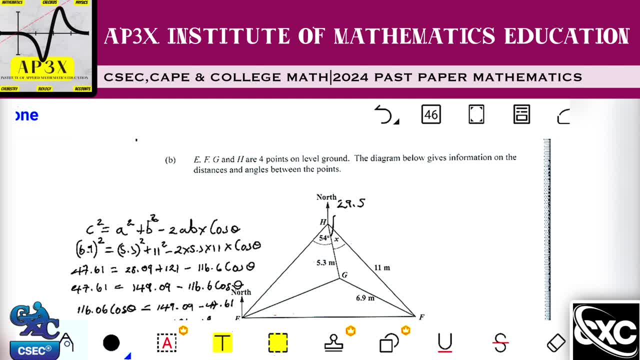 What we're looking at then is in fact, see here, let me just use a different color. A vertical tower. We're looking at saying draw a straight line up like that. All right. So that's the vertical tower G, T. 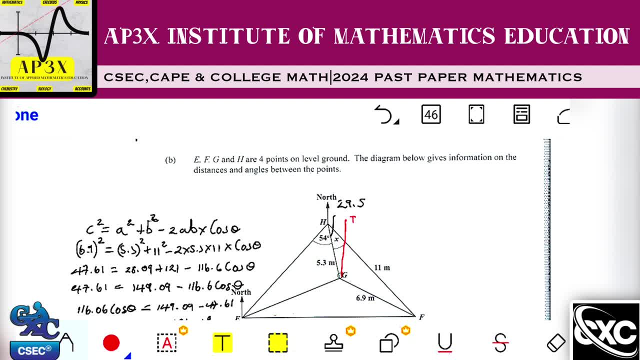 So T will obviously be in here. So that's a vertical tower that's constructed at G. 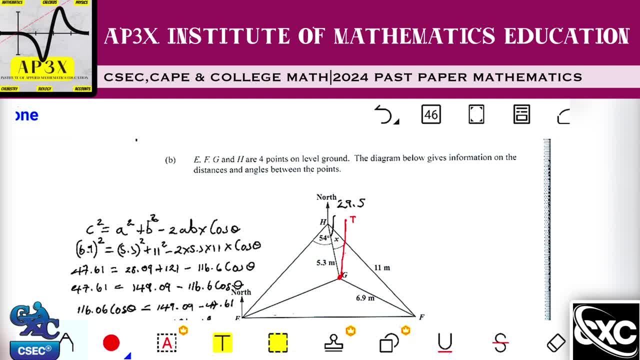 All right. So that's the vertical tower. 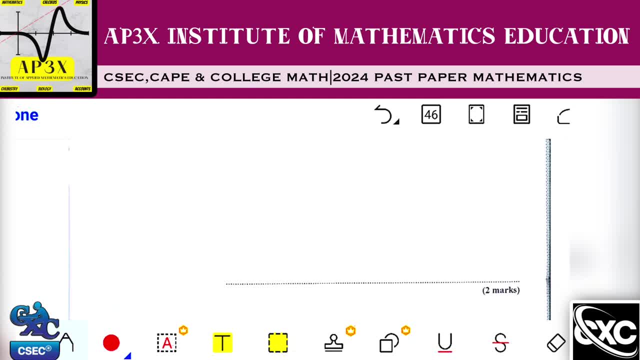 And then it went on to say something that, let's see here, guys, constructed at the point G. And it's pivoted to the ground at the points E, F, and H. E, F, and H. So E, F, and H. So it is pivoted. 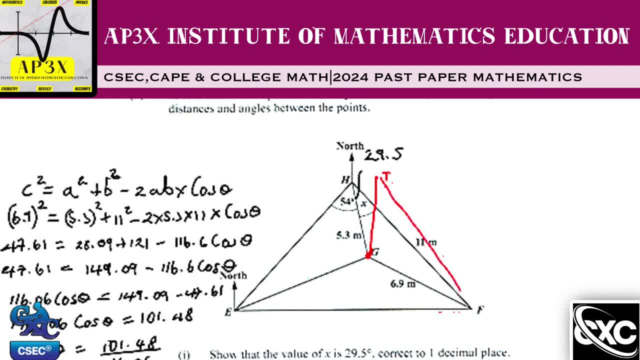 So what we're looking at then is that a line basically connects this to this. And we know that it's a vertical. 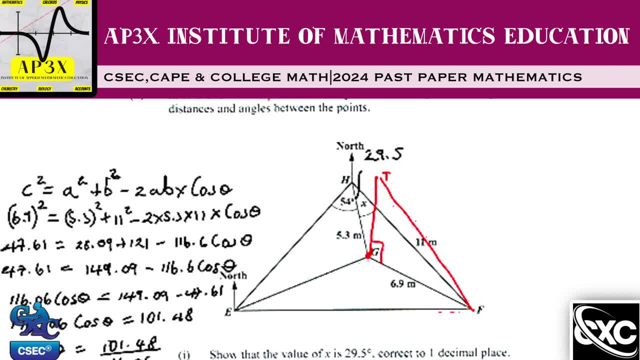 So we know right away that that angle there is 90 degrees. And it's pivoted to the ground. So basically, we're looking at a right angle triangle being constructed on this platform here. 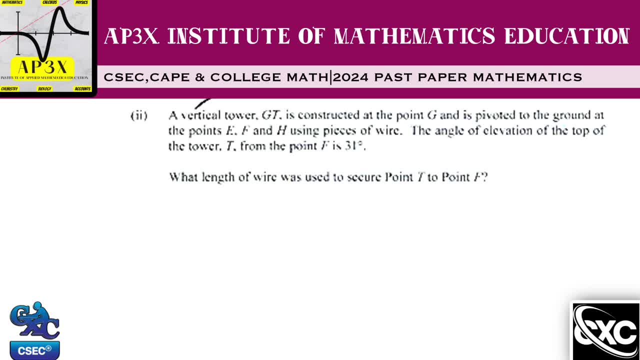 So let's just take this out here. Let's just take this diagram then. 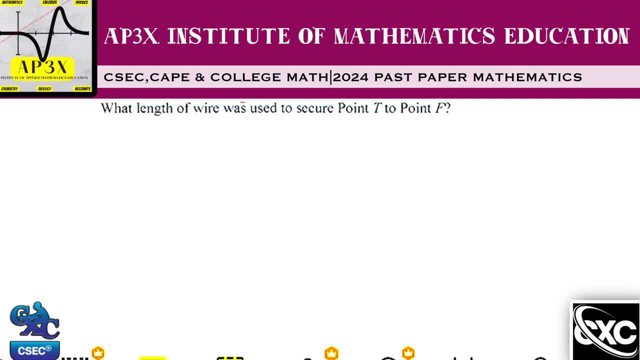 Because what helps is that once you can interpret the question, then you can draw your separate diagrams to help you. 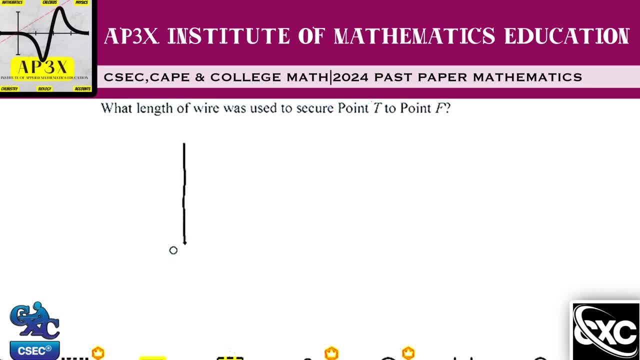 So we're looking at, say here, this vertical tower that was constructed. It's pivoted at G, and then it was connected, then, say here, to F, all the way down here. And we know that this is 90. 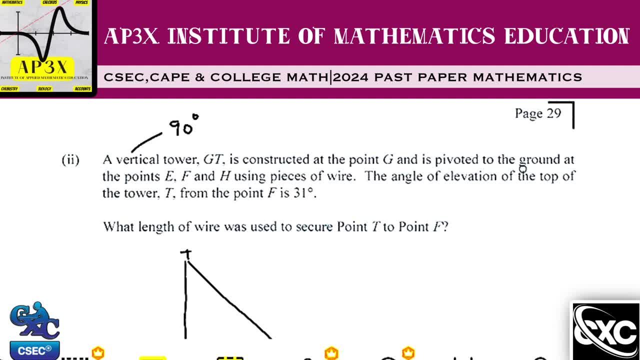 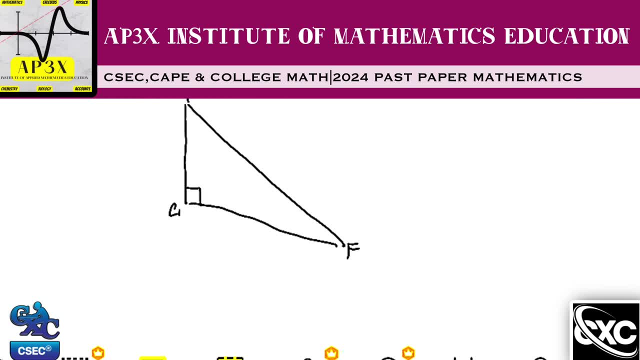 Let's see what it then goes on to say. It says that the angle of elevation of the top of the tower T from the point F is 31. So from F, this is 31 degrees. So the elevation angle is the angle looking up at T, and that is 31. All right. 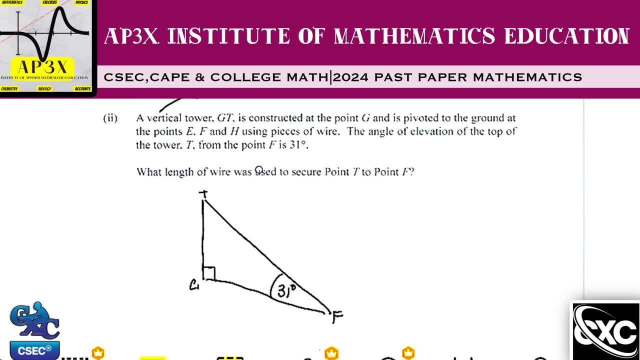 And let's see what other information was given to us here. It says, what is the length of the wire? What length of wire was used to secure the point T to F? So we're looking for this side here. That is X. 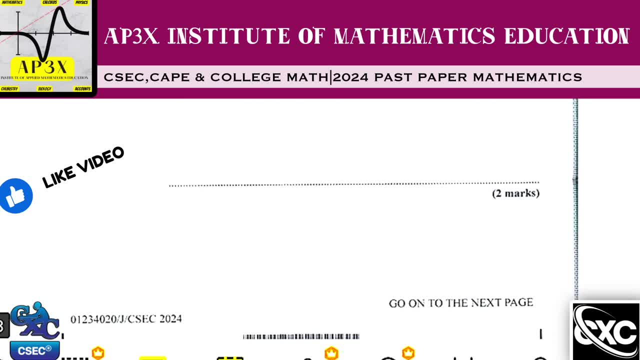 All right. So we only have an angle and an unknown side. Let's look back at our main diagram to see what other information is up there. Vertical tower GT. So. Okay, GT. So could it be this? All right. 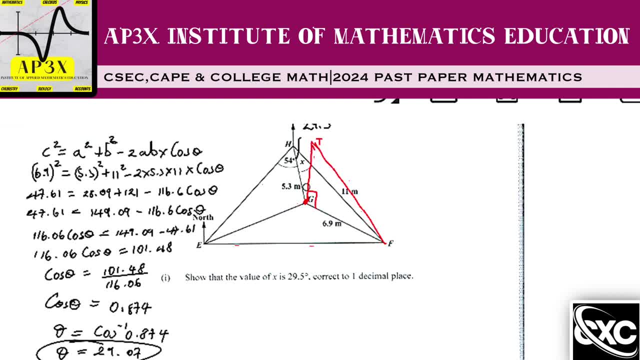 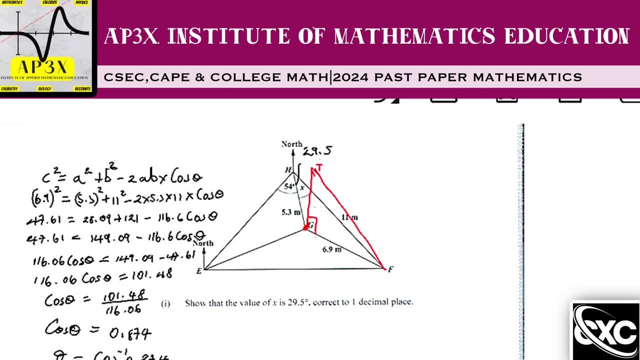 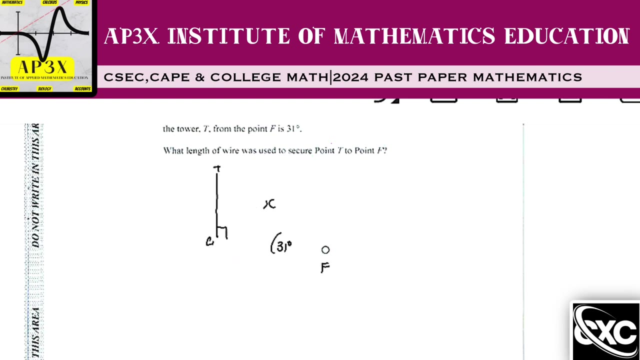 So I think what we're looking at here is the base of the triangle is actually 6.9, because the vertical tower was connected from G and then connected to F. So already we know that, say here, GF is 6.9. Not sure how that missed me, but just kind of rereading the question here, so we know that right here is, in fact, 6.9. All right. 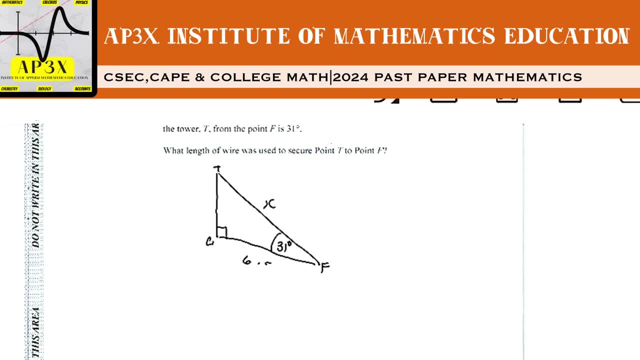 So therefore then, this is 6.9. So therefore then we can go ahead and use the, that's the hypotenuse. This is the angle, so that is my opposite. This is my adjacent here. So therefore I can use the cosine ratio here. So cosine theta is equal to adjacent divided by hypotenuse. All right. Because that's my hypotenuse. This is my adjacent. 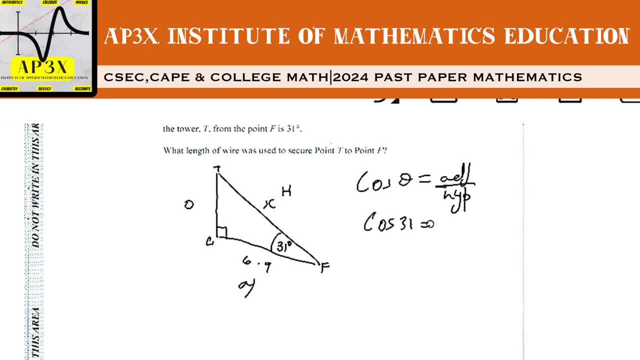 So the cosine of 31 degrees is equal to the adjacent, say here, is 6.9. 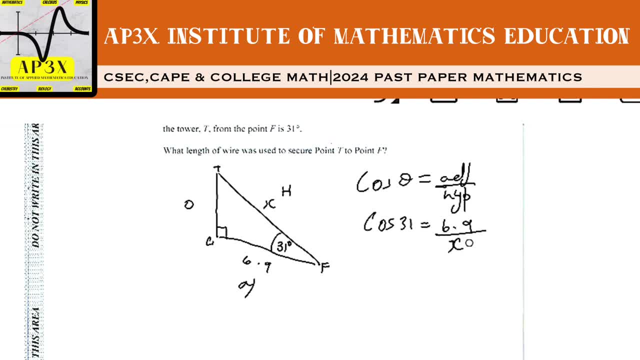 And the hypotenuse is, in fact, what we're looking for, which is X. In this case here. 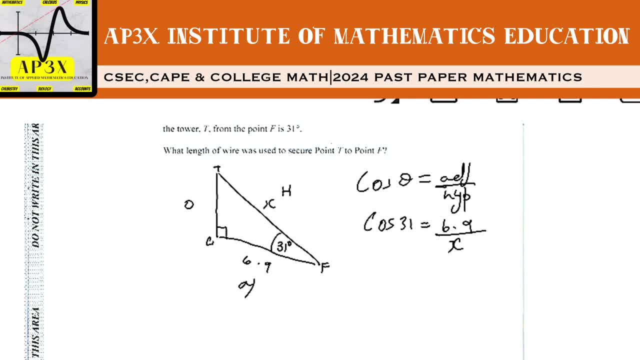 So the cosine of 31, that is 0.5, 0.857, 0.857, and that's equal to 6.9 divided by X. When the unknown is at the bottom of the equation, we can therefore just take the X and put it up here and have the 6.9 being divided then by the 0.857. So we say 6.9 divided by 8 point, pardon me, 6.9 divided by 0.857, and it would end up with a result here of 8 centimeter, 8 meters, 8.05 to be precise. 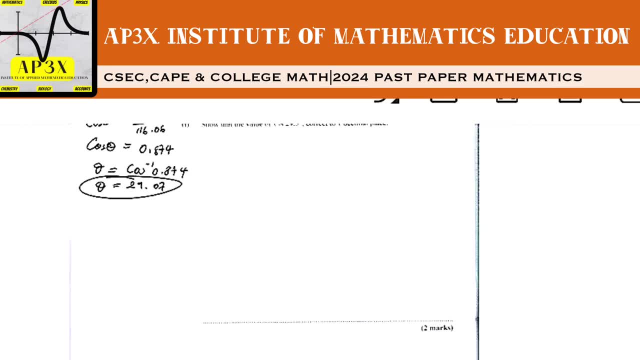 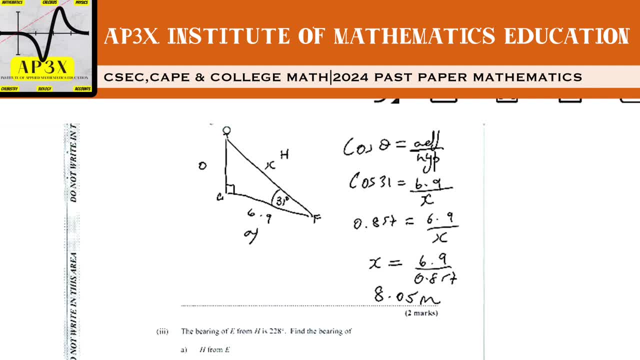 That is how you find the length of the wire that connects the top of the pole, the top of the vertical pole, GT, to F, okay? 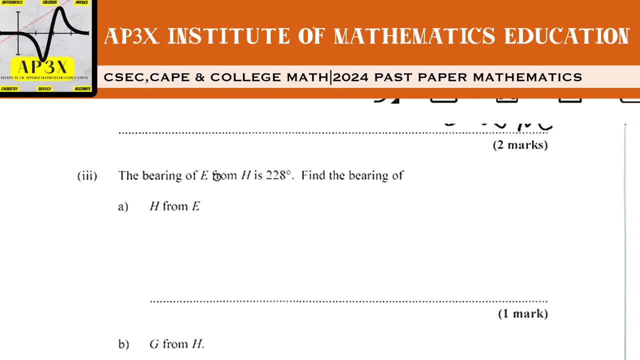 Now we're then looking for finding the bearings of E from F, the bearing of E from F. 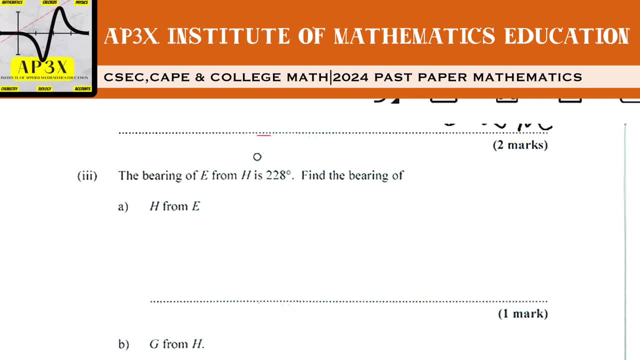 Remember that a bearing is measured in a clockwise direction, so we need to start from the start, we need to draw up, we need to draw a north line at H, and then bend, follow the angle in a clockwise direction until we meet at the line leading us to E. 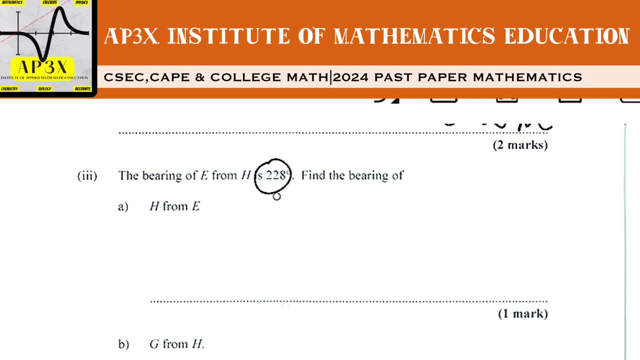 Now, it seems as if they have given us the bearing, okay? So they, in fact, has, they have told us here that the bearing of E from H is 228. I initially thought that they were asking us to calculate it. So they are telling us that it is 228. Then we are required to find the bearing of F. H from E. 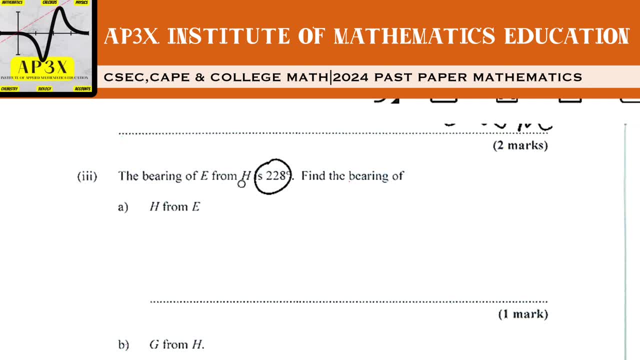 So they give us the bearing of E from H, but we are to find the bearing of H from E. So let's go on our diagram then. So we know that E from H is 228. 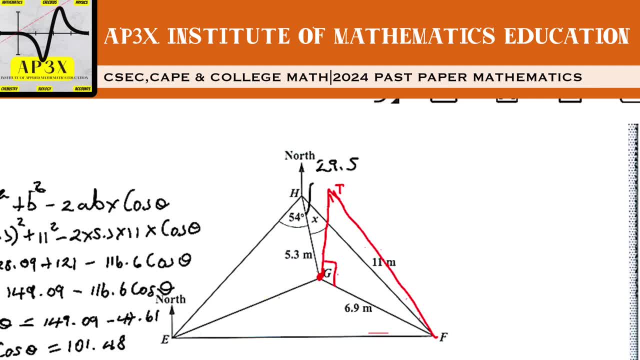 So E from H, let's go ahead then and kind of just clear this up a little bit. 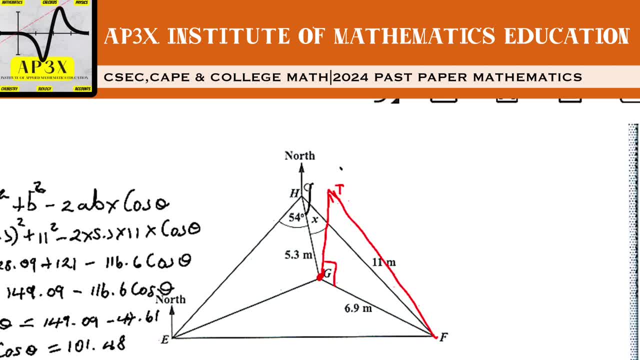 E from H, so I'm going to need some sort of north line here to help me. So E from H then. 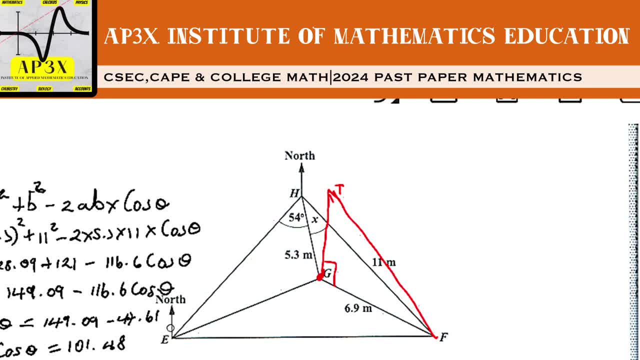 So where we have E, where is E? This is E here from H. So this is my north line. 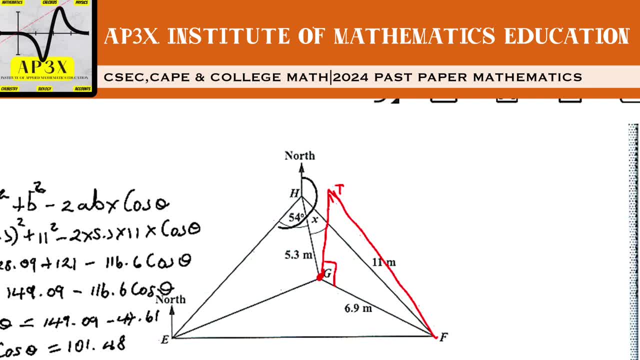 So come around like that, all the way around here. That's going to be 228. That's what they're saying. All right. That is 28. 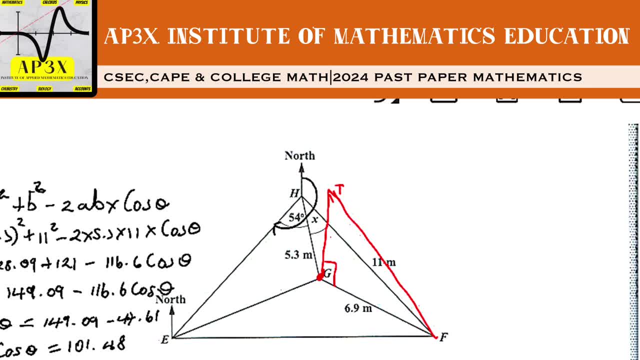 All right. So if that is 228, our requirement then is to, in fact, find the bearing of H from H. So H from E, so H from E, so north line here, H from E, so H from E. We need this outside angle right here. That's the bearing that we're looking for. 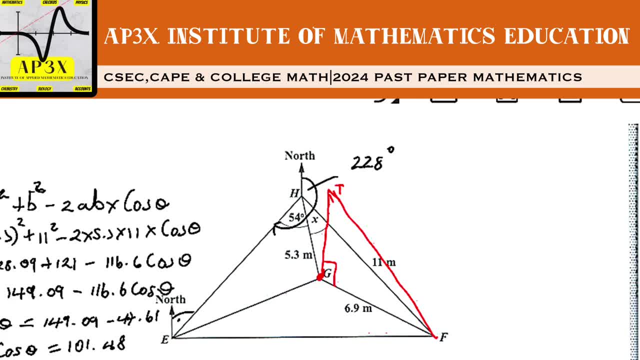 Now, this is a little tricky. So you guys have to pay very close attention to what I'm going to demonstrate here. And I don't have a lot of space, guys. 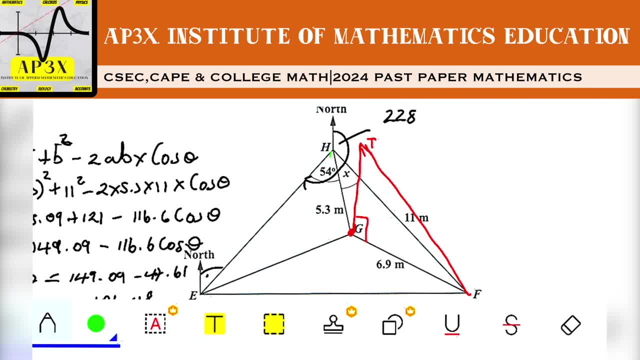 Now, since this is a north line, if I were to extend, say, here, a line, an auxiliary line, I'm going to have to extend, say, here, a line, an auxiliary line, I'm going to extend, say, here, a line, an auxiliary line, and call it my south line, then already I know that whatever this angle is from the south to here is going to be equal to, say, here, the angle down here because of the alternate angle principle. 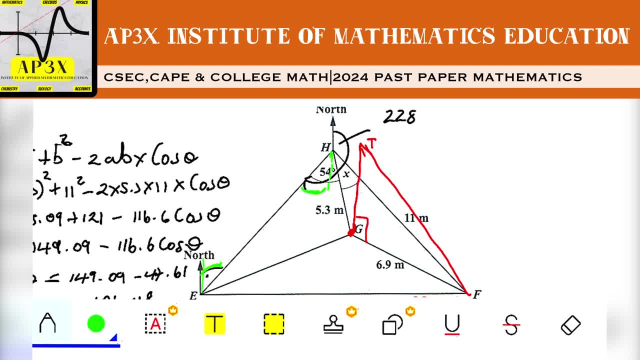 When north and south is parallel, then you're looking at forming a Z angle. 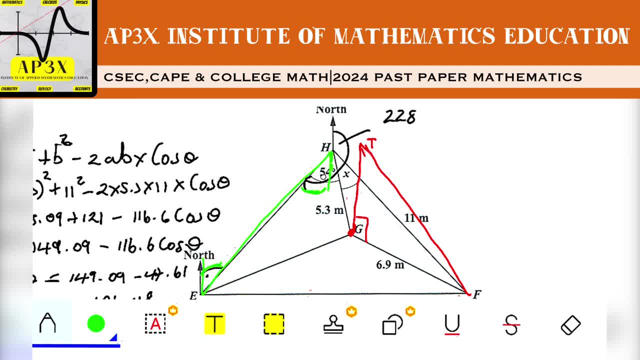 So right here is going to be equal to right here. Now, please note that the 54 is, in fact, what we want and a little tiny piece over here. All right? 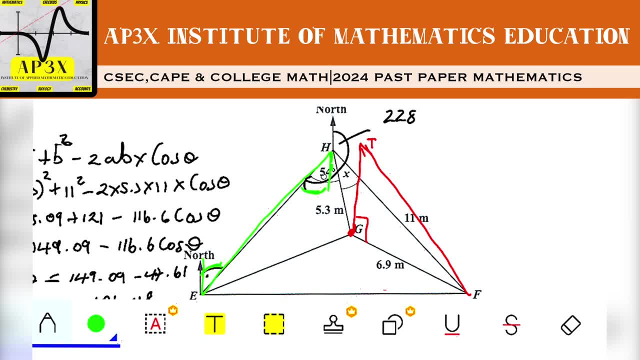 So that 54 can be a little bit tricky. It might be misled to think that the angle down here is 54. 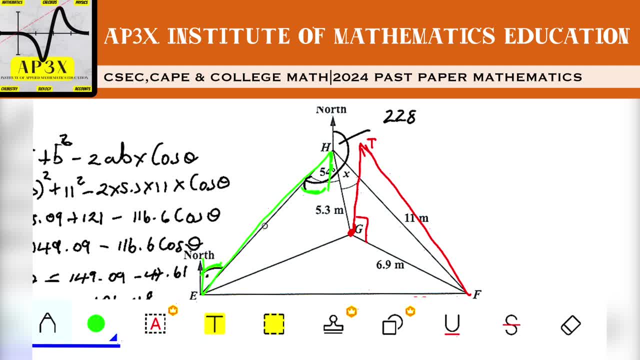 Now, to find this angle inside the Z here, this Z that I've drawn with my green line, to find this angle, I know that the complete angle is 228. And I know that from north to south is 180. 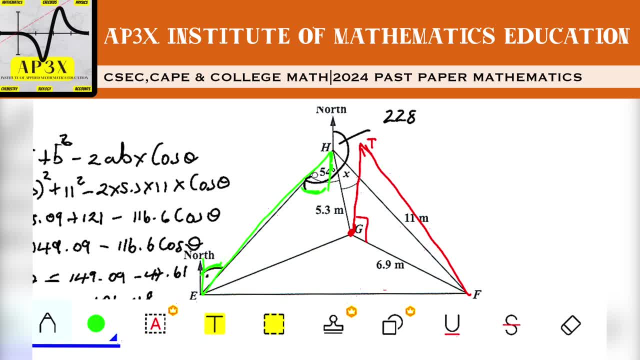 So this piece of angle in here is going to be 228. Minus 180. 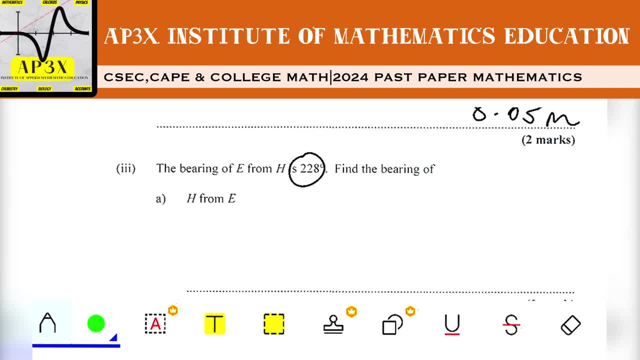 So if you go down here and we write that in that angle, then let's give it a name. This is S here. 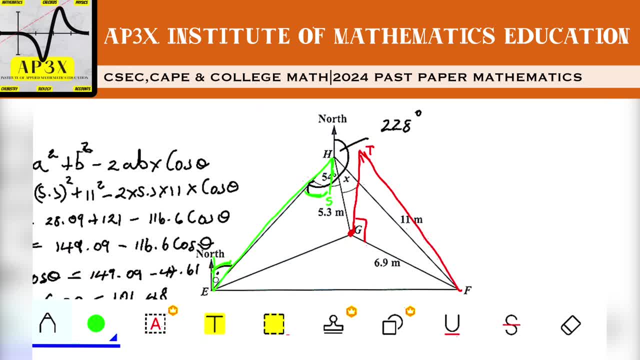 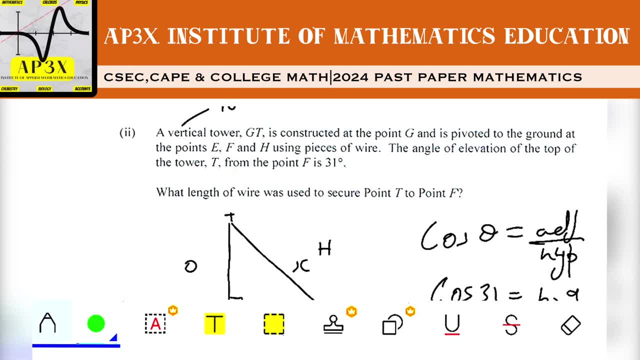 So I know that this angle that I'm looking for is, in fact, EHS. So EHS. So angle EHS. 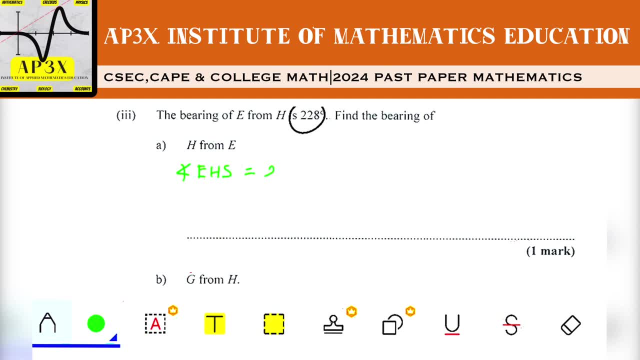 EHS is equal to 228 minus the degree from north to south. And then, therefore, then that works out to be 48 degrees. 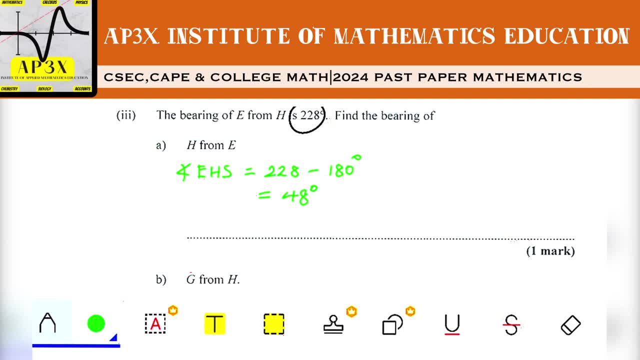 So that angle in that little section of the diagram there is, in fact, 48. 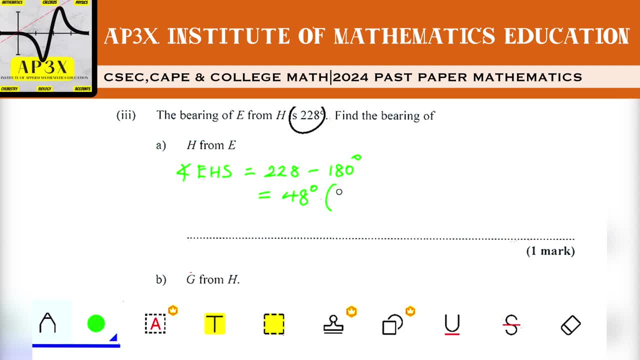 And that is as a result of, say here, angles at a point on a straight line measures 180. All right? So I don't think I need to write a statement for that one. 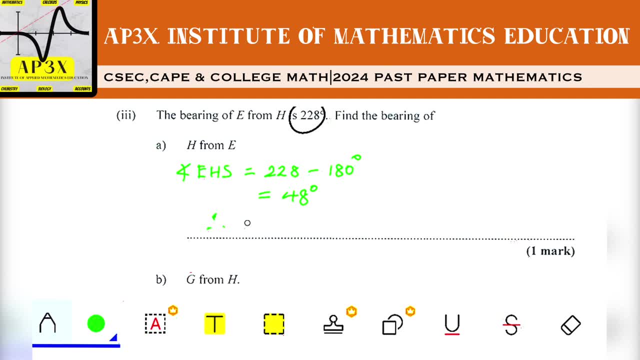 So I can, therefore, then conclude that the bearing, so H from E is, in fact, equal to 48 degrees. And that is as a result of the angles being alternate. So alternate angles are equal. 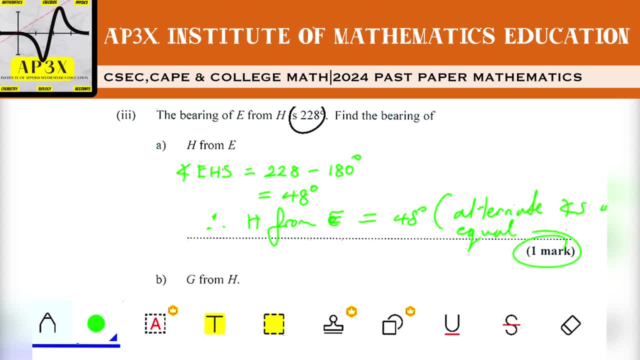 Again, 6 is a little bit stingy on the marks there. I thought that was a lot of thinking for just one mark, but it is what it is. 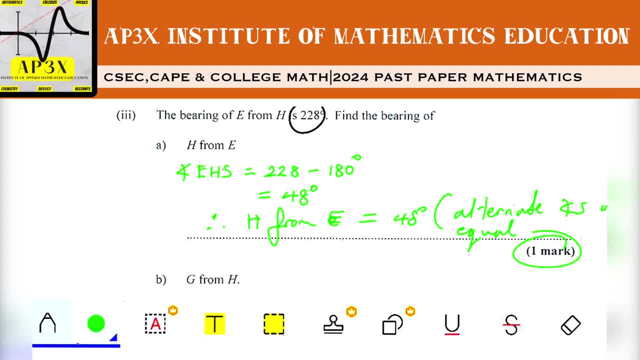 It's one mark. So that's what we have to do to calculate that angle in here. 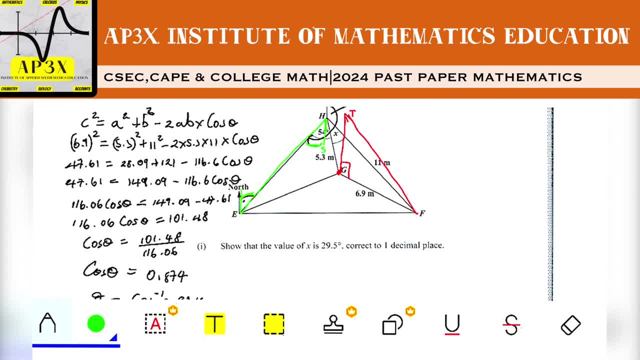 So let's go on our main diagram now and then write in that 48 degrees here. So this is, in fact, over here, 48. 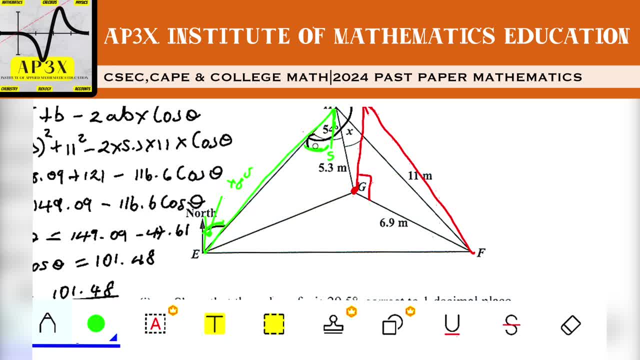 And then, therefore, then this angle inside here is, in fact, also 48 degrees. So right away now, if I need to find this, I can just take 48 away from 54. Or if I need to find it later on, that little piece right in here. Right here. Okay? So let's hold on. 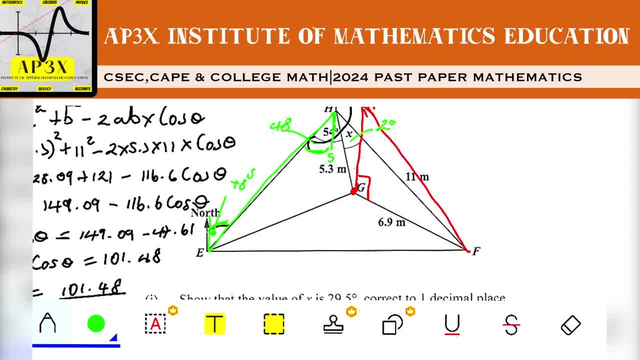 Let's see if we're going to need that. Remember that this X already we've proven is, in fact, 29.5 degrees. 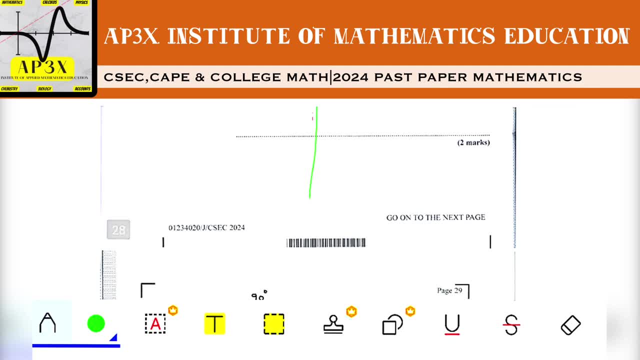 All right. So that is the bearing of H from E. 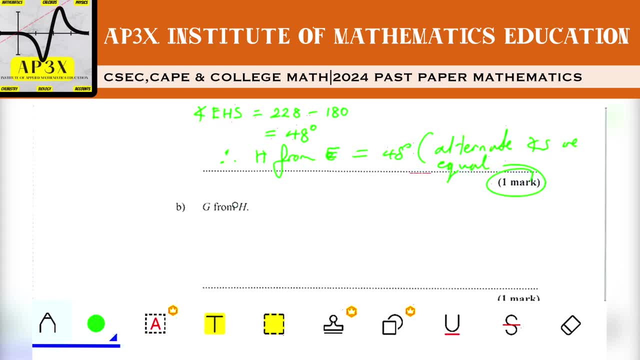 Now we're looking at the bearing of G from H. So G from H. Now we need to draw our north line at H and head towards G. So G from H. 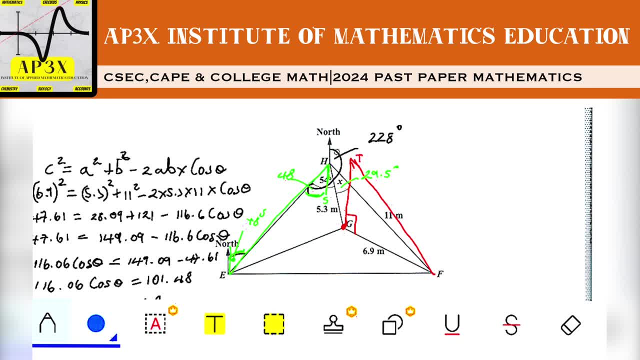 So from H, again, now we already have our north line, but then we're going around to G. 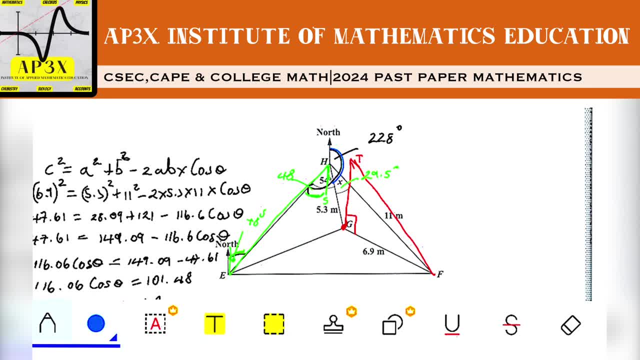 So looking from H to G here. This is that part right there. All right? 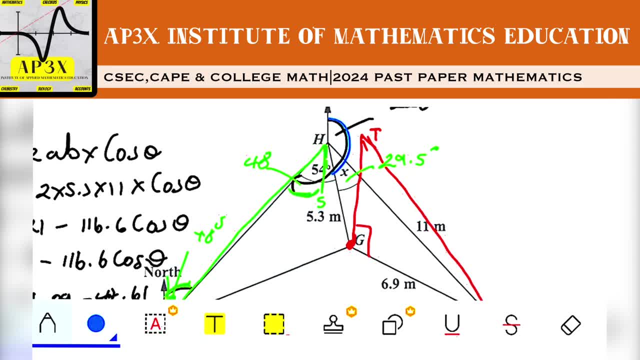 That is inclusive of that 29 degrees, 29.5 degrees. Now, how can we do this? 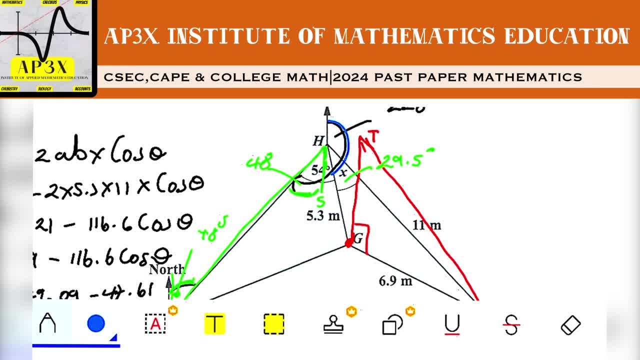 We know already that from here to here includes our 29.5. So we don't know the full angle coming around from north to this position here, G. 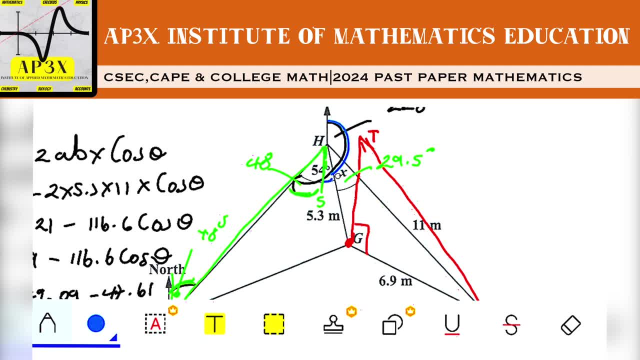 Now, as I said, we don't know the full angle. As I said, this angle in here might be very useful. 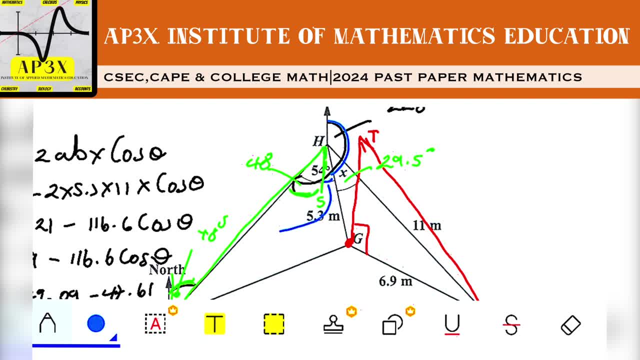 So this piece of angle, hopefully you guys are following. That little piece right in here is, in fact, going to be 100. 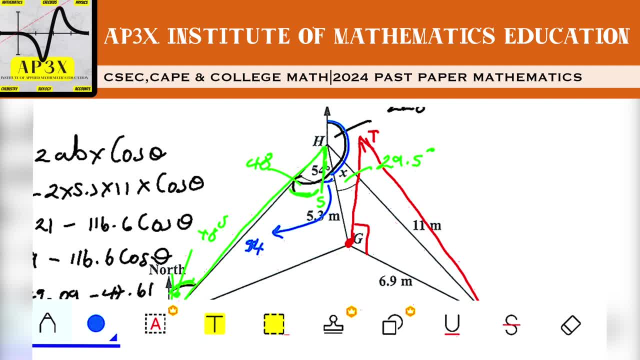 And sorry, it's going to be actually 54 minus the 48 that we just calculated here. That's 48. 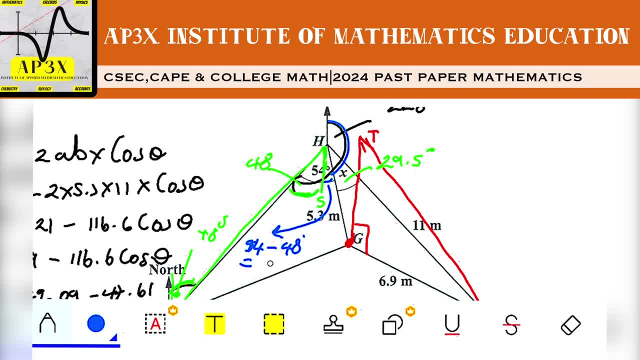 So that little piece of angle right in here is going to be equal to, say, here, 6 degrees. So this little piece right in here. Let me just shade it for you right here. It's, in fact, 6 degrees. All right? 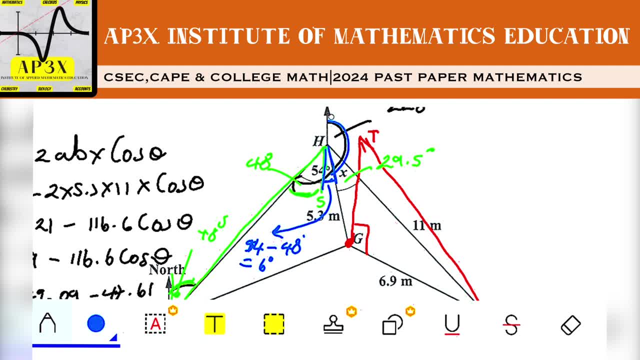 So now that I know that angle is 6 degrees, I know that the complete angle coming around all the way here is, in fact, say here, 180. 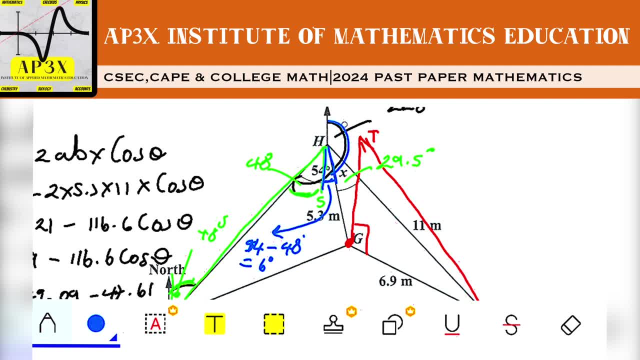 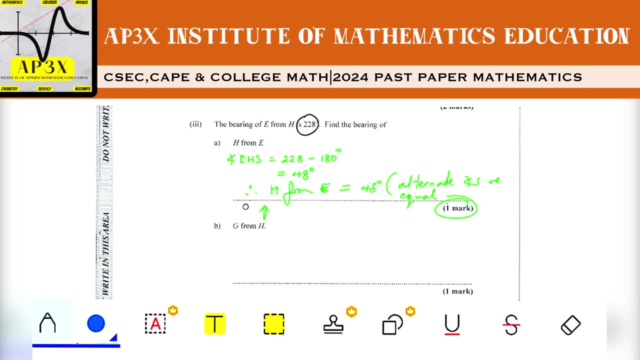 So all of this angle is from north come all the way around to this constructed auxiliary south line that I drew is 180. And I know that a part of it is 6 degrees. So I can find the rest. So I can just simply scroll down to my section here, and I can say G from H is, in fact, 180 minus 6 degrees. 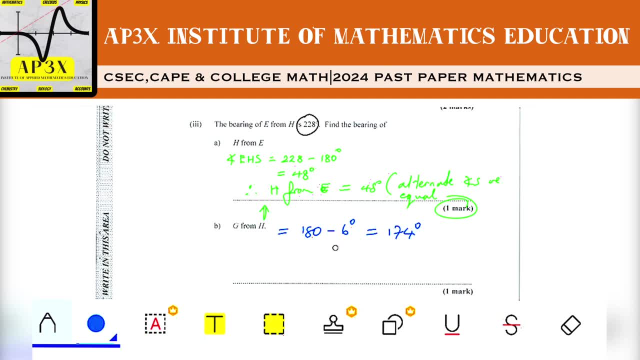 And that's equal to 174 degrees. 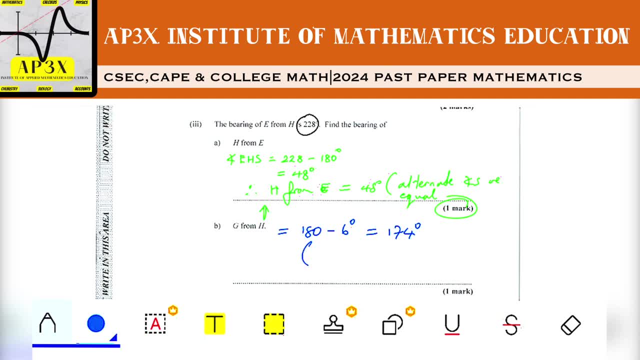 That reason would have obviously been that north to south equals 180. So north to south equals 180 degrees. 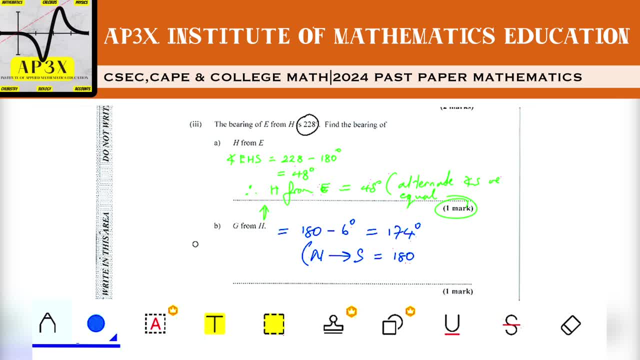 And my additional calculation would have been that 54. Takeaway. 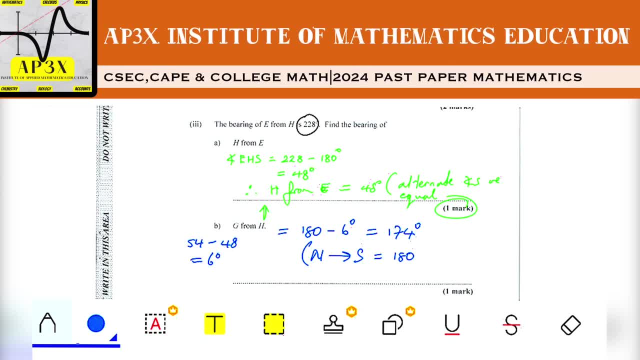 48 degrees would have been equal to the 6 degrees here. We could actually name that angle. 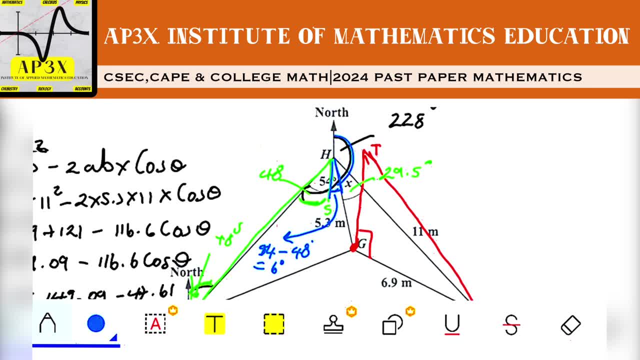 All right? We could name that angle, that 6-degree angle that we zoomed up here. 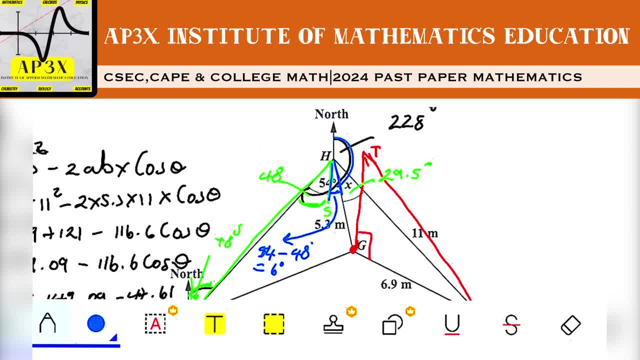 We could name that angle SHG. So angle SHG. So angle SHG here. 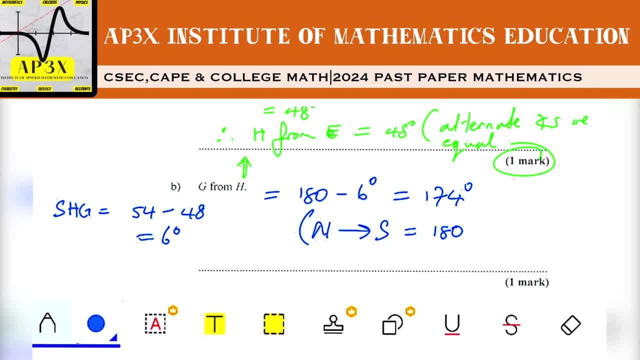 SHG is equal to 54 minus 40, which is 6 degrees. And so, therefore, G from H would have been equal to 180 minus 6. So 6 degrees equal 174. All right? 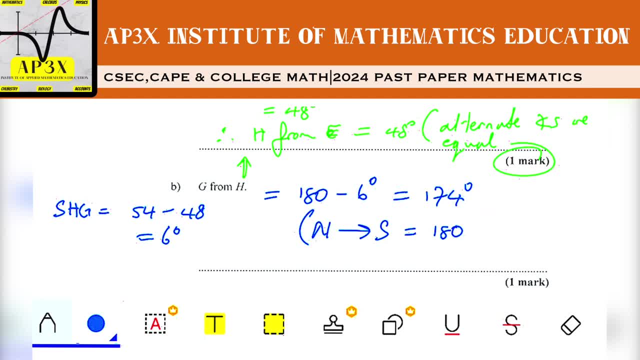 Angles at a point in a straight line measures 180. All right? You could do that. 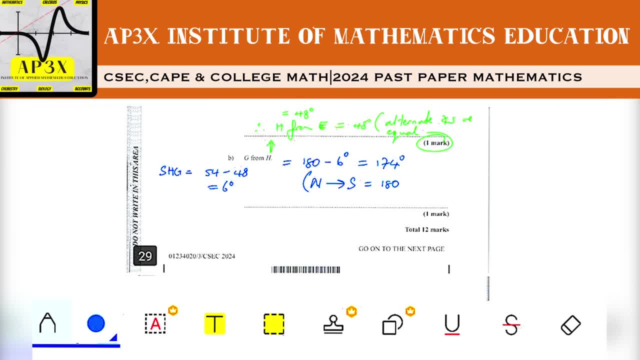 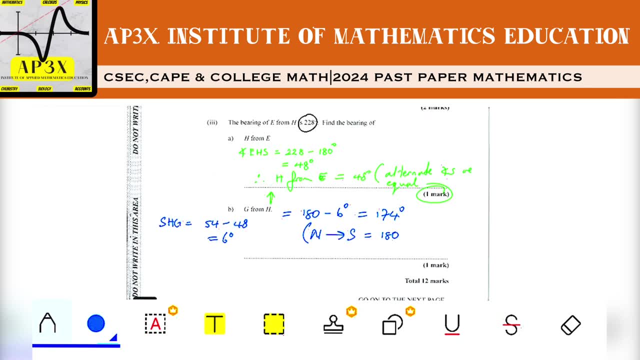 So as I said, guys, circle geometry can be very, very tricky. You really have to be able to see in between diagrams, the angles and so forth. But as I said, if you want some real practice on it, check out my tutorials on circle theorem. It can be quite helpful. All right? So this was a tricky one by CXE. 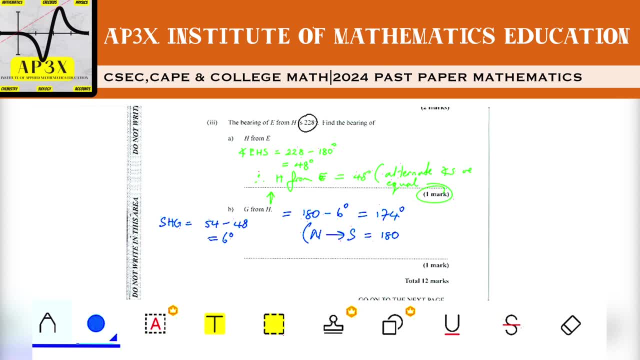 Definitely put a number on this one. So definitely the difficulty level of this question, I would say, is about 6 or 7 in terms of what a student needs to know. 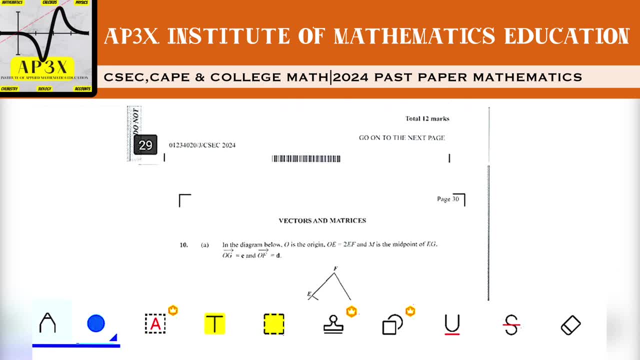 So definitely, hopefully, that little demonstration there helped you out. 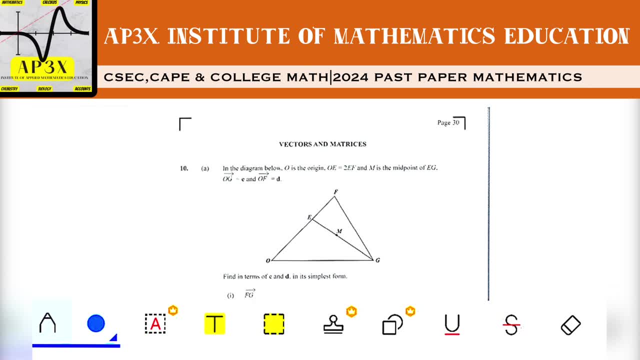 So we're going to be moving on to the last question then of this particular paper here. We are just approaching an hour. 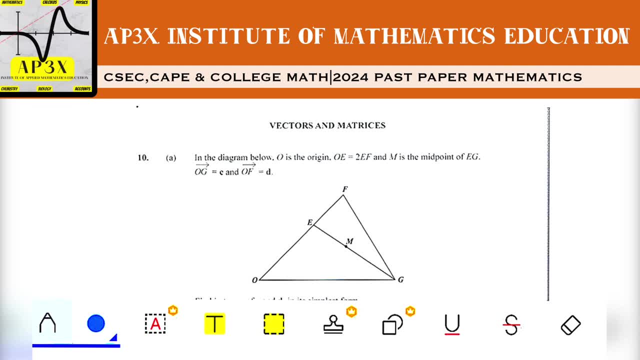 It did take some definite detail work, you know, to get to this point. So hopefully you have liked the video and you are, in fact, learning as we go along here. 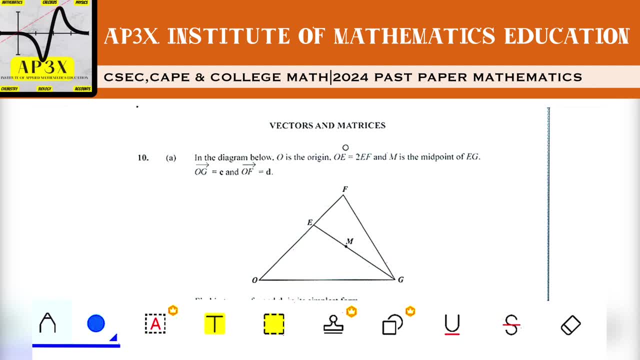 Now, in the diagram below, O is the origin, O to E is 2 times EF, and M is the midpoint of EG. 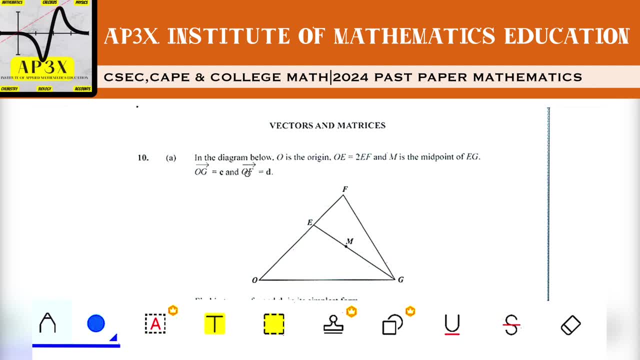 The vector OG measures C units and the vector OF measures D units. 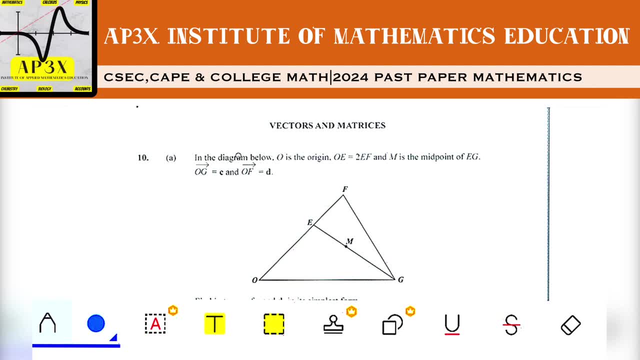 Let's try to interpret what the sentence is saying in this instruction here. 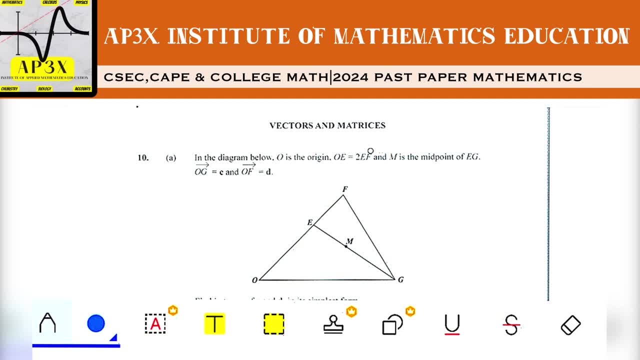 And vectors is also another challenging topic for many math students. So hopefully this might be helpful. 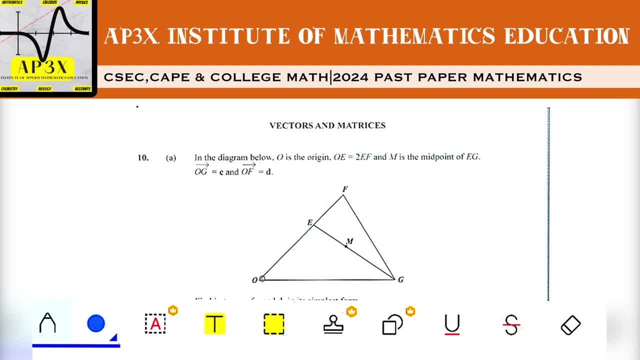 So first it says O is the origin here. So that's 0, 0. And E, O to E, that's O to E, is equal to 2EF. 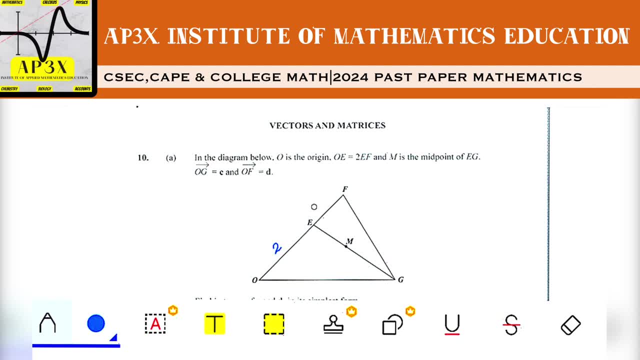 So that means this ratio here is a 2 to 1 ratio. Because it takes 2EF, so it takes 2 of this distance here to make 1 of this distance here. All right. So it's a 2 to 1 ratio. We get that. All right. 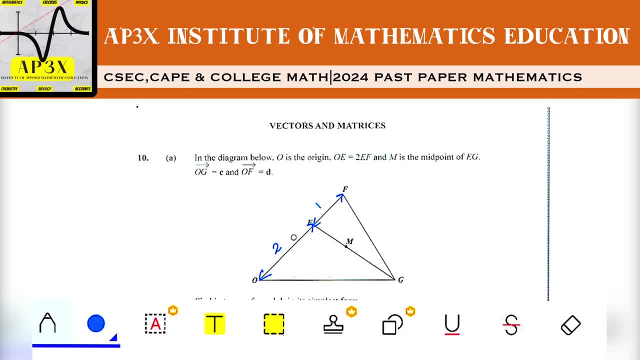 So O to E is 2 and E to F is 1. So it takes 2EF to make 1OE. All right. Fair enough. 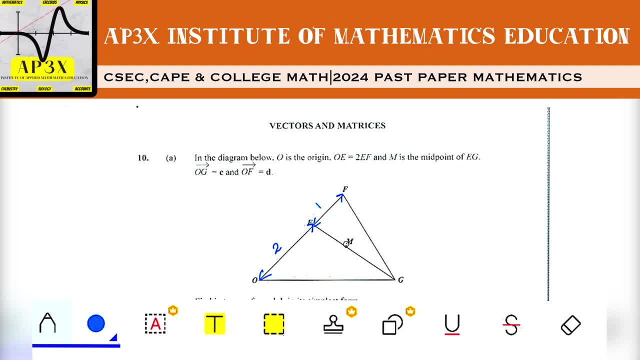 M is the midpoint of EG. So when something, when a point becomes, or when a point lands in the middle of a line, it says that this segment of the line is equal to this segment of the line. That's what we know for sure. And it says that OG is C. Units. So O to C, O to G is C units. Let's put our C units here. 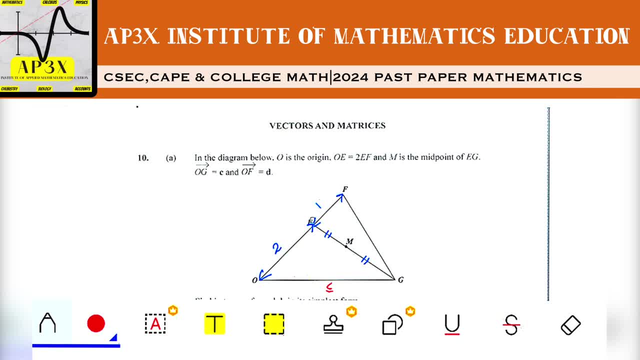 And O to F here, O to F all the way up here from O here down here to F all the way up here is in fact, say here, D units long. All right. 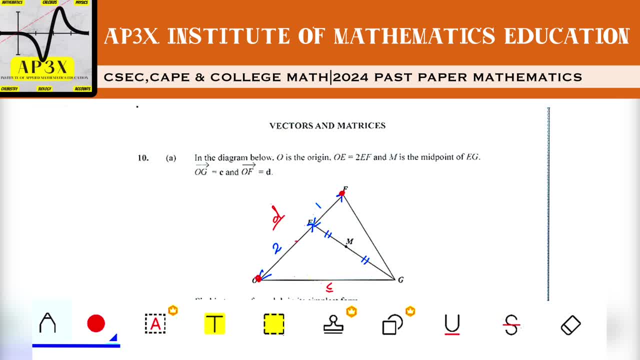 So I know that from here to here is O to F. So our vector R should be going that way. And our vector R for this one is going that way, O to G. And O to F. All right. 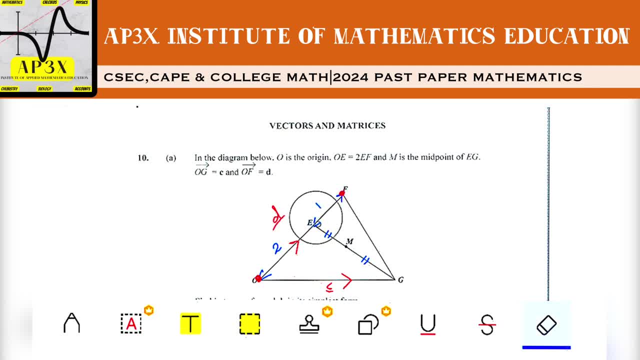 Notice, let me just clear this up a little bit here so it doesn't become too confusing. All right. So there we go. We have a 2 to 1 ratio here. All right. We got you there. All right. Beautiful. 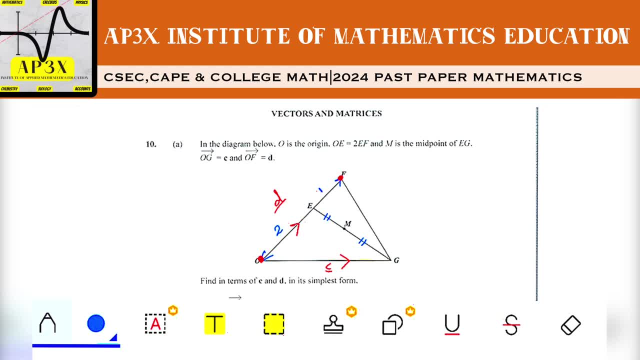 So now next, now they're asking us then to calculate, say here, or find in terms of C and D, in the simplest form, FG. So F to G, then we have to use what is known as. The triangle laws of vectors. 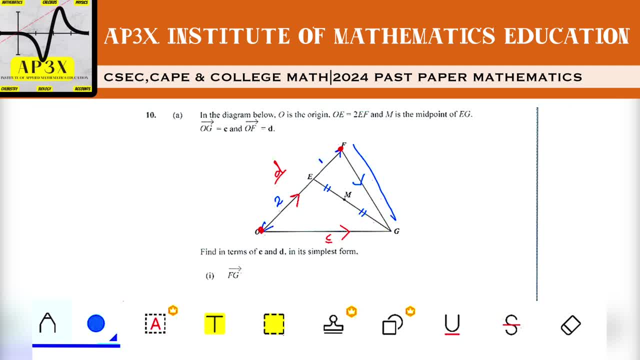 So if we go, if we want to go from F to G, we have to go from F back to O, and then we have to go from O to G. So now find this, then we are going to simply say using triangle law of vectors. 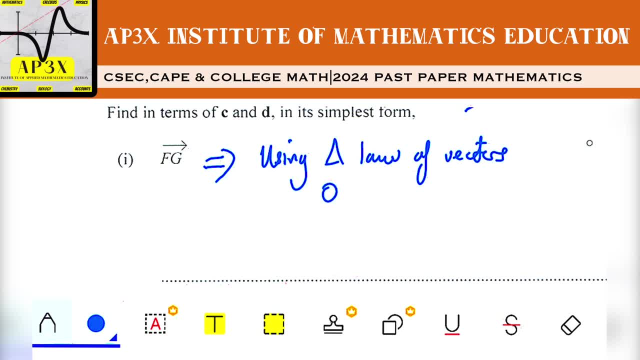 We're looking then at O. Pardon me. 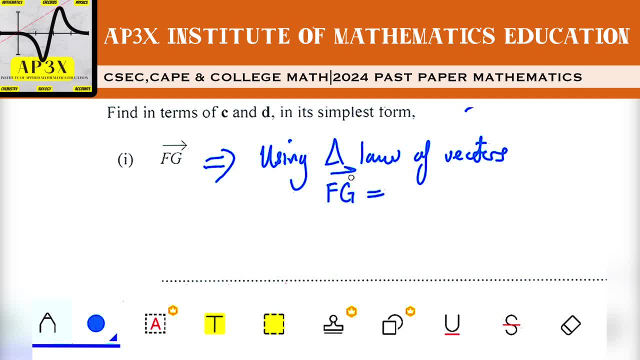 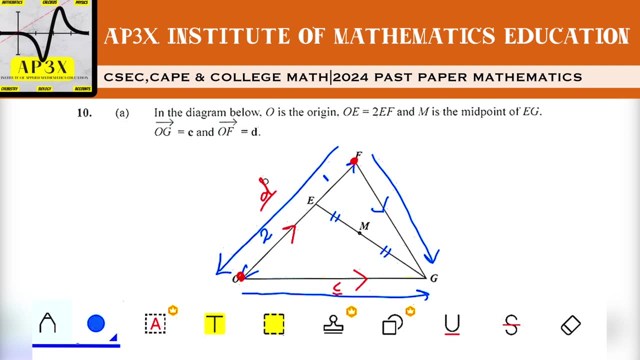 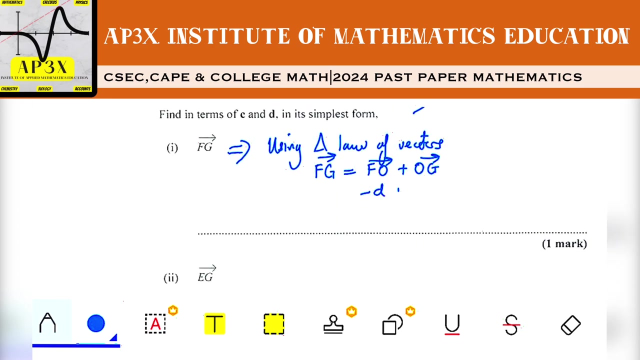 F to G is in fact F to O plus O to G. So F to O will be the inverse of OF. So since O to F is D, then F to O is minus D. It's the inverse vector. And then, of course, O to G. 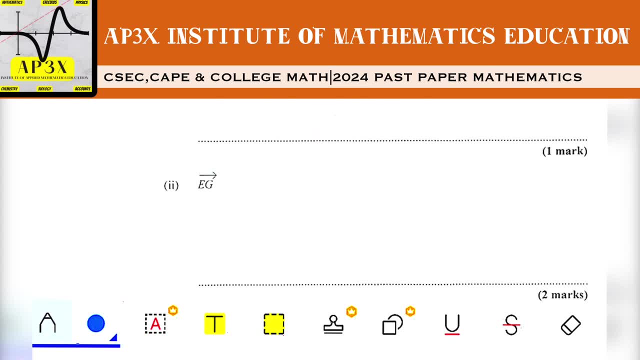 Clearly, we were told that O to G is C units. So therefore, then that is minus D plus C. And that's it. That is our answer. 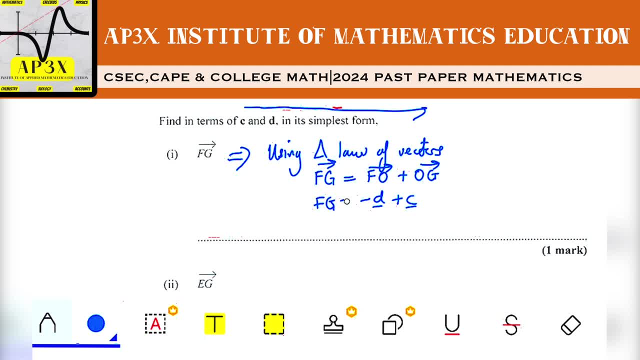 So F to G is in fact D plus C. That is our result. Let's just put that in a little box here. All right. 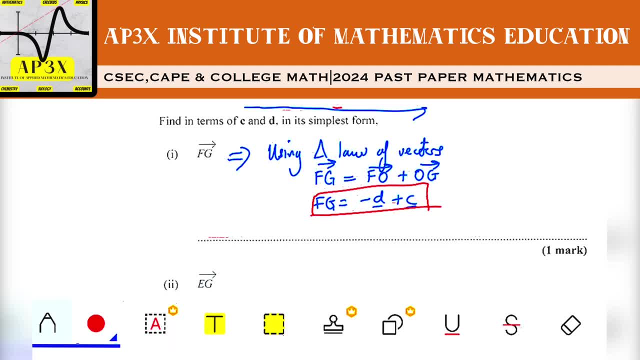 So it's not really challenging in terms of getting the result, but you must be familiar with the concept of triangle laws of vectors. Now, let's look at finding. E to G. 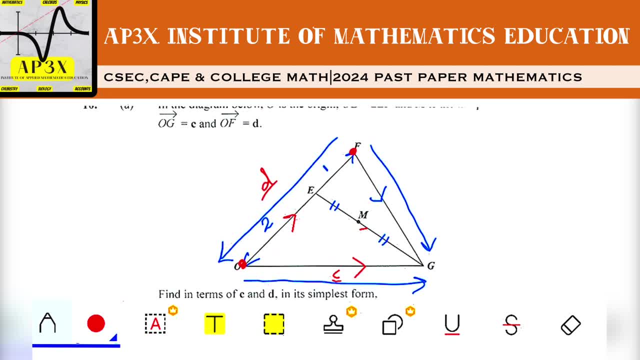 So from E to G is right here. So let's put our arrowhead here. 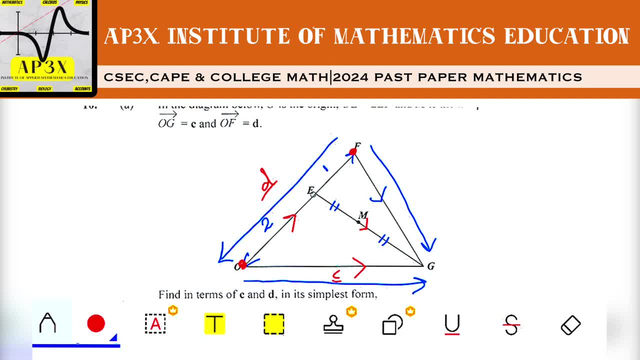 So E to G, once again, it's the same procedure. We're going to go from E to O and O to G. Or you could go E to F and F to G, whichever one you want to do. I'm just going to go with what was already given to me. It doesn't really matter which direction, though, as long as I end up back at the ending point. 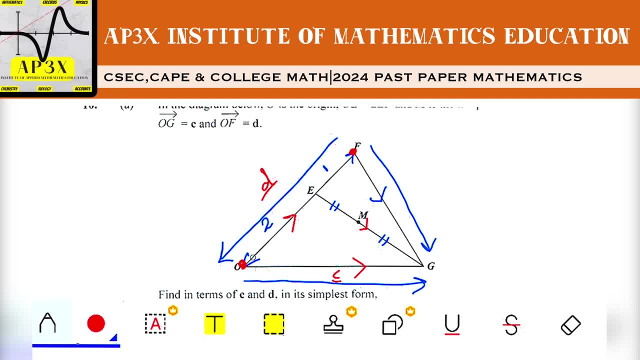 So I'm going to go. I'm going to take E to G. It's going to be E to O. Plus O to G. E to O. Plus O to G. 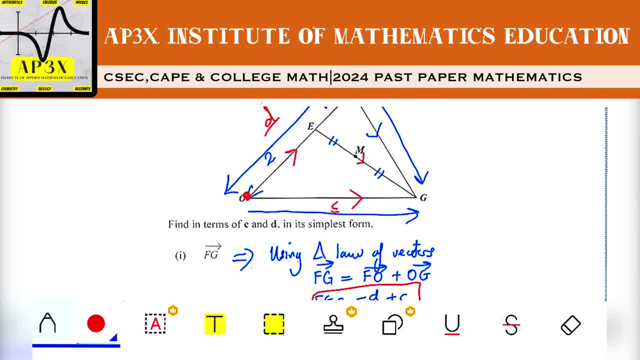 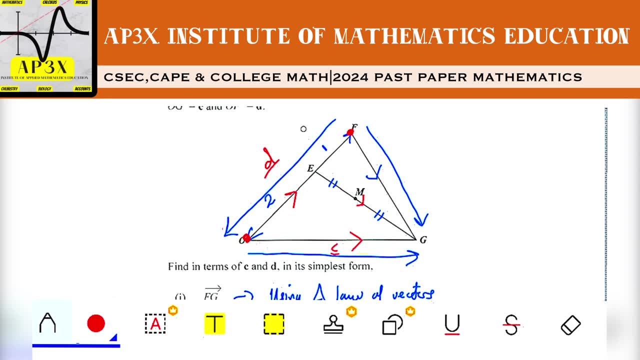 Now, we know that there was a relationship between EO and the whole entire vector OF. We know that the whole length is D. So already I know that from here to here is going to be two thirds D. 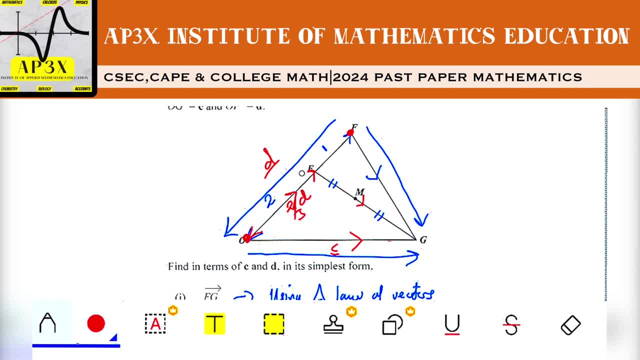 It's going to be two thirds D. It's two thirds the whole entire line. 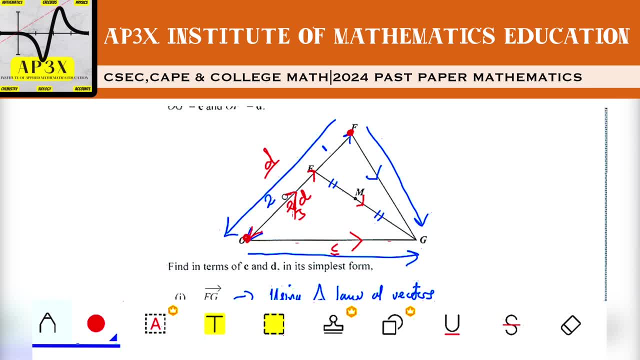 So this section here from E to O, remember the vector is going this direction, but we are forced to go that direction. So we know that O to E compared E to F is a two to one ratio. So I know that the total parts of the line is three and O to E is two out of the three parts. So it is. 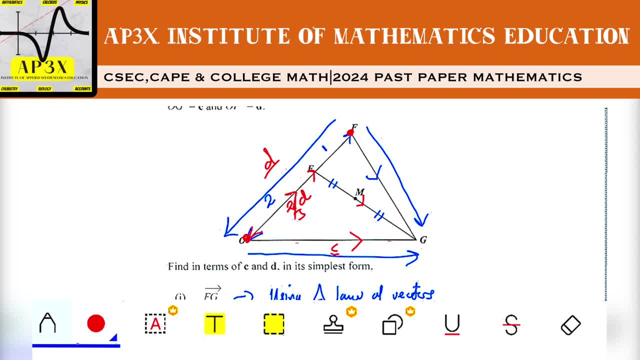 It is two thirds, but it's negative because I'm going in the opposite direction of the vector. 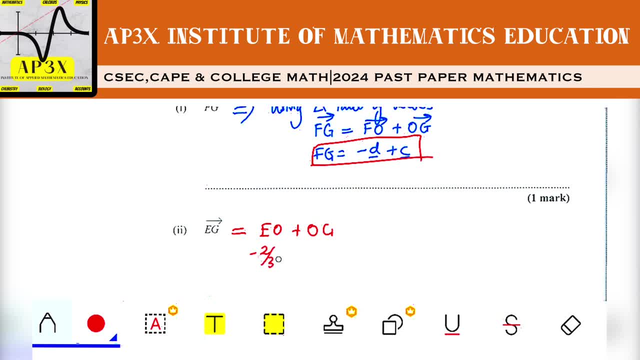 So E to O is negative two thirds D. 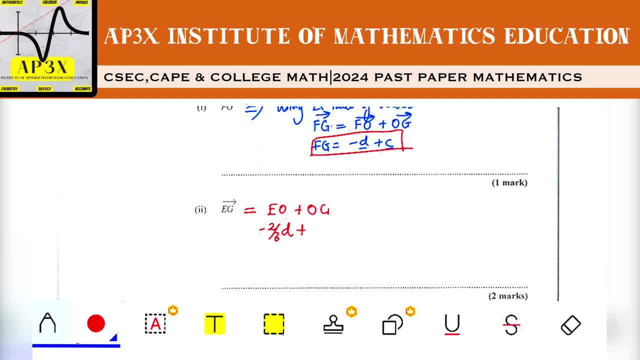 And O to G, as you would have already seen, is in fact C. 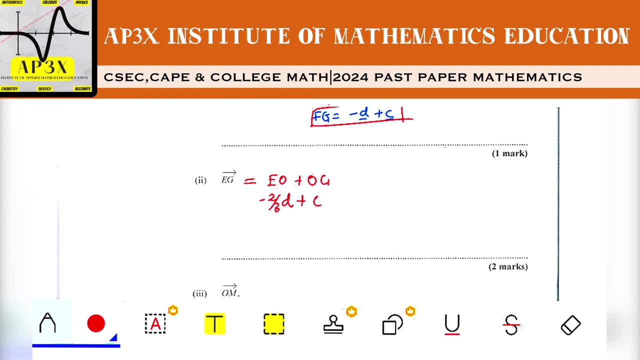 So that's negative two thirds D plus C. Or if you do it the other way, you might end up with C minus two thirds D. Same answer. All right. 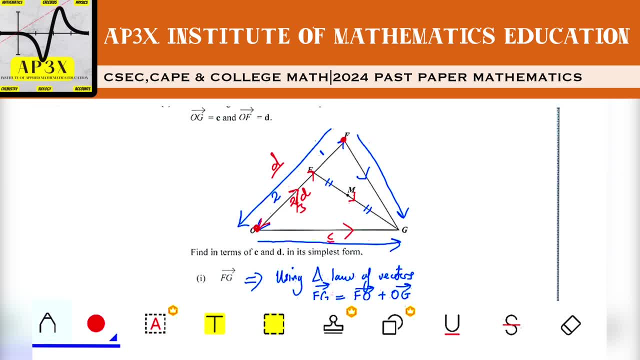 And then O to N. And then O to M, we must connect a line from O to M, obviously. 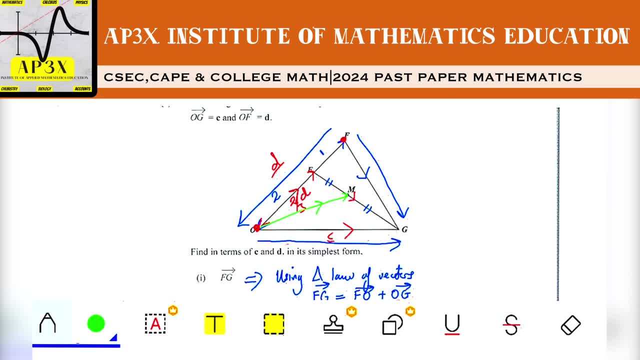 So from O to M here, put on our arrowhead here, is again another triangle. O to M is going to be from O to E, which is in the same direction of the vector, which already we established just moments ago that O to E is two thirds. 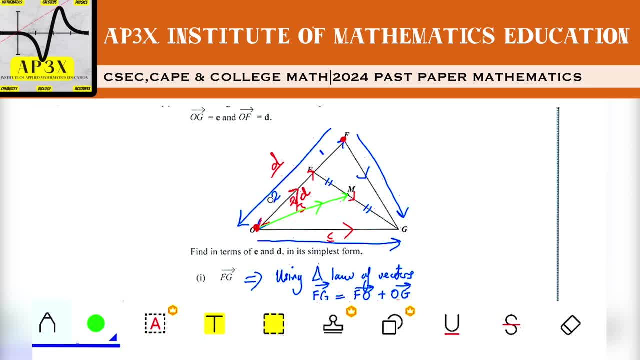 Why two thirds? The ratio is two to one. So when I add two plus one, this whole entire line, O, F has been split into three parts. And so because the ratio is two to one, then it simply means then that O, E is going to be two out of the two, three parts here. 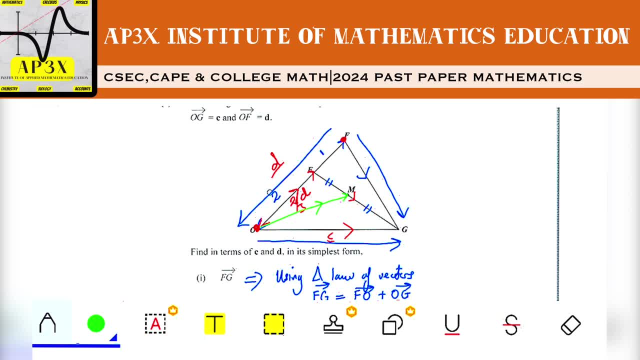 We are going in the same direction of the vector. So O to E is going to be two positive two thirds D. 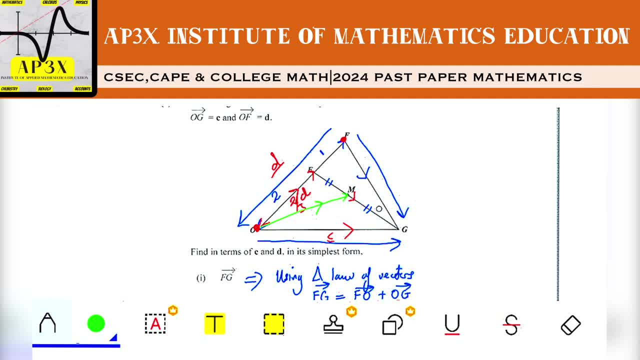 And notice then that E, M is going to be half of E, G because M is the midpoint of E, G. 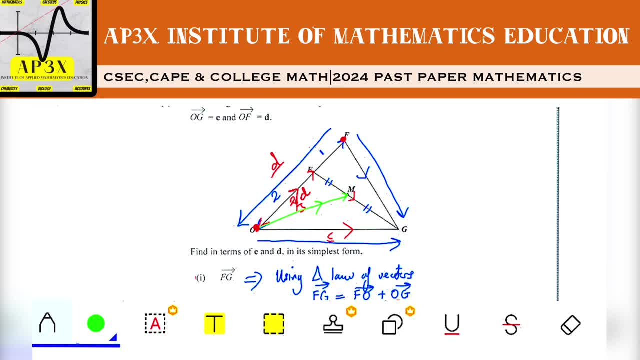 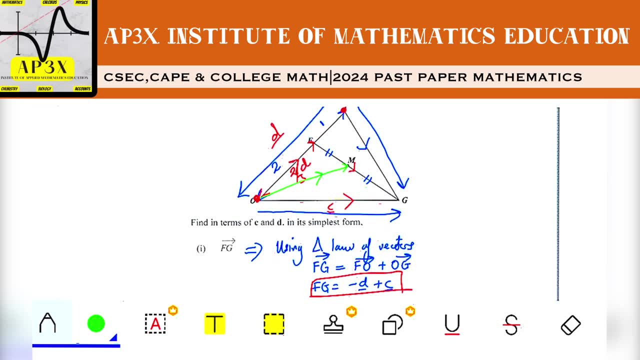 So E, M is going to be half of E, G. So then I could write a statement here and say that O to M is going to be equal to O to E plus E to M. 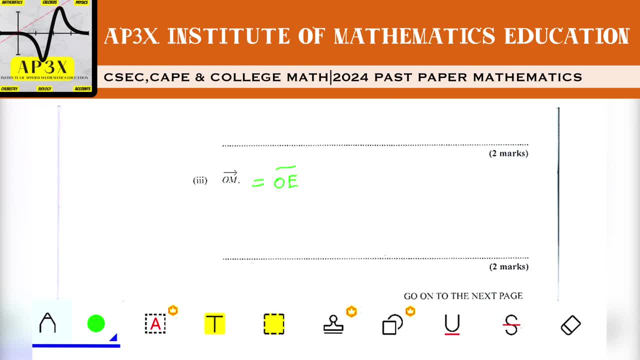 So O to M is going to be equal to O to E plus E to M. 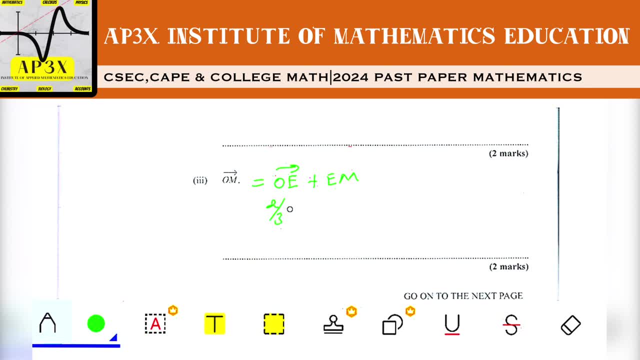 And O to E is going to be two thirds D. Because up here we were looking for EO. So EO was negative two thirds D. Obviously then OE is going to be positive two thirds D. 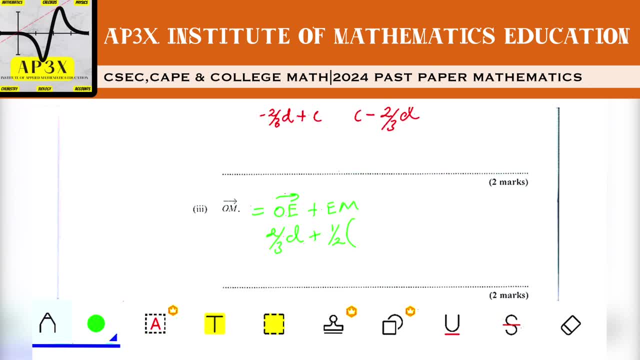 And then of course, E, M, we just established that that is going to be half the length of E, G. And see, we have here E, G, which was just calculated. 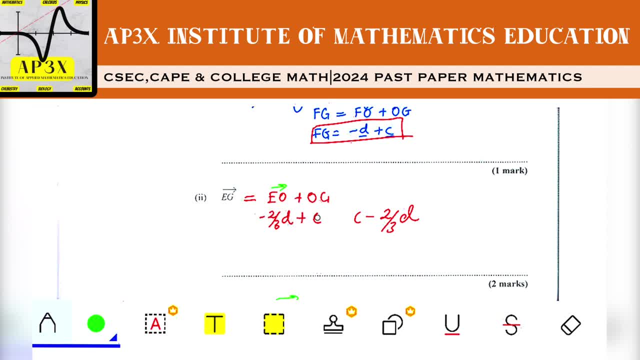 E, G is going to be negative two thirds D plus C. 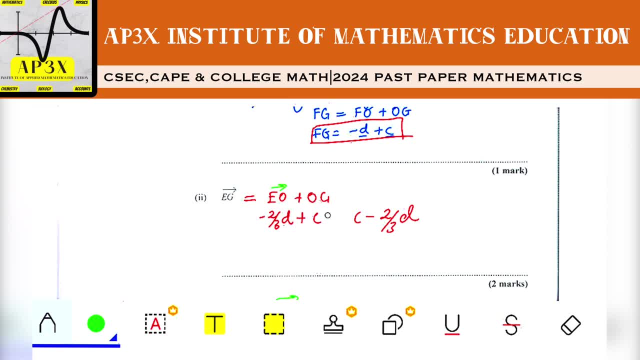 But since, oh, pardon me, is this E, G? Yes, this is in fact E, G. 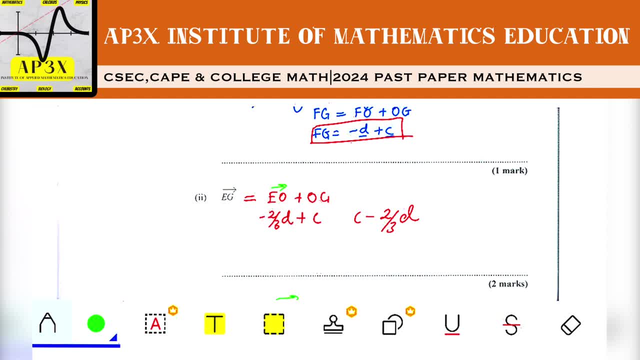 E, G we had worked out to be negative two thirds D plus C. 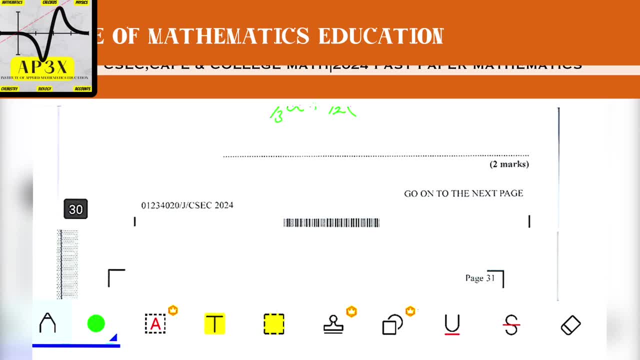 So since E, G is negative two thirds D plus C, then it's going to be half. 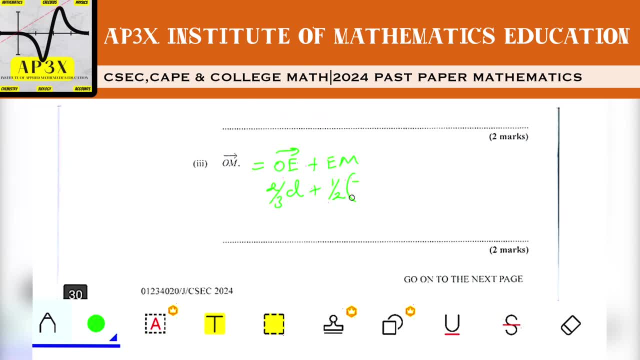 Negative two thirds D plus C. So then this is two thirds D plus a half of two thirds D is going to be one times negative two, negative two over two times three. 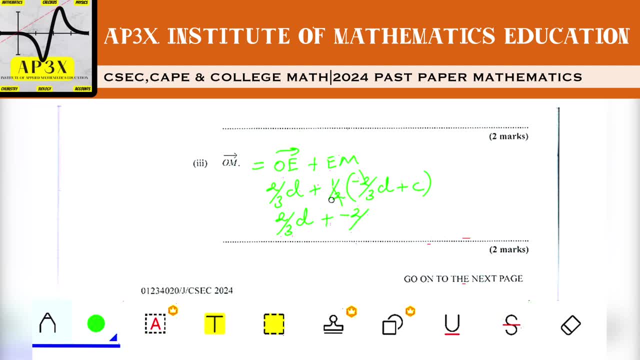 Oh well, we can just cancel the two twos here. So a half of negative two thirds. Is negative one third. So we can just fix that up right away. 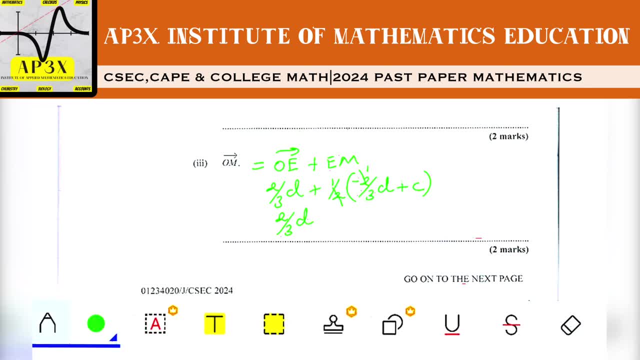 So a half of two thirds. This two here cancels this two here. Already. So this two here cancels this two here. So we'll have negative one over three D. So negative one over three D. All right. 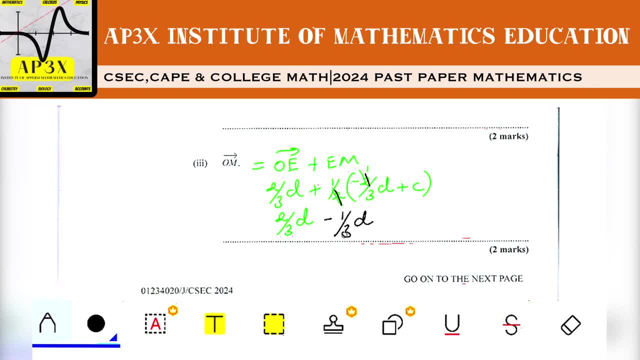 So that's a half. So a half multiplied by this gives us negative one third D and a half multiplied by C. 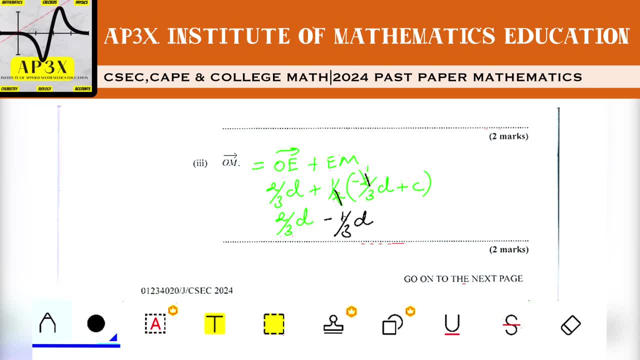 We have to use the half to distribute inside. So half of this is negative one third D and half of C becomes a half C. 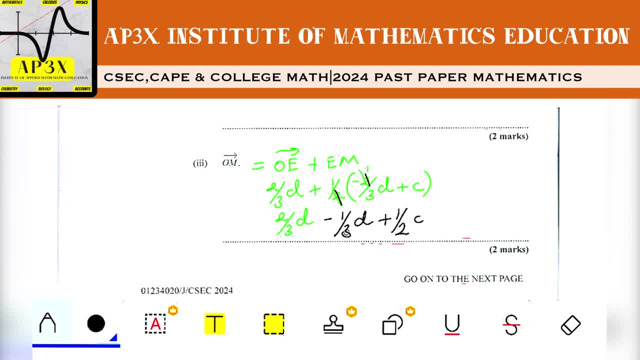 Now we have to group like terms here. We have two thirds D take away one third D. Well, that's kind of straightforward. 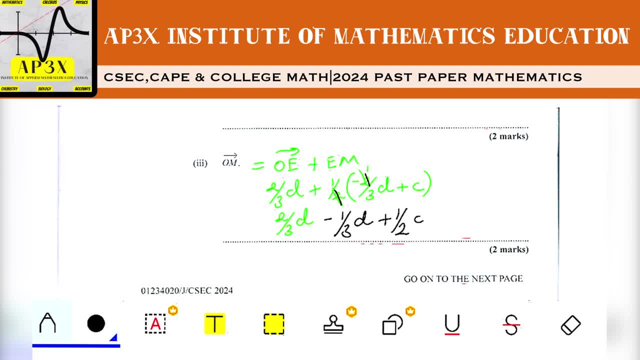 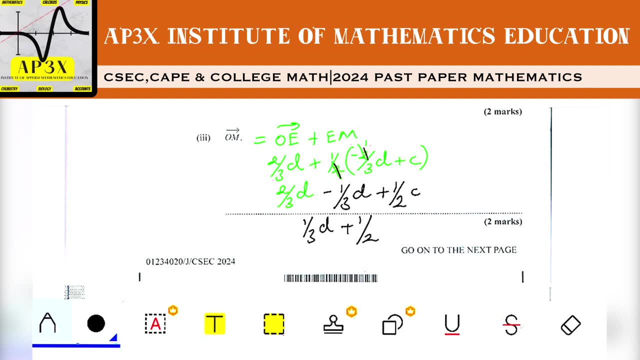 The LC and the denominators are the same. So two take away one is in fact one third D. Plus a half C. And that is your result. All right. 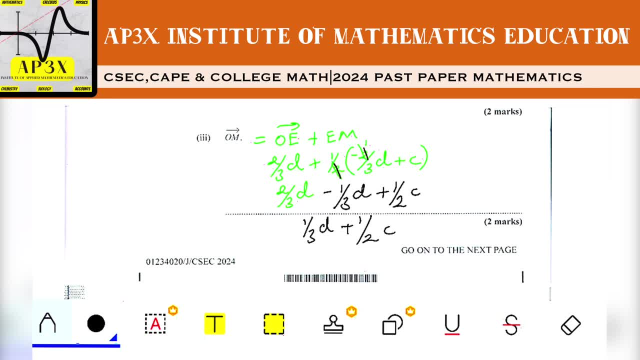 Vectors can be a little bit complicated at times. But if you have any knowledge about triangle laws of vectors, definitely you'll realize that it's not as challenging as it appears to be. All right. 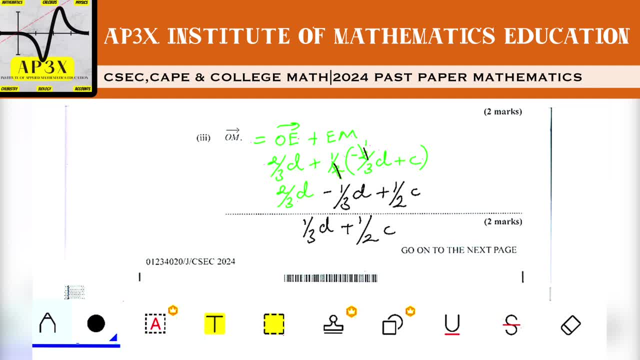 I'm not sure if at the point of you watching this video, I would have already made a vectors video or series of questions, past people questions. If it's available, you can check my vectors playlist. 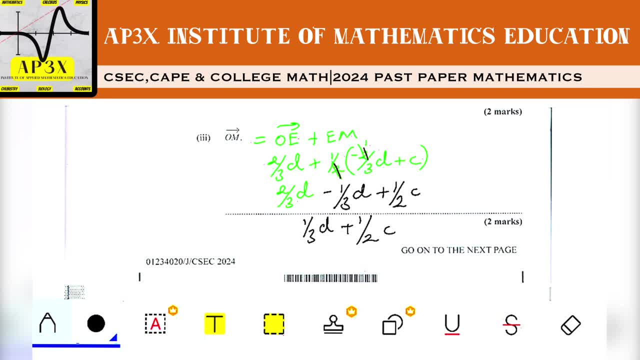 If not, then hopefully upon watching this video, I would have already posted that video on that. All right. 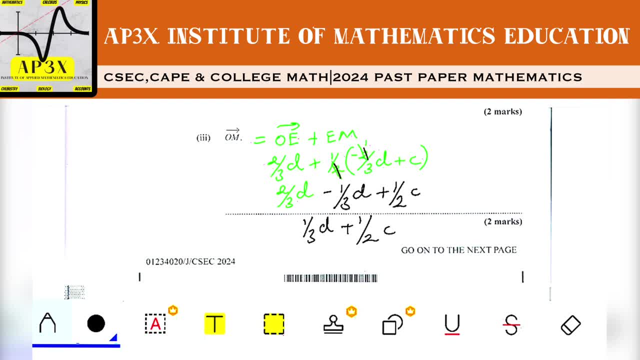 So look out for my vectors review tutorial video. All right. 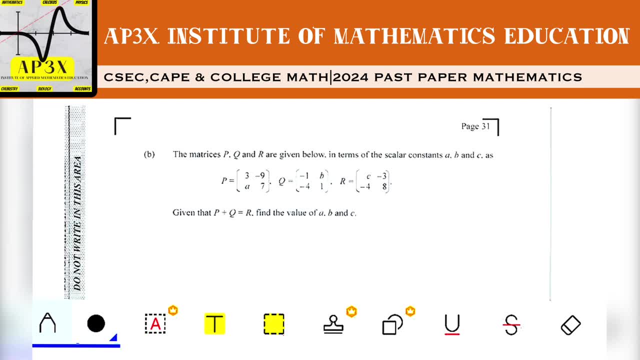 And then now just to wrap up the paper here as we're a little bit over an hour, 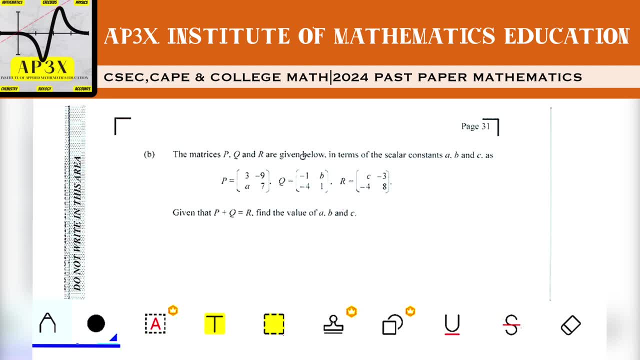 the matrices P, Q and R are given below in terms of the scalar constants. A, B and C. So we have A here, we have B here and we have C here. It says, given that the vector, the matrix P plus the matrix Q equates to the matrix R, our task is to find the values of A, B and C. All right. 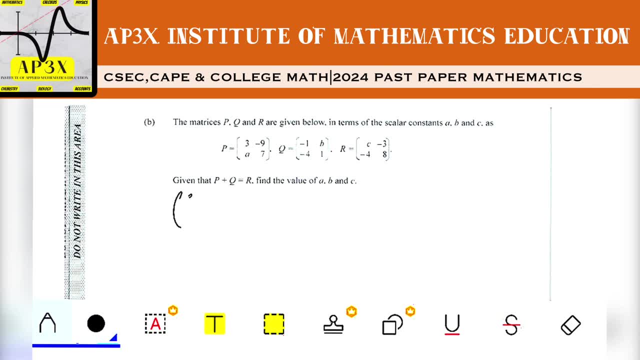 So we're going to write down our matrix P here, which is 3, negative 9, A, 7. We're going to add that then to matrix Q, which we have here to be minus 1. 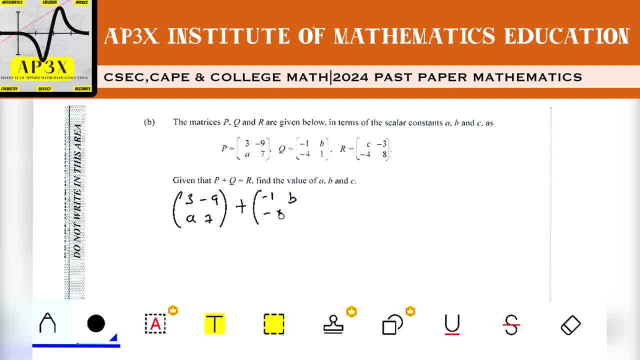 B, negative 4, 1. 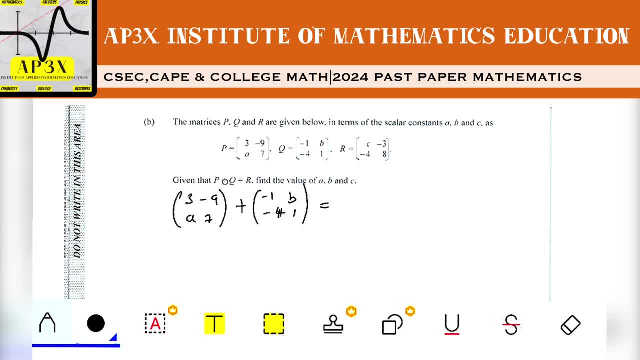 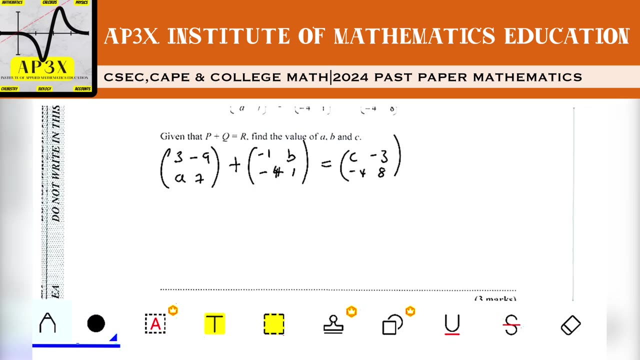 And we're going to equate that then to the matrix R based on the conditions given to us here. We're going to equate that to the matrix R, which is C, minus 3, minus 4, 8. So now when we're adding matrices, we know that we have to add corresponding entries. So the first gets added with the first. The second gets added with the second. The third gets added with the third. And the fourth gets added to the fourth. So if I add 3 plus negative 1, I'm going to end up with 2. 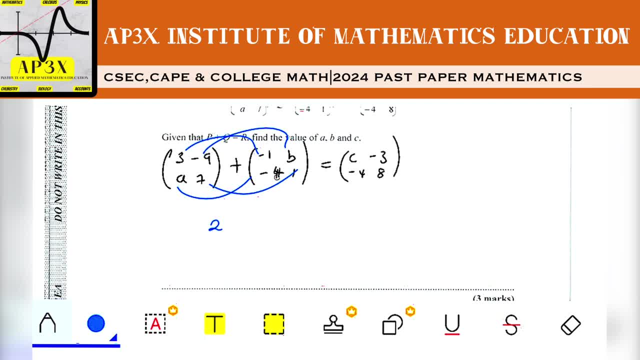 If I add negative 9 to B, I'm going to get negative 9 plus B. You cannot add unlike terms. So we just merge them together. 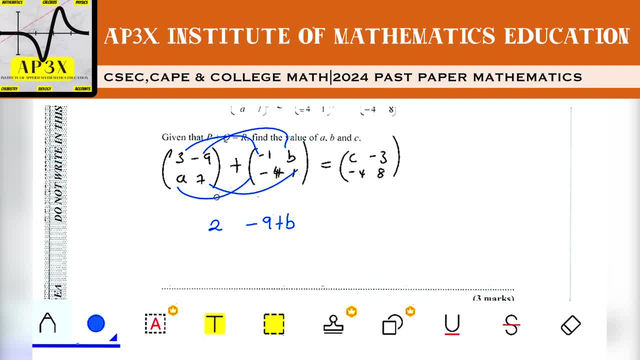 If I therefore add A to negative 4, I'm going to end up with, say here, A, take away 4. 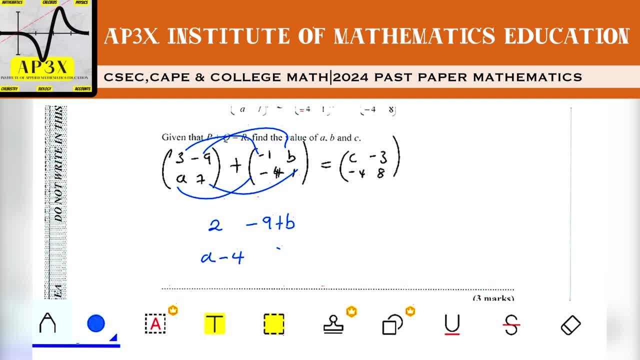 And of course, when I add 7 to 1, I'm going to end up with, say here, 8. And so that sum of matrix is then equated to the matrix here, C, minus 3, minus 4, 8. 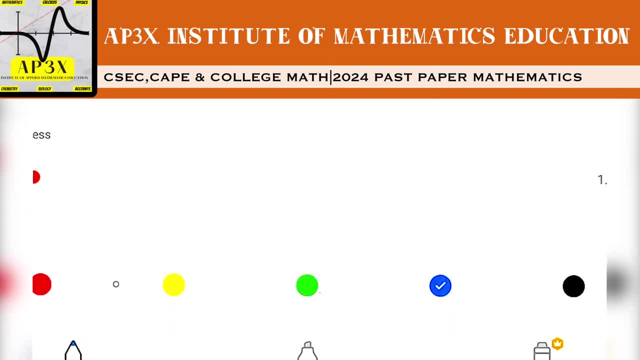 Now we're going to compare coefficients. Sorry, we're going to compare entries. 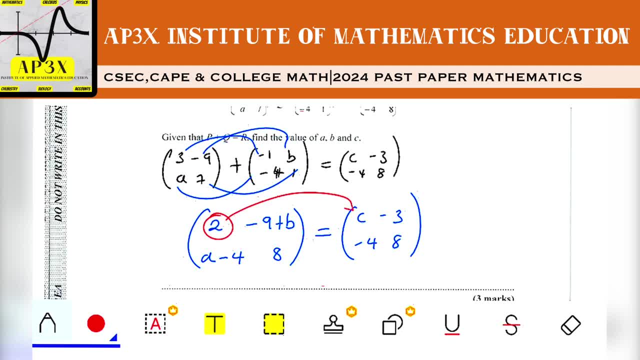 It means then that this 2 here is going to be equal to C. Because if two matrices have... So this 2 here will be equated to C. 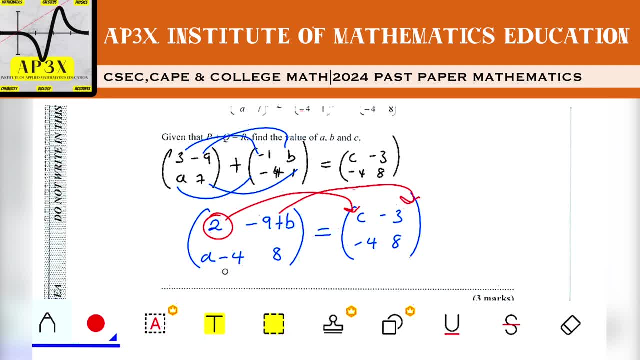 This negative 9 plus B is going to be equated to negative 3. This A minus 4 is going to be equal to negative 4. And this 8, obviously, we had worked it out perfectly to be equal to 8 then. So we know we're on the right track. 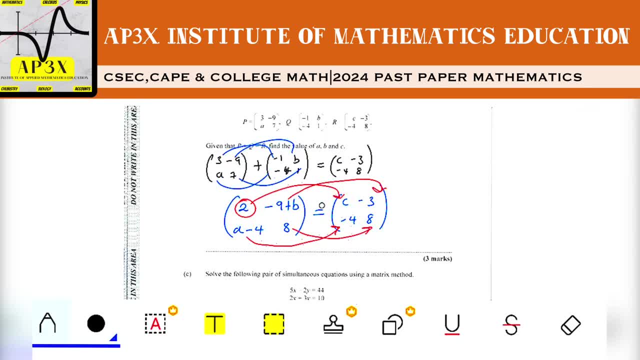 Now to wrap this up then, our first value here is that C is equal to 2. So right away we are gone. That C is equal to 2. 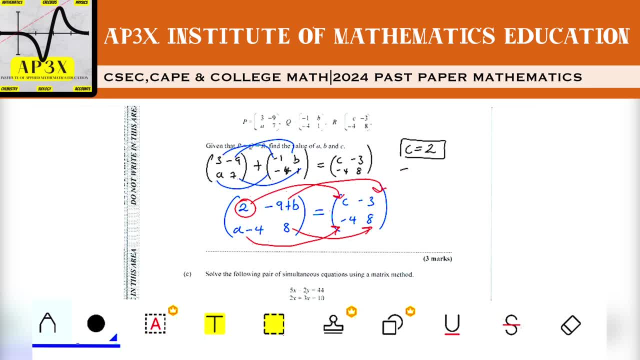 Our next equation here shows us that negative 9 plus B is therefore equal to negative 3. So we can solve this very simple equation, bring the negative 9 over. We end up with B being equal to negative 3 plus 9. 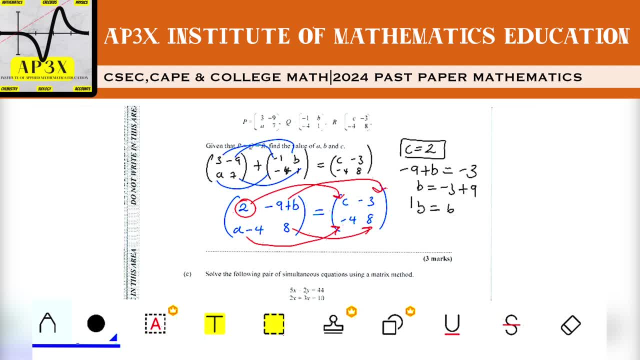 So B then is equal to, say here, 6. That's right. 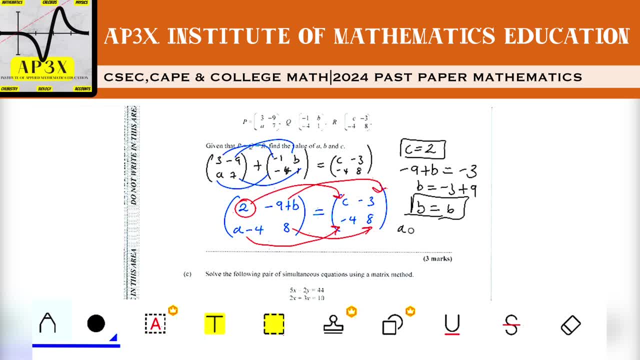 And then, of course, our next equation here is that A minus 4 is equal to, say here, negative 4. 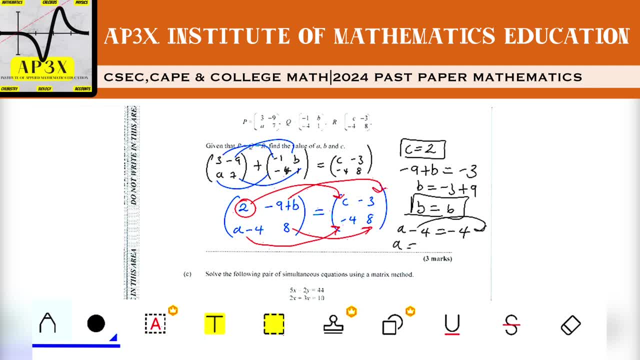 So if I bring this negative 4 over here, I'm going to end up with A being equal to negative 4 plus 4. It so happens that A is equal to 0. All right? And that is my third result. So A is equal to 0. B is equal to 6. And C is equal to 2. 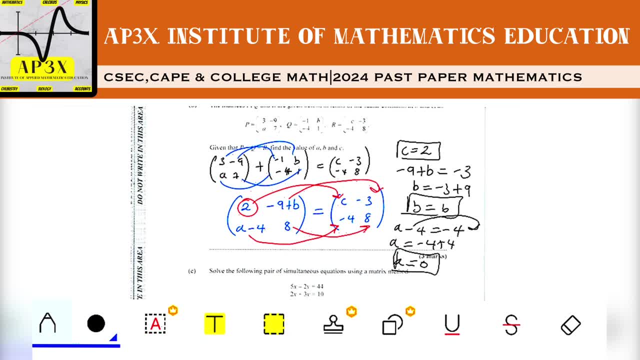 So this particular problem was possible because we know the concept of equal matrices. All right? So hopefully you guys got a hang of that. 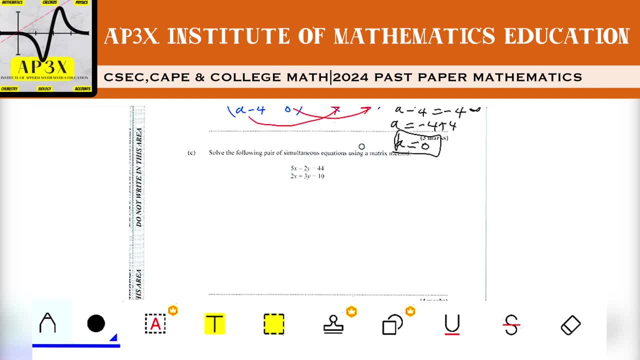 Now. It says here that we are to solve the following pair of simultaneous equations using a metric method. 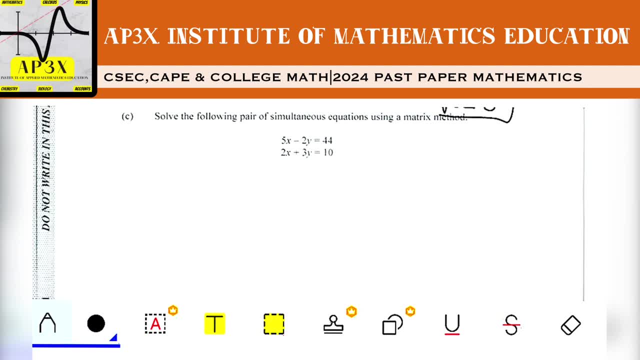 And so there's only one metric method that exists for simultaneous equation. So we're not going to be using the elimination method or the substitution method. 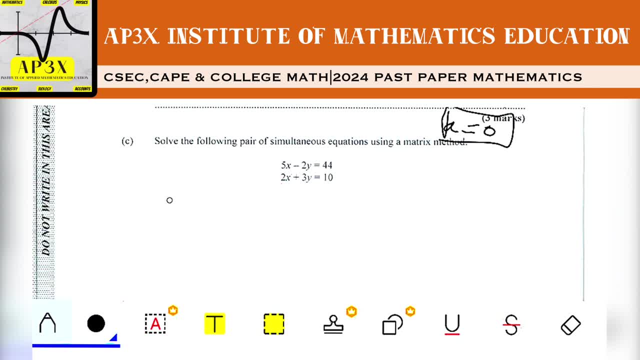 We're going to be using the metric method, which therefore clearly states that A multiplied by B equals C. Pardon me. Equals C. Where B is our unquantifiable. Unknown metric. 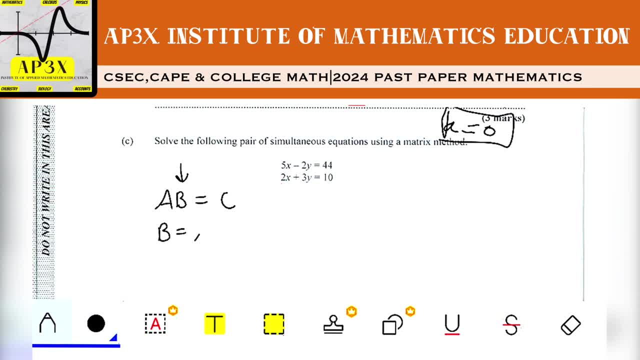 Then that means B is equal to the inverse of A multiplied by C. That is the shortcut method. 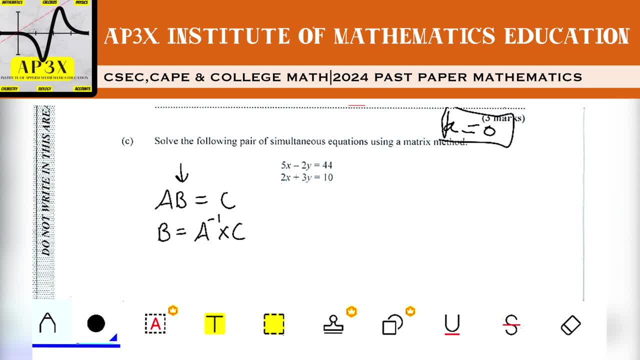 Now, I do not have a matrices tutorial playlist available. So you're just going to take my words for it, guys, and look at other circumstances, other situations where I might have videos explaining matrices questions. But at the moment of making this video, I do not have a playlist on matrices. Hopefully I can get to that. Soon and very soon. But here we go. 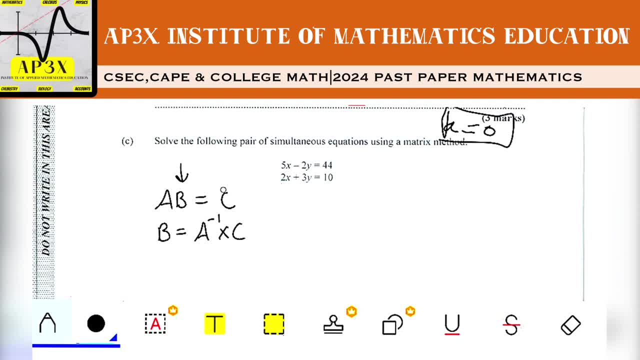 We're going to set up the equation here in the form A B equals C. 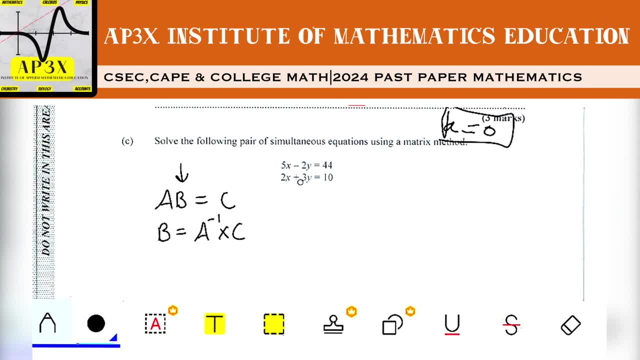 So therefore, to get the matrix A, we're going to take out the coefficients of the equations. 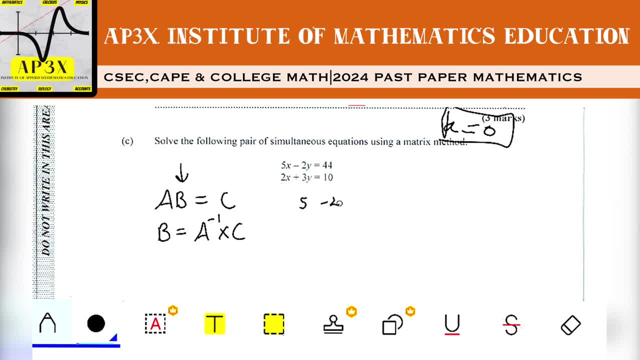 This is five. Negative two. Two. Three. 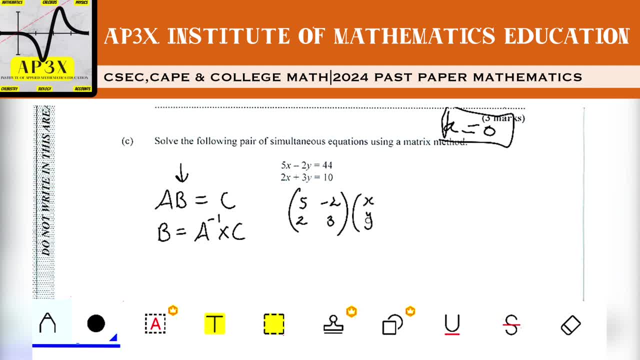 Then the matrix B is obviously going to be the values that we're looking for, X and Y. And then we're going to equate that then to the matrix C, which is representing the solutions to the equation. Forty four and ten. 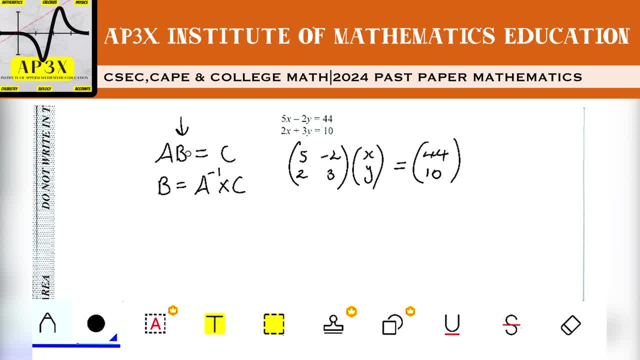 And so that is the setup, of course, then, as I stated that since the matrix B is the unknown matrix A that we're looking for, then X Y is going to be, say here, equal to five, negative two, two, three, inverse. 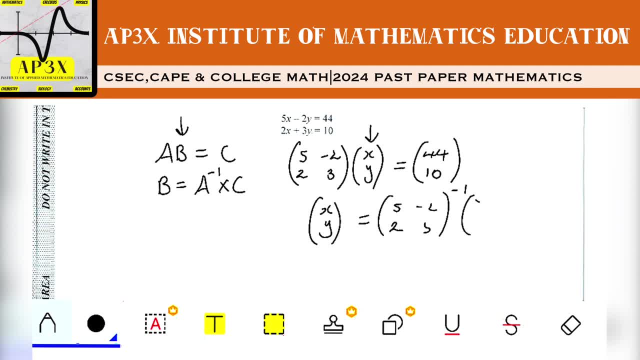 That's minus one. And then we're going to multiply that by forty four, say here, ten, forty four, ten. 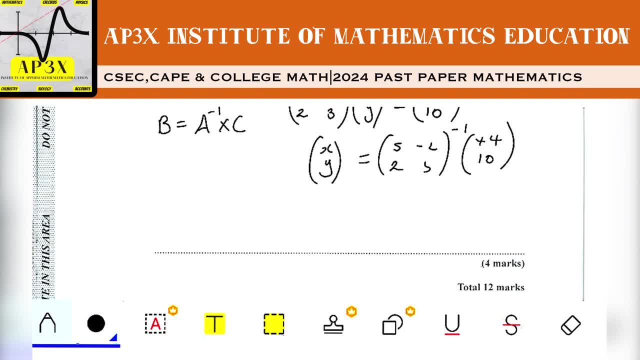 So then our knowledge on inverse of a matrix. Is applied here now to find the inverse of a matrix. 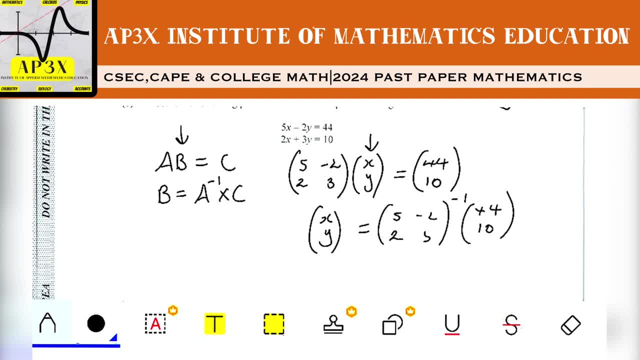 We know that in this case here, we're looking for, um, we're looking for B. All right. So we're looking for a inverse. Let's call this metric here. E. 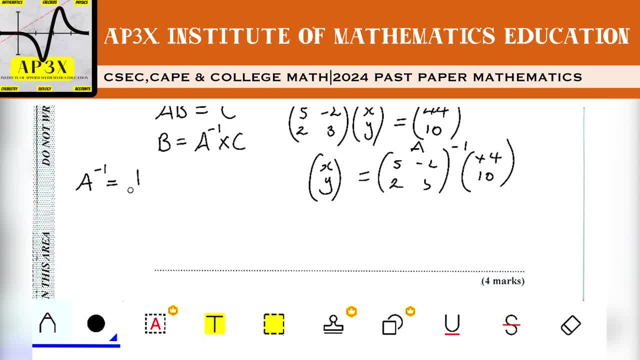 So a inverse is equal to one divided by the determinant of E multiplied by the adjoint of E. 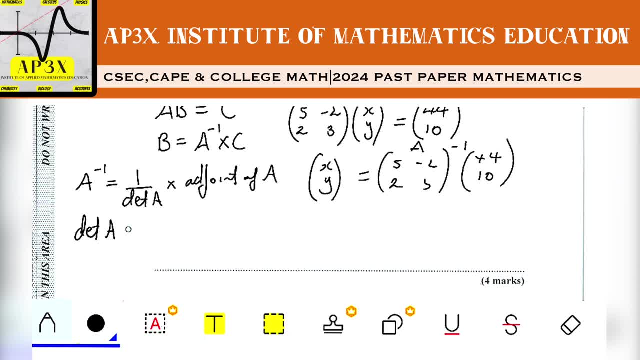 So determinant of E. Is equal to the formula A, D minus B, C. 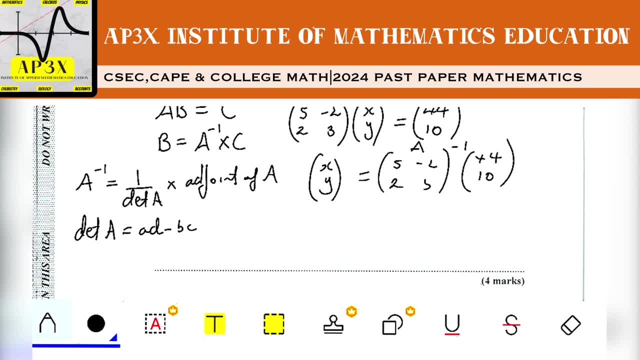 So in this case, A is our first entry, which is five multiplied by our last entry here, which is three. We're going to subtract that from our second entry, which is negative two multiplied by C here, which is again, here, say two. So five times three is fifteen and negative by negative is positive. Two times two is four. So we end up with a determinant. Here of nineteen. 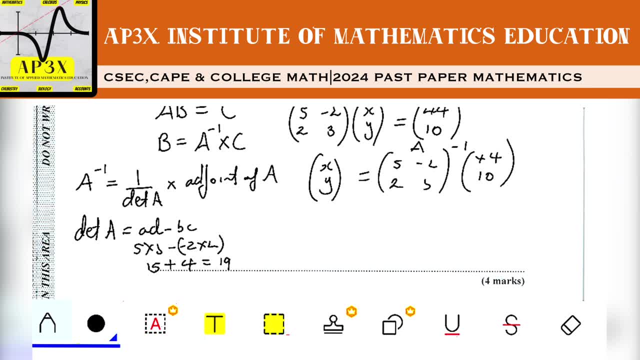 Bear in mind, guys, that I'm working this paper with the assumption that you guys have already been through the topic of matrices and you have an idea. All right. 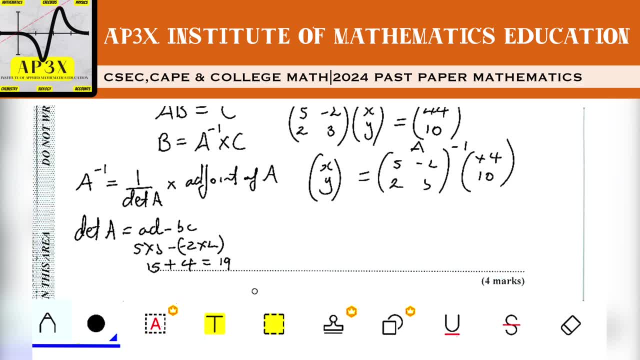 So if you have not done the topic of matrices, then this might look a little bit foreign to you. All right. So here we go. Good. 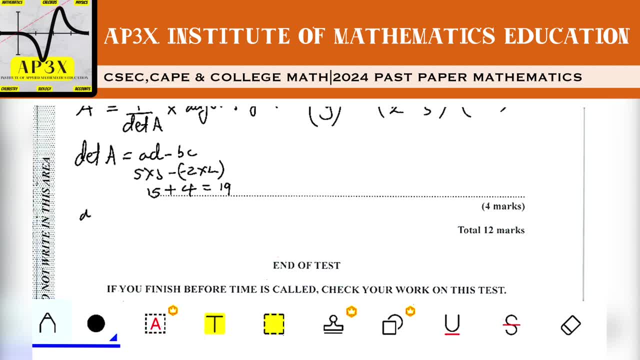 So now that we have the determinant of E, we need to find the adjoint of E. Some teachers will see that this is where you diagonalize the metric or other instructors will see. This is the cofactor of the metric. 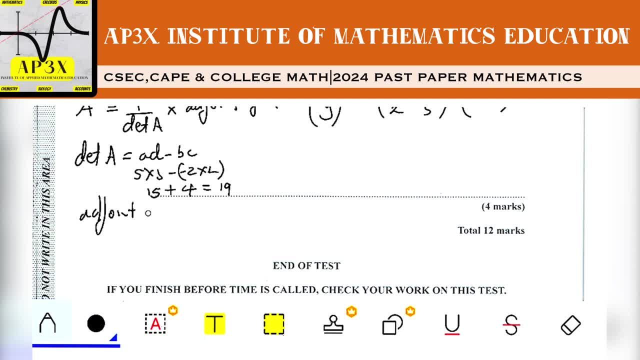 So adjoint, cofactor, diagonalize the metric, same procedure. Now to do this, then we're going to take the lead diagonal of the metric. All right. 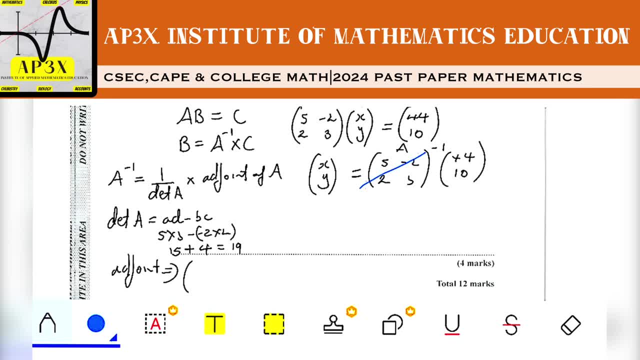 So we're going to interchange the entries of the lead diagonal. So we're going to interchange those entries. 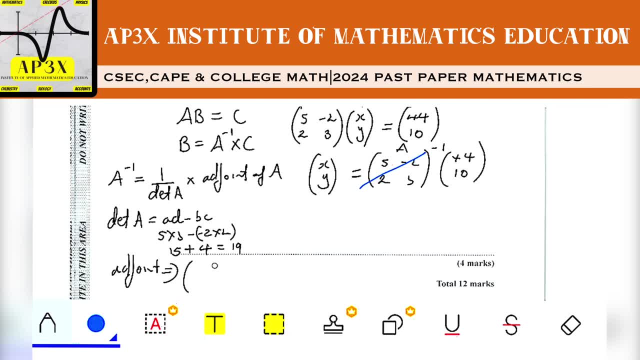 So two negative two, the positive two goes up and the negative two comes down. And then we're going to change the signs of the non-linear. Leading. Okay. So pardon me. I think I made an error here. The lead diagonal. 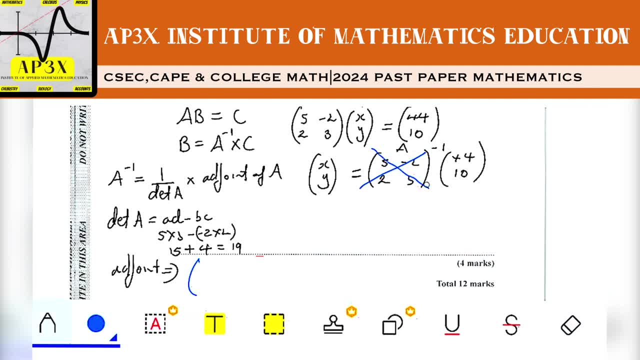 Okay, pardon me. So the lead diagonal is in fact five and three. 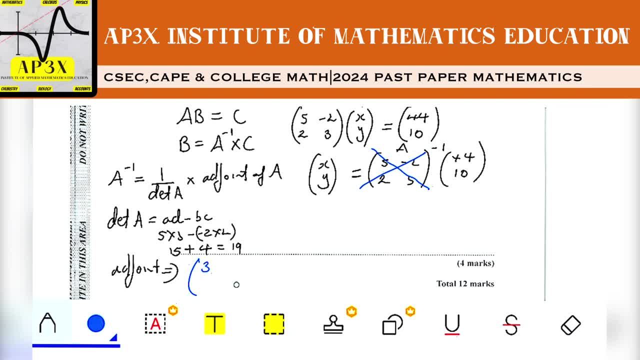 So we're going to interchange the entries of the five and the three. So the three comes up and the five goes down and we're going to change the signs of the non-leading. 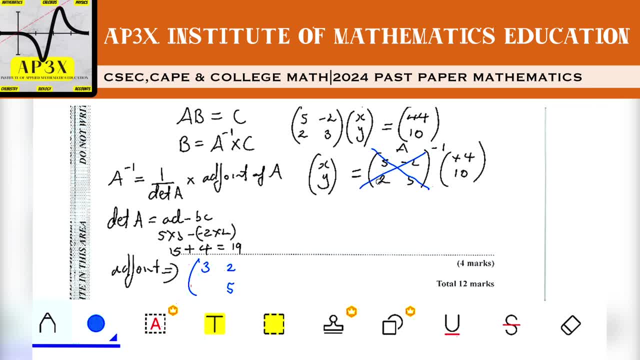 So we're going to change this negative two here to positive two. And we're going to change this positive two here to minus two. 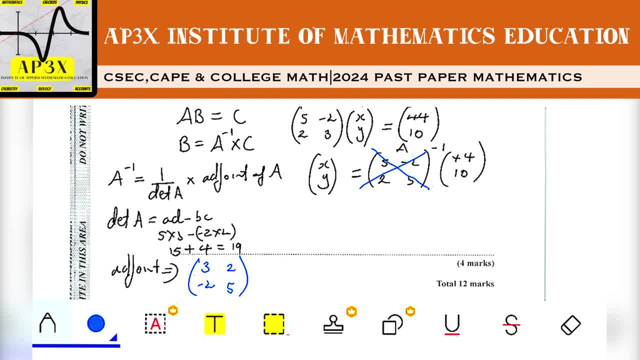 So the metric has been diagonalized or the metric that is the in that is the adjoint of the metric. 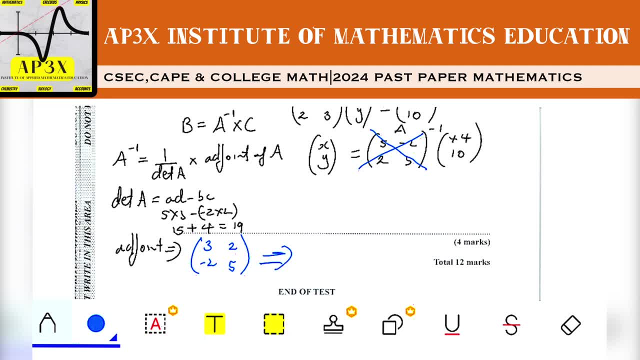 So therefore then to find the inverse of the metric then we're looking at one divided by see here the determinant, which is 19 multiplied by the adjoint which we have here to be two negative two five. Now we could go inside and put each of the entries over 19, but that's going to make the math a little bit more challenging. So I'm going to keep it in its scalar form here and then from here now, I'm just going to use that as my inverse metric in its scalar form. So XY then is therefore going to be equal to the inverse of this metric, which we then just calculated to be one over 19 multiplied by three. Two negative two. 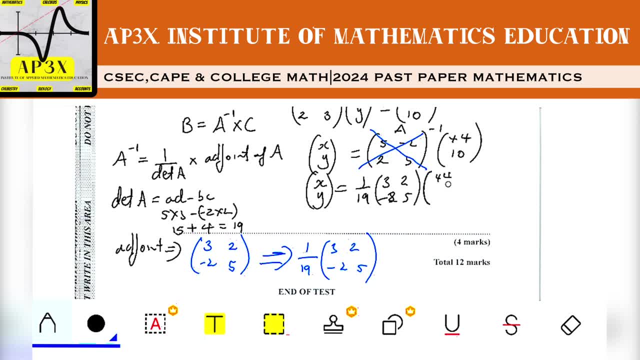 Five and we're going to times that then by 44 and 10. You can see it's four marks guys. So it's a lot of work. 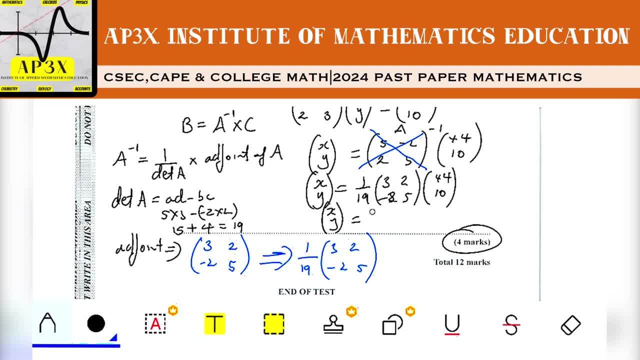 So now we're going to have XY, which is therefore then equal to one over 19 and we're going to then go row by column for this metric here. 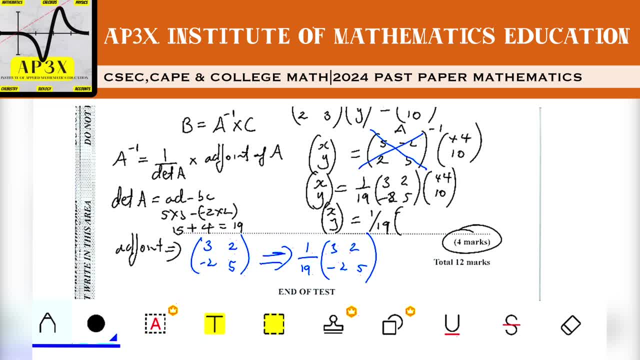 Now three times 44 that sounds like 132. So that's 44 times three. That's 132. 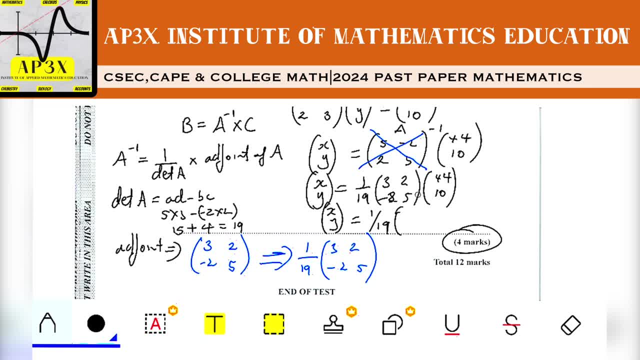 So when we go row by column and this is off the assumption that you guys already know how to multiply matrices. So row by column here we go three multiplied by 44 is in fact 132. 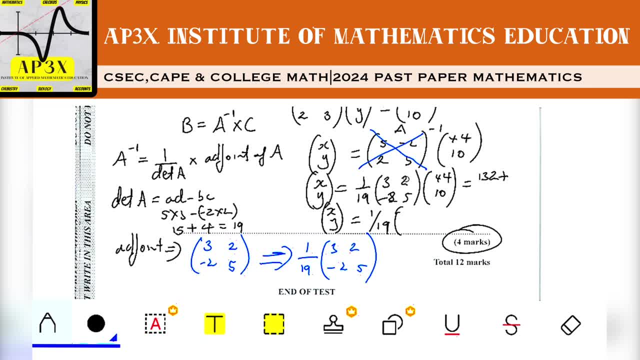 132 and we're going to add then two times 10 to 20. And then of course row by column again negative two times 44. 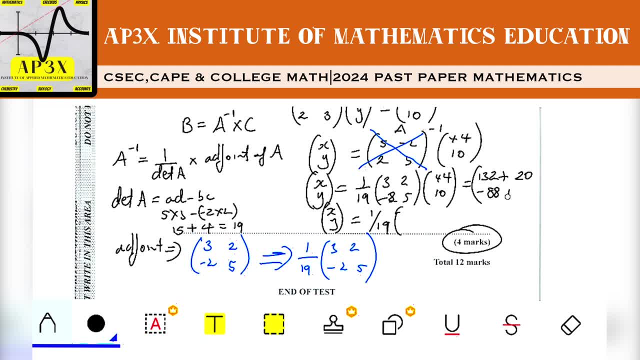 That's negative 88 multiplied by five times 10 is 50. 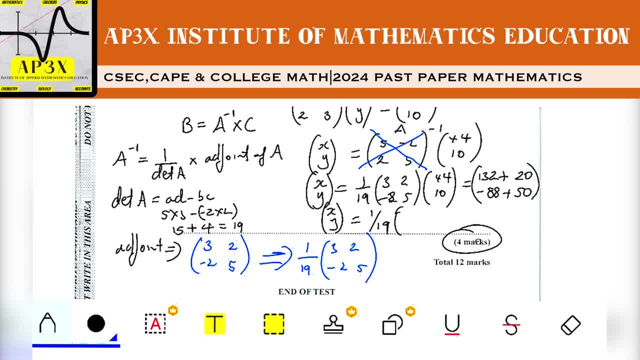 Now by doing all of that then 132 plus 20 that sounds like 152. So let me just go here and put my 44 10 here. So I know that when I do all of that, 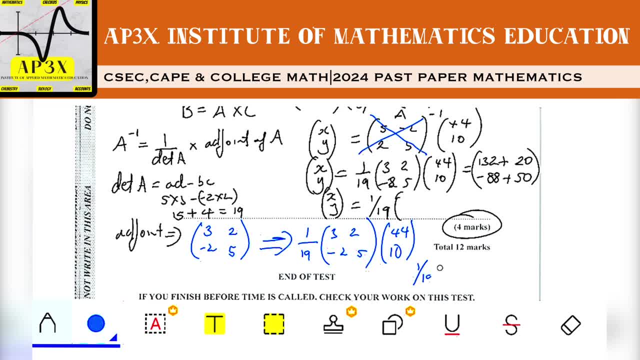 then I know that one over 19 will then multiply say here 32 132 plus 20. 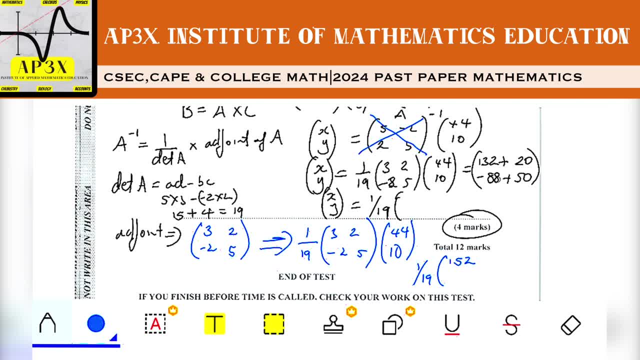 That's 152 and of course negative 88 plus 50 is going to be negative 38. 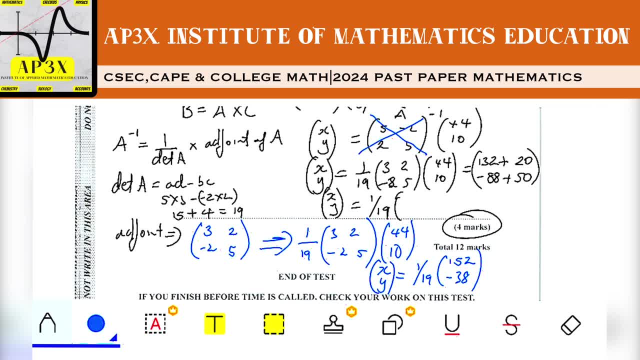 All right, and that's going to be that XY is equal to this. So by wrapping this up then we're looking at X being equal to 152. 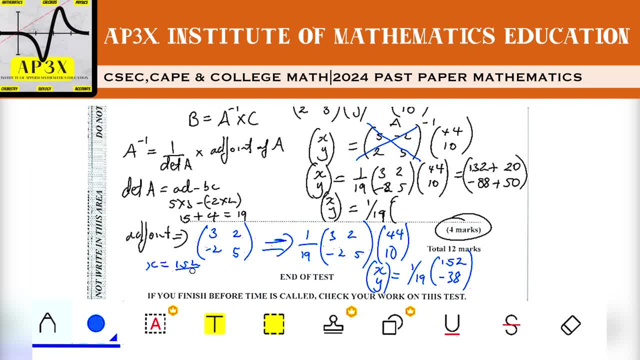 So X is going to be equal to 152 divided by 19. So that's 152 divided by 19 and that's eight. 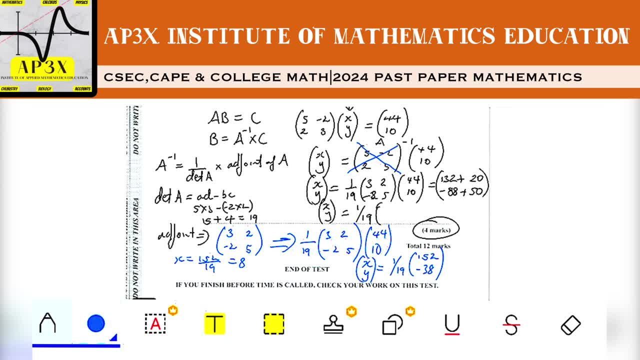 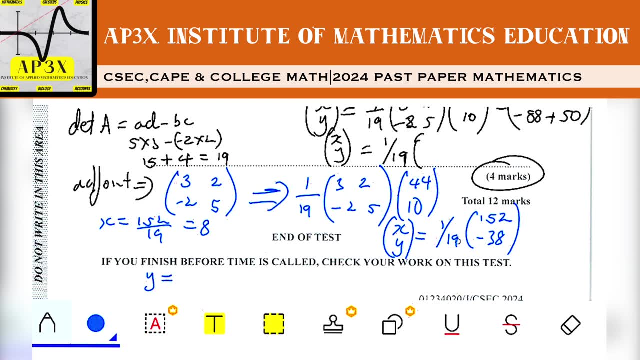 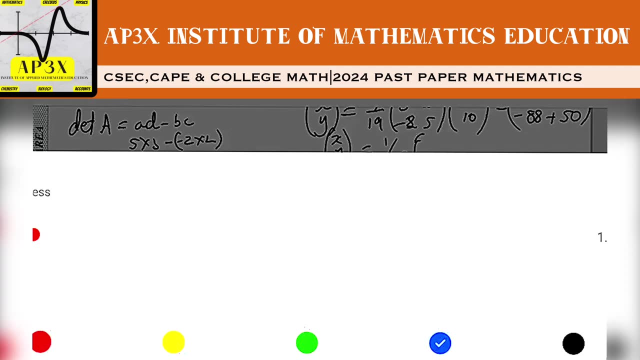 And then it works out that Y then is equal to running out of space here guys. So Y then is equal to negative 38 divided by 90 which is equal to negative two. So those are my two. 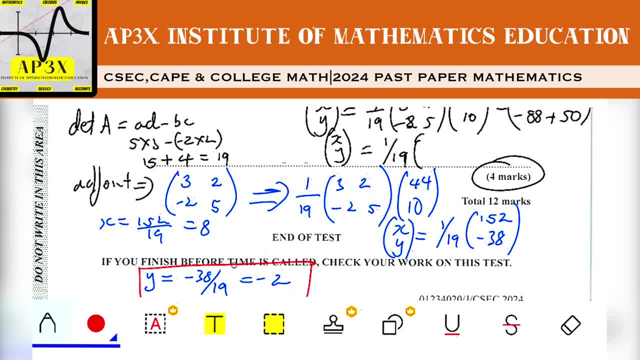 All right, now it was in fact a very lengthy video. 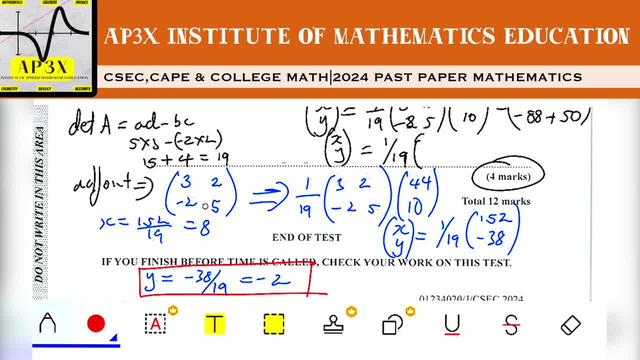 All right, I really try to take the time out to go through these process with you. I actually made this video for a specific group of students who are currently being prepared for the exam up on watching this video. 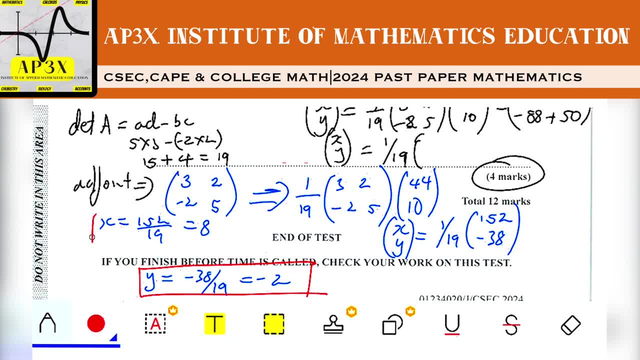 You may or may not have completed the topic of matrices. If you have already then most of what was explained here that been a little bit clearer to you. All right, so I hope I was able to help you in, you know, understanding the whole entire paper. My overall analysis of the whole 2024 people. It was really a nice paper. It really dibbles and doubles with a lot of different areas in math that you students should have already been exposed to from 10th grade. So it really dibbles and doubles with everything. 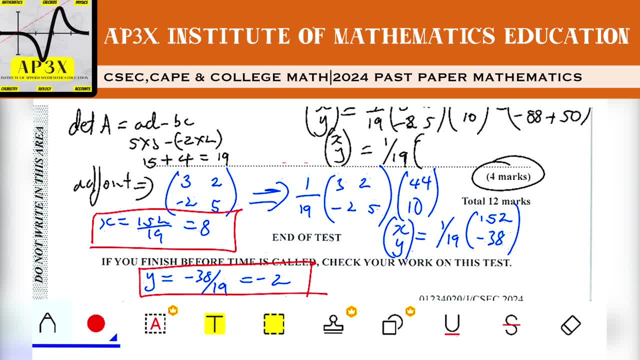 We saw a little bit of matrices. We saw a little bit of simultaneous equations and we saw a lot of simultaneous equation. We saw two very really, really interesting questions. 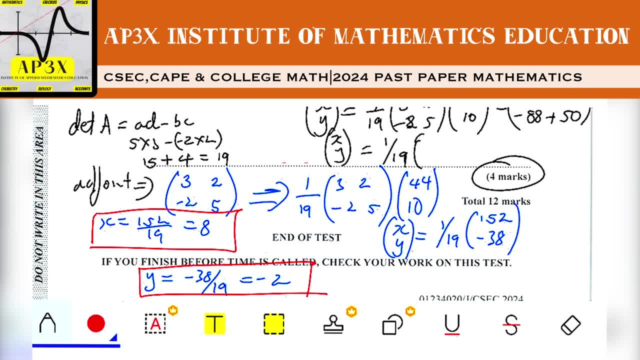 The circle theorem difficulty level was I would say some six or seven maybe at maximum eight. The functions was nice. The construction was very simple. 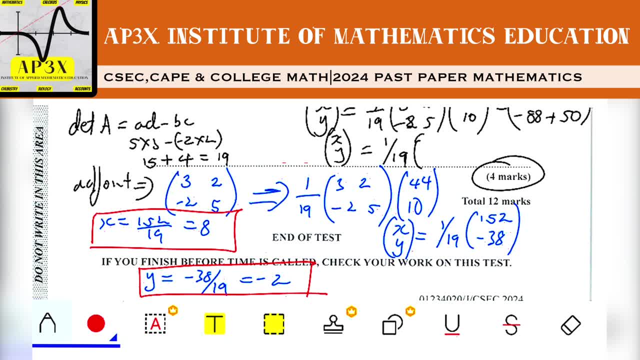 The worded problems in question one, two and three. They were okayed. 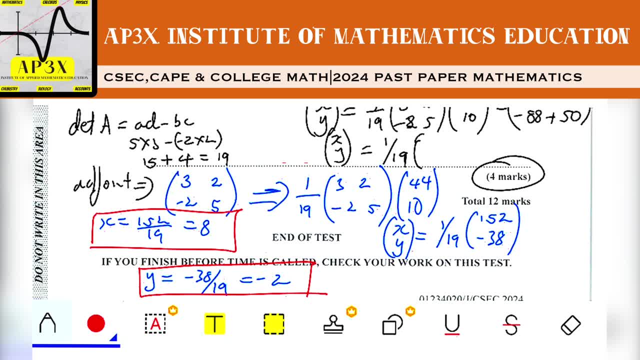 I really like the simultaneous question at the end of video number one. The statistics was also a little bit easier than usual. The pattern question was also very nice as well. 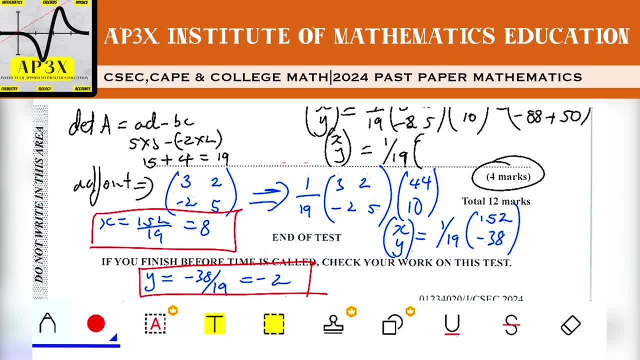 So overall in my estimation at first glance, the paper looked a little bit challenging but upon just going through the paper in details, it wasn't as bad as I thought it was. So I will give this an overall seven or eight in terms of being a really good paper. 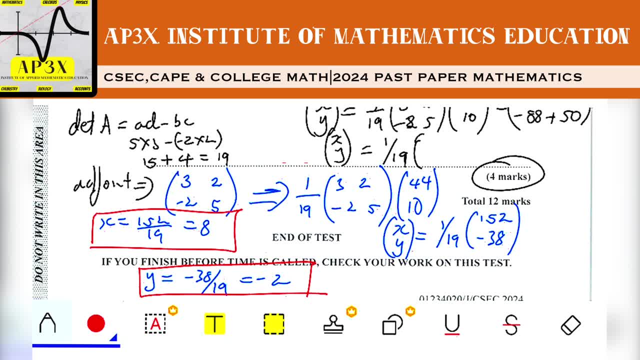 All right, not much challenge, but there were challenges. 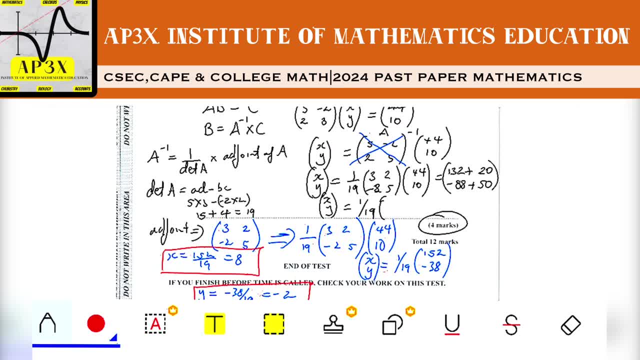 All right. So hopefully you guys enjoyed the video and you enjoy the series of breakdown forms for 2024 January paper.